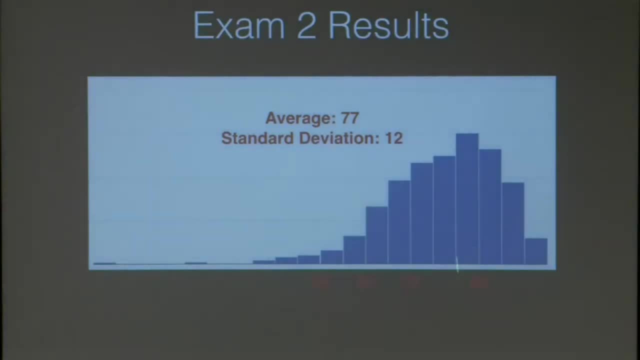 That's the A range, This is the B range, right. So the average was in the solid B range territory. And then, and so it goes, The standard deviation was 12.. Now I could tell you know, exam one. I. 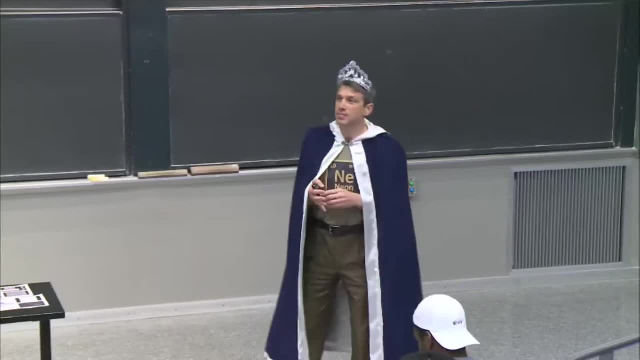 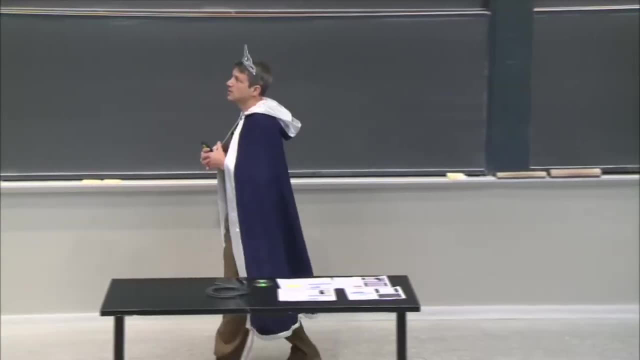 think a lot of the topics of exam one many of you had already seen and I think in this exam some of you had not seen some of these topics, especially like the crystallology of the holography, but also even the molecular orbitals, the band structure, And I could tell that you 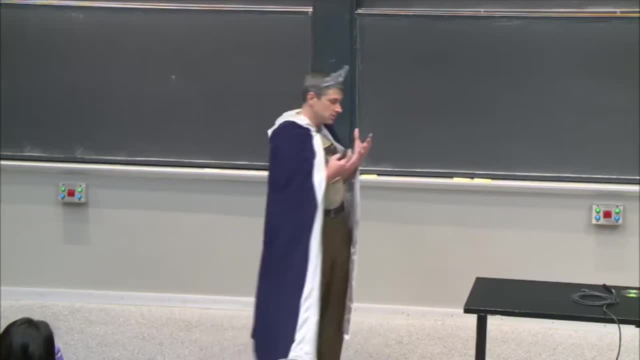 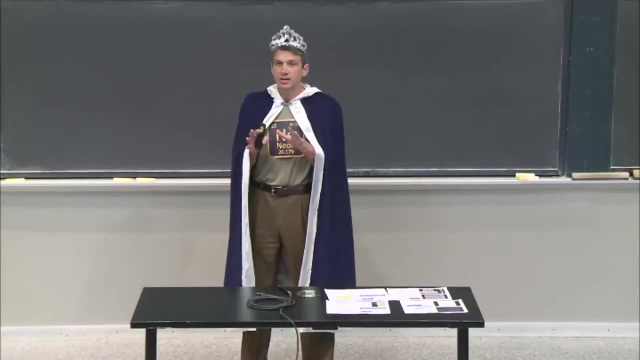 know. so some people were a little bit maybe, you know, had to work a little harder, maybe a little bit stressed, and I could sense some of that. But you know, when I get stressed what I do is I need. 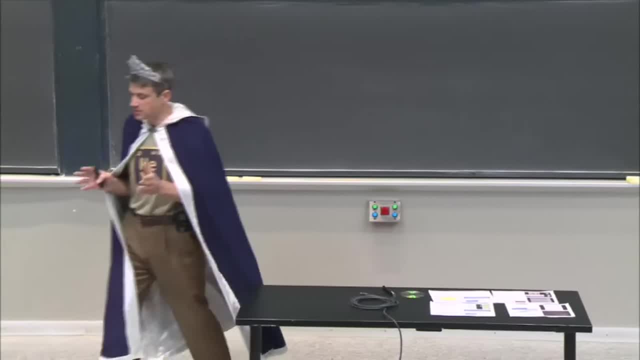 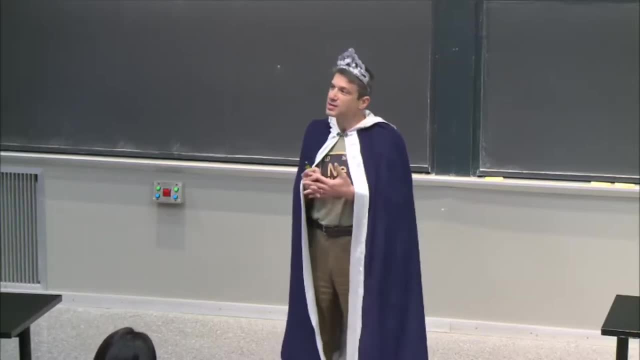 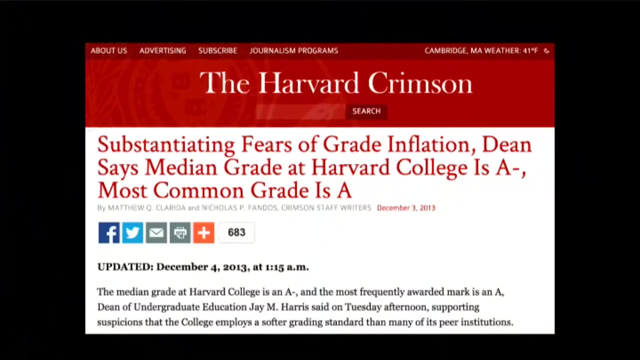 to kind of de-stress somehow, and sometimes, you know, some people listen to music, some people do other things. I always like comedy as a way of relaxing, And so what I do is I'll go to the Google, like for articles about Harvard, and I found, and so I found- this one. This is actually an 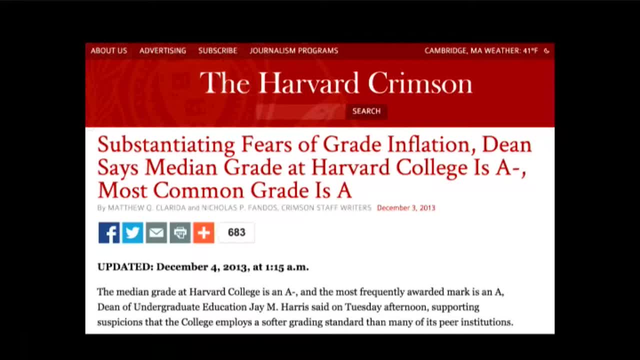 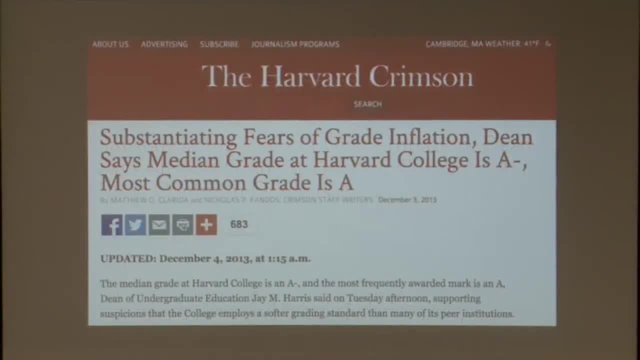 article in the Crimson and you know, and so some a few years ago, and the most common grade at Harvard is actually an A, an A, a solid A, the most common grade, And I like this. Okay, suspicion. 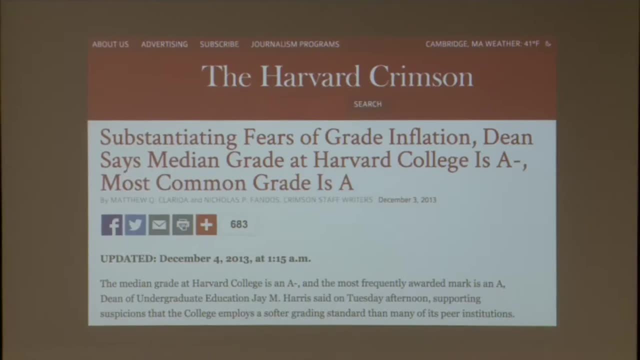 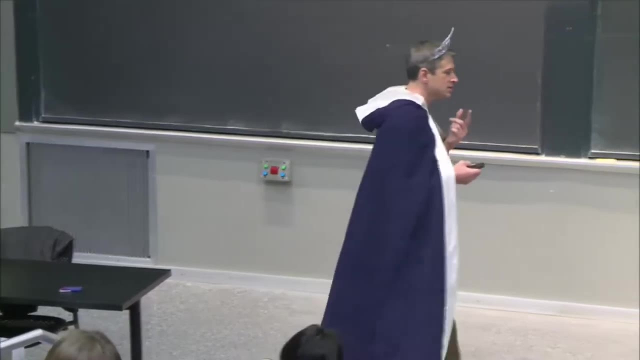 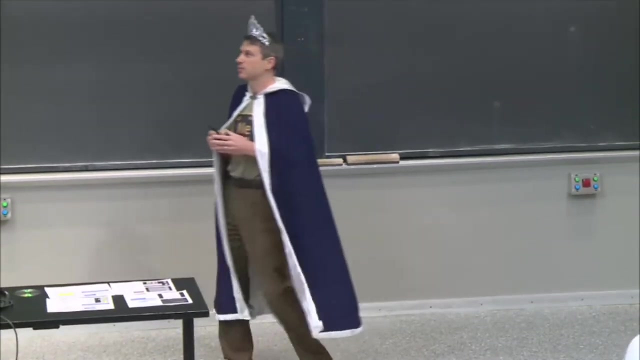 that the college employs a softer grading standard than many of its peer institutions. You think, If I mean, if everyone's getting an A. you think I mean, but the thing is so. what I wanted to point out is like there's a difference, right, And it's not just about: okay, you're privileged. 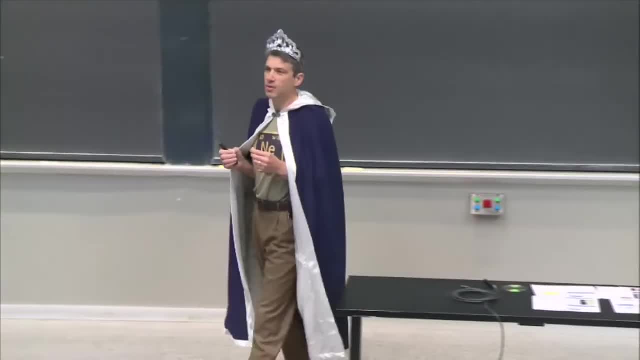 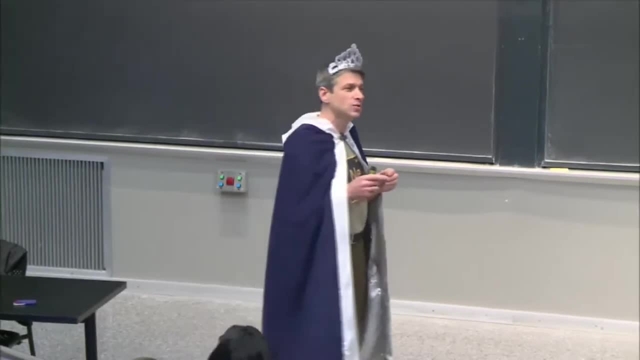 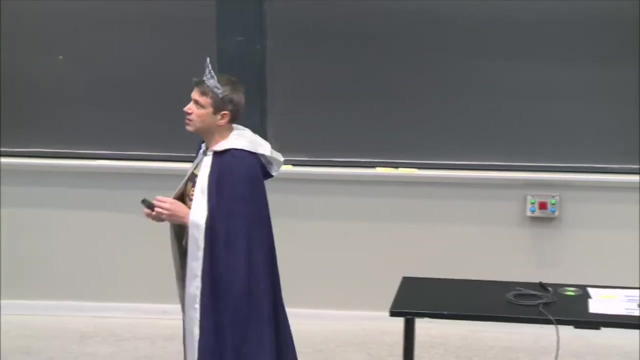 therefore, you deserve an A, whereas we know that that actually takes work. That's not the point I want to make. The point I want to make is that we know also what to do when we miss things. We know what to do when we don't get things right. right, That's when you do the work. 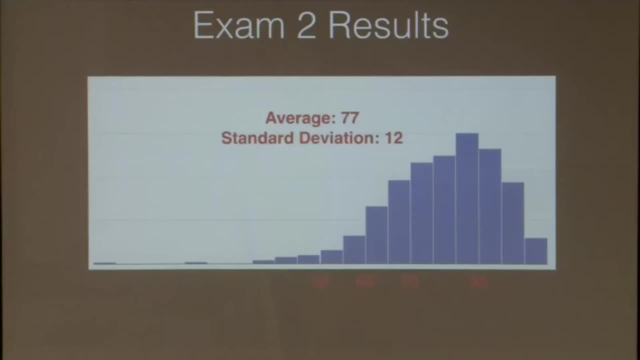 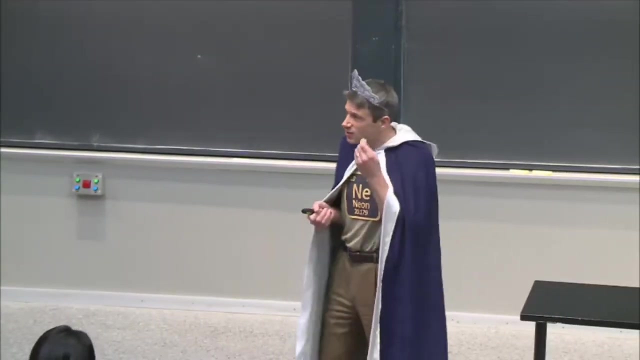 You know. so, wherever you are on this curve, go back and figure out what didn't work, What did you miss. Figure that out, because that's where you learn, right. I mean, there's a Thomas Edison who said: I never failed, I just did 10,000 experiments that didn't work. right, That you know, you got. 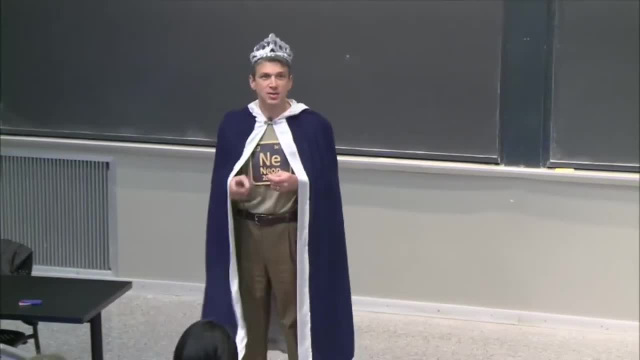 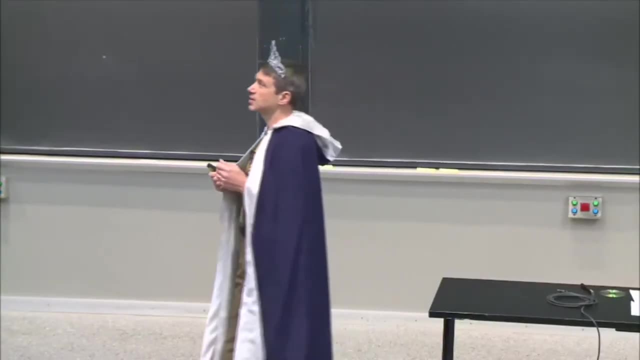 to get through that. You got to know that it takes hard work, and that's the thing that we know here. That's the difference, So please make sure you do that with exam two. We are all here to help you continue learning. I'm a noble guy. 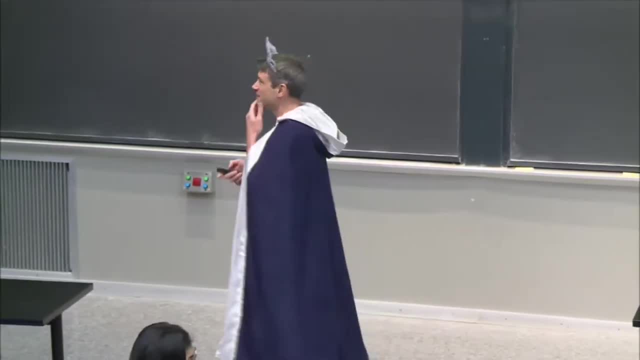 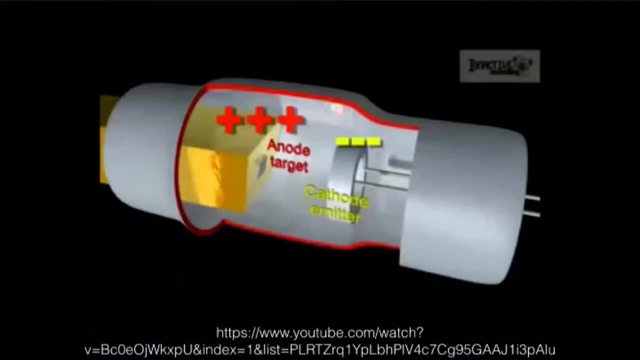 Yes, Anyway, Okay, And speaking of continuing to learn, right, where were we X-rays? So the last time now, on Friday, we had sort of you know some other things going on, but I also was trying. 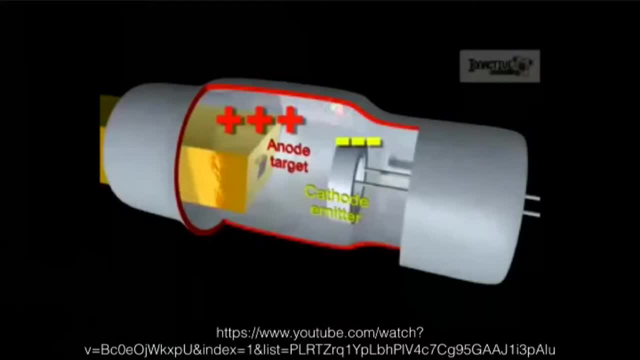 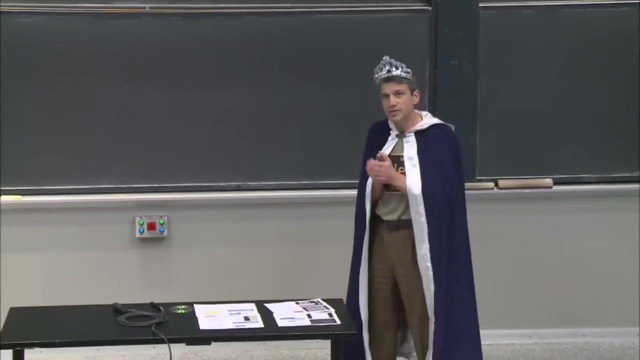 to teach you guys about X-rays and Gesundheit, And what we did is we learned how they're generated, right- Remember that The Roentgen experiments right- And so I want to pick up here with the kinds of X-rays that we have. There are two kinds of X-rays. 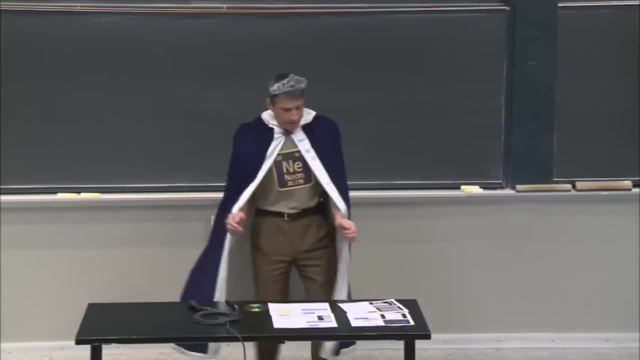 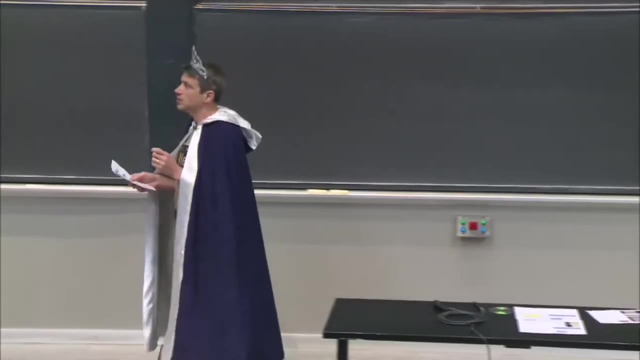 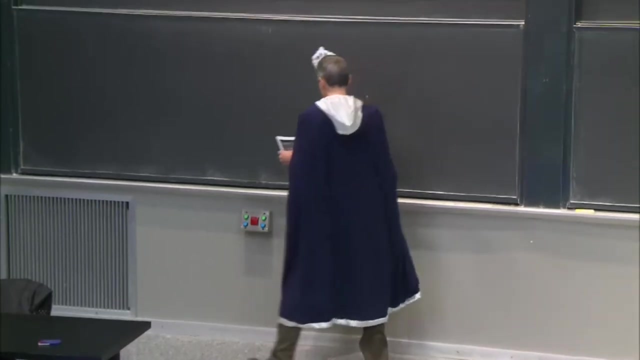 right, And we learned about those on Friday And I want to just remind you about those And I also want to show you a video to kind of recapture what they are. The first kind of X-ray- remember we plotted this as intensive X-ray, And so I want to pick up here with the kinds of X-rays that we have. There are two kinds of X-rays, right, And we learned about those on Friday And I want to just remind you about those on Friday And I want to show you a video to kind of recapture what they are. And I want to show you a video to kind of recapture what they are And I want to show you a video to. 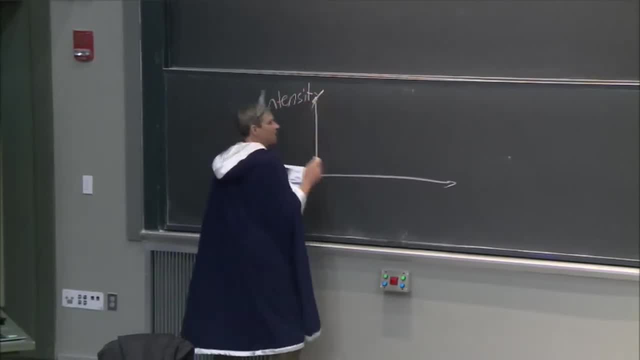 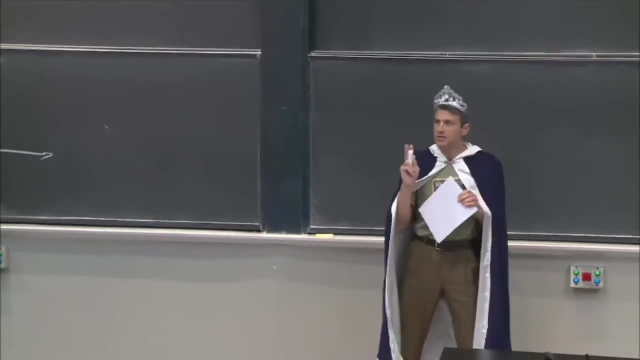 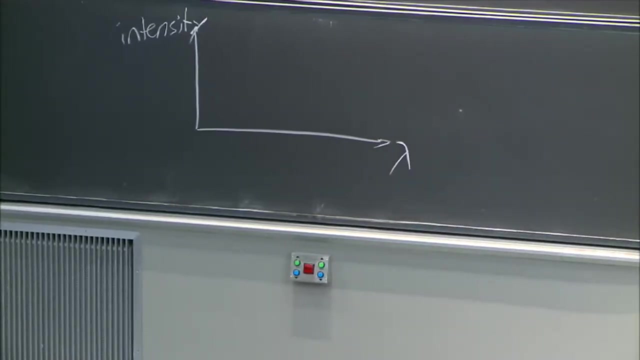 and I'm not going to draw the cathode ray tube again and the experiment that Roentgen did and all that. but I'm going to just jump to the two kinds of X-rays that you get right. And so if you plot the wavelength of the X-ray versus the intensity of the X-ray right, then one kind is the bremsstrahlung. 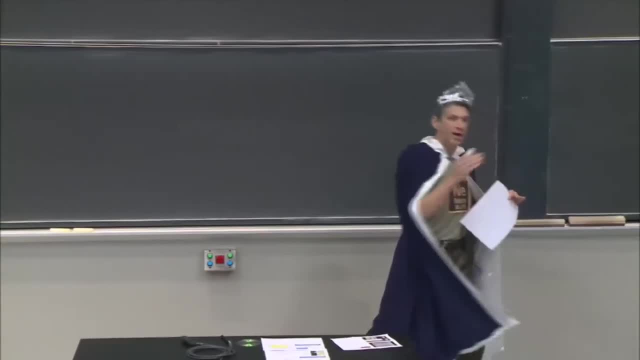 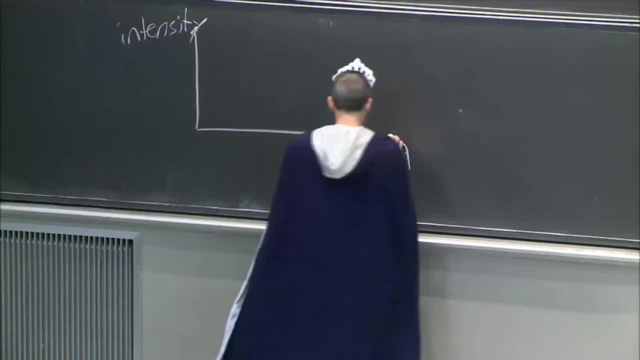 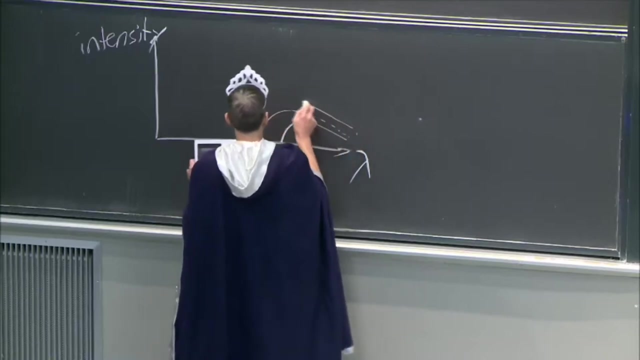 which comes from that electron getting slowed down, And if it slows down it emits radiation in a continuous spectrum, right, And so you might get. you know, remember, we sort of drew these: yeah, OK, And this might be, you know this. 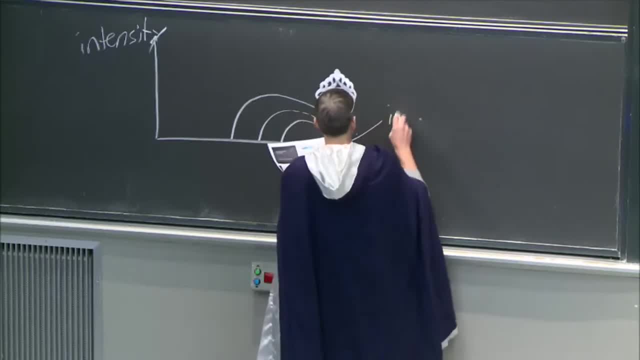 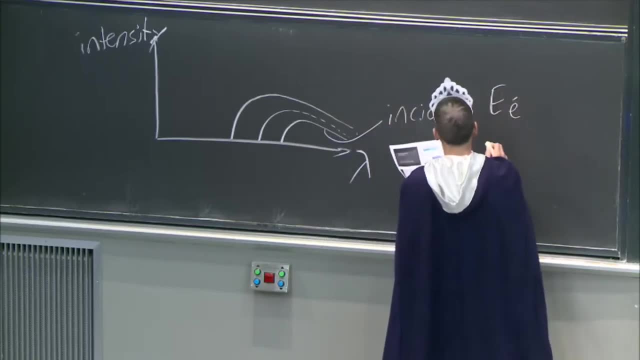 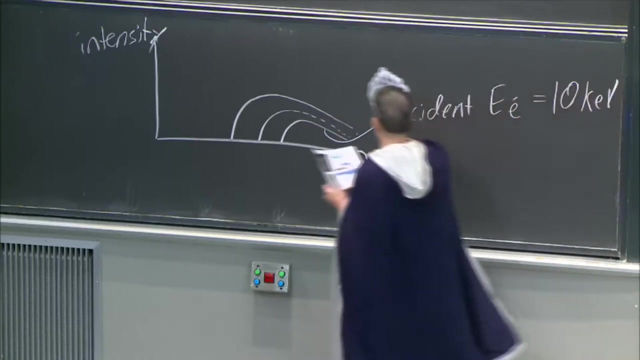 would be like the incident electron energy right Incident, let's say incident energy of the electron- OK, maybe like that's OK, I don't know, like 10 keV, 10 keV, And then up here the incident energy of the electron. 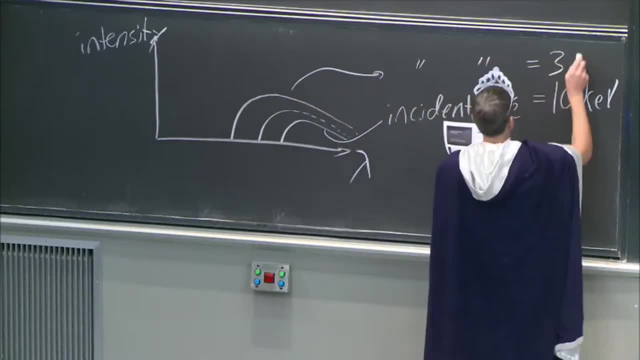 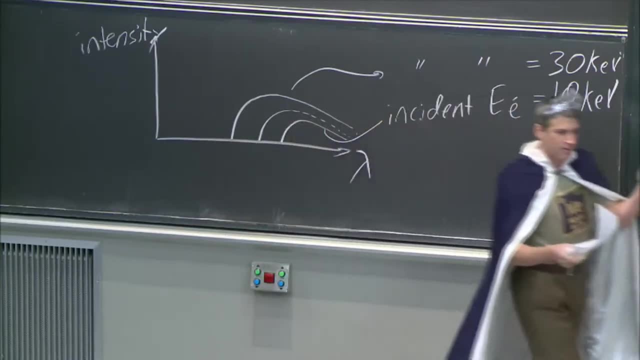 was, you know, something like maybe 30 keV, right. And so you see that as you hit that anode, remember what Rankine did: He took a cathode ray tube and he upped the voltage, So he really cranked up the voltage. 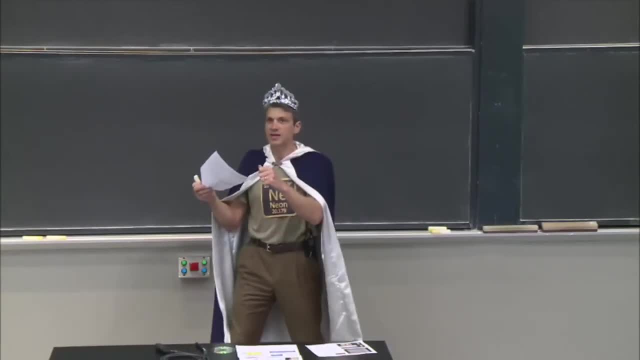 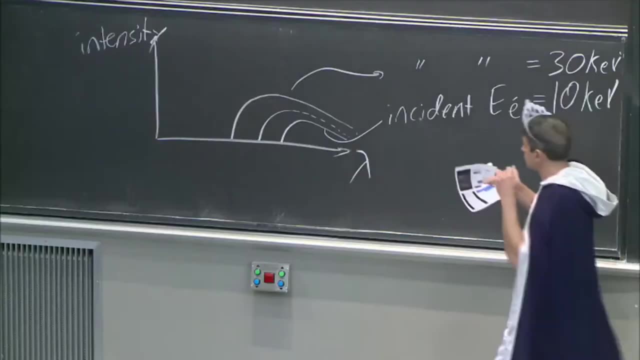 So those electrons coming off the cathode are going really fast, right? And then what he did is he put a piece of metal in their way And what happened is those really high energy electrons. they see those metal atoms and sometimes they get inside the electron cloud and they turn. 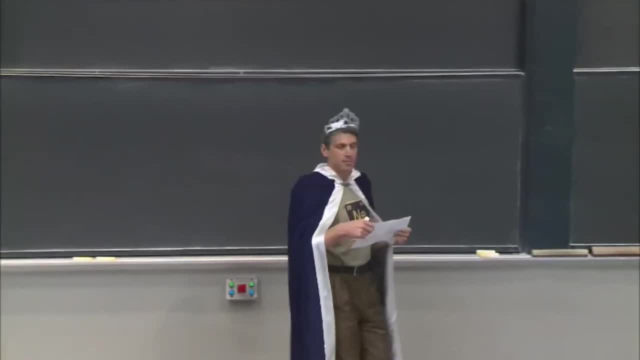 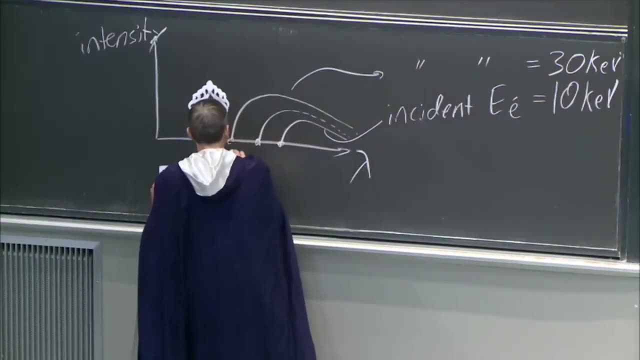 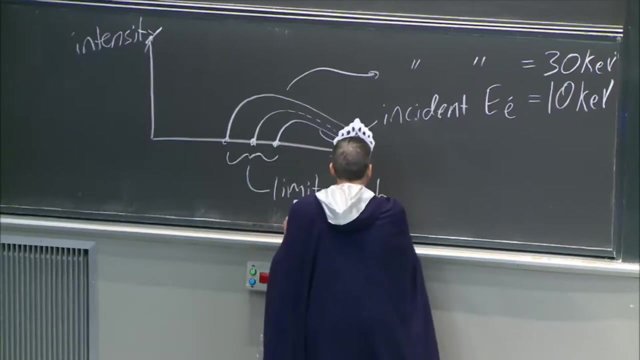 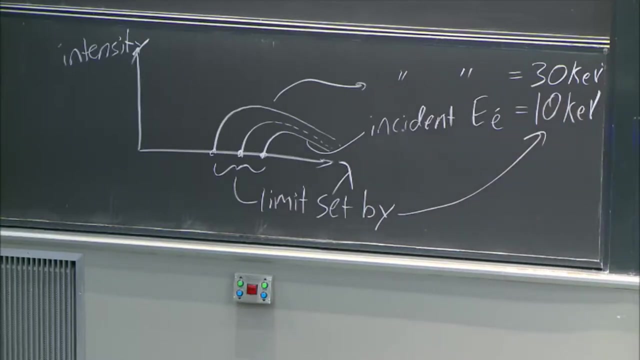 And that's when they give off this continuous radiation. But we also know that there's a limit here, right? Remember that We talked about that And that this limit is set by this: The maximum amount of energy that you could get out. 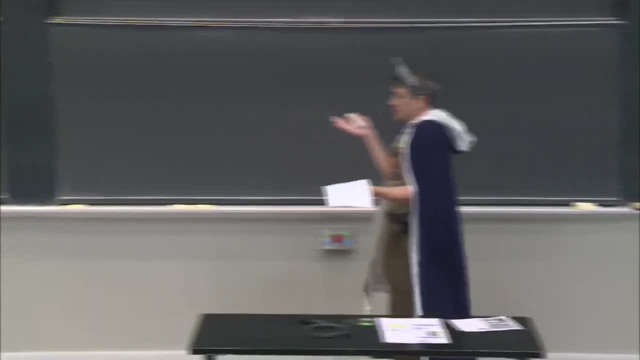 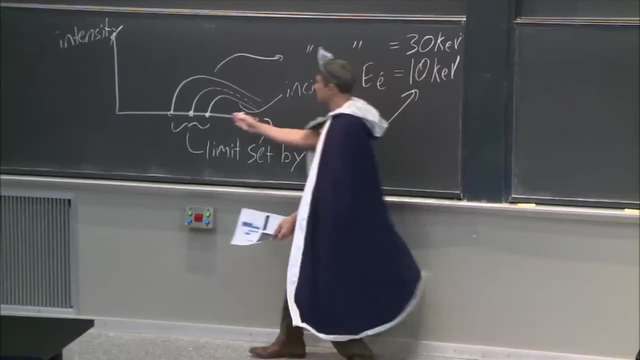 of a photon being emitted this way would be equal to the incoming electron. The incoming electron transferred all of its energy to the photon, So that's why there's a maximum And it's also why it increases. Remember: shorter wavelength, higher energy. 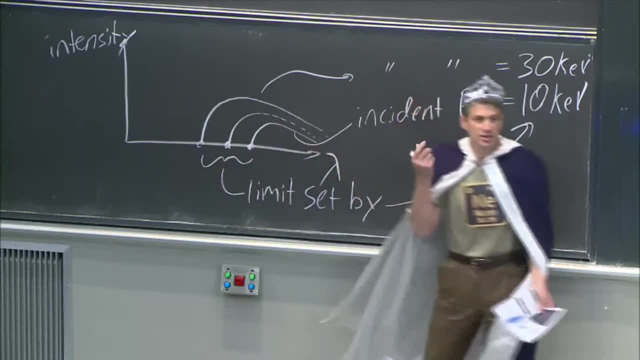 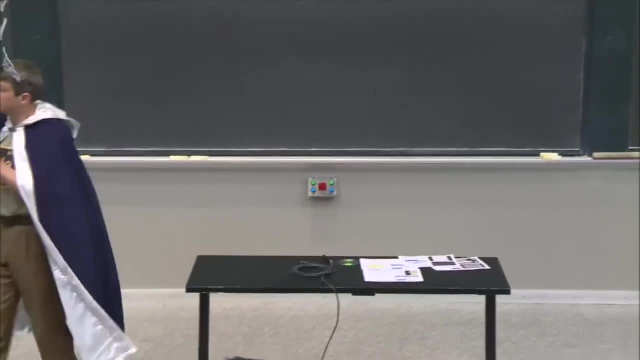 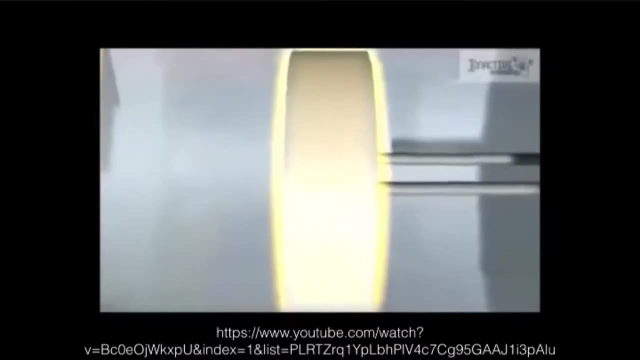 So it increases as you increase the energy of the incident: electron- OK, That is Bremsstrahlung. Let's watch a video, because this is actually a very nicely done video that captures it with animation. So here's your CRT Now, OK, here they come. 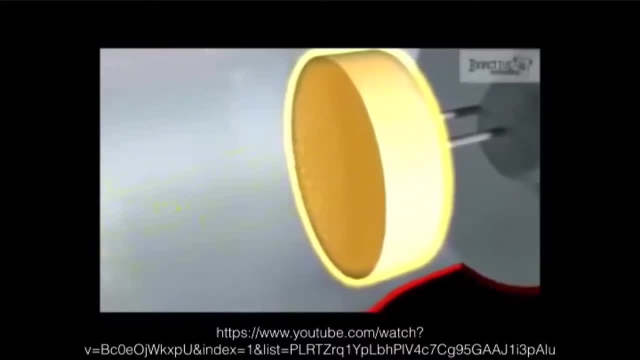 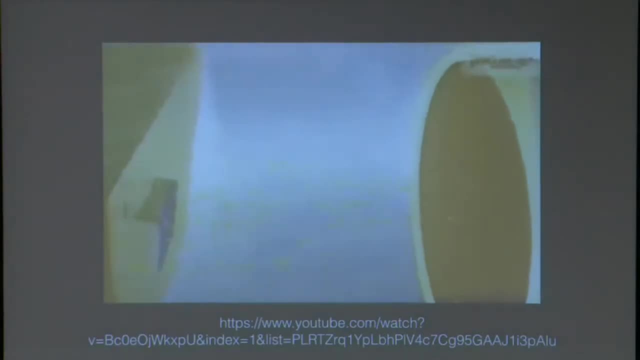 Those are those electrons and their voltage is high. So they're coming out. Look at them coming out really fast, right? Lots of kinetic energy, OK. And then there they go And they put, and this is what Rankin did. 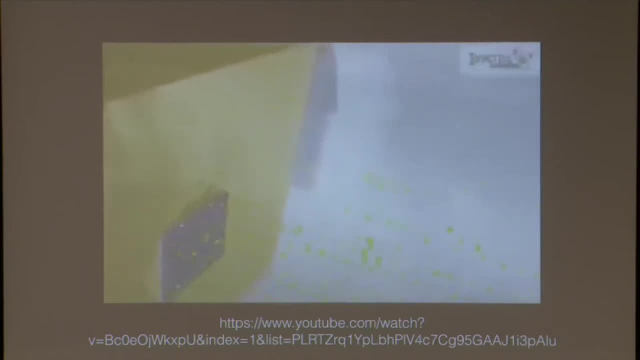 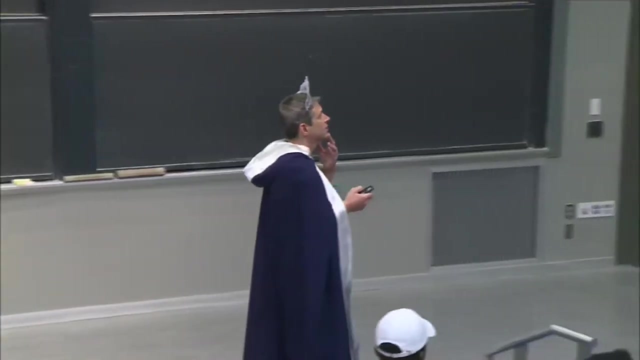 He put a little piece of metal in there. So now those electrons are hitting the metal. OK, So those are the two things that he differently remember. the room lit up even when all the lights were off. OK, there they are. 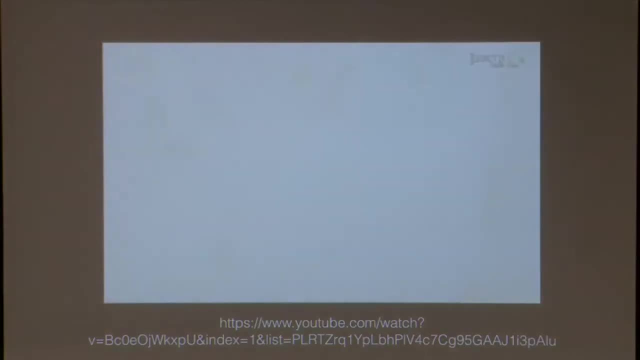 Nice Good electrons. Oh, and here they go, And there's the metal atom. OK, And oh, look at that. Now, what are these? Those are X-rays coming off. Those are the electrons hitting the metal. And here's the metal atom. 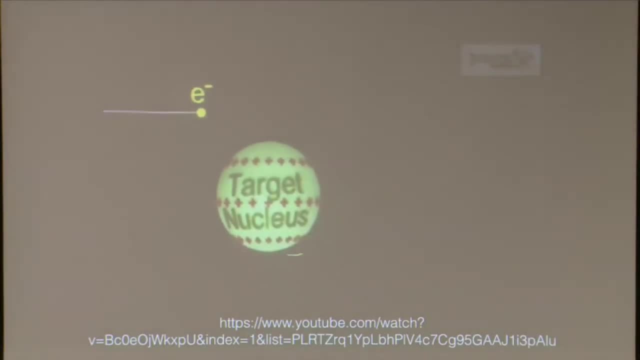 And as the electron comes in, remember it's not going to go, Remember it sees the charge of the nucleus And it gets deflected And that deflection loses energy And that loss of energy goes into a photon Now, because these electrons have such high energy. 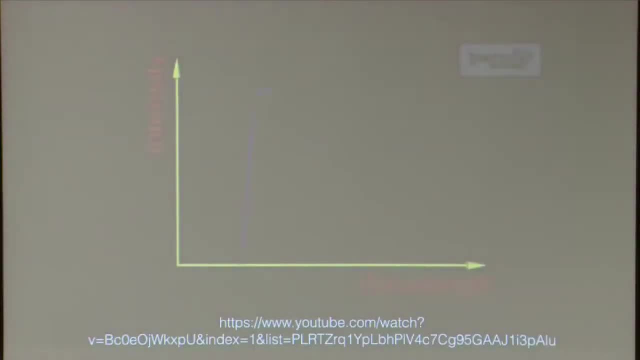 to start with, because they have such high energy to start with. the energies of the photons are very high. They're X-rays, right, They're X-rays And so OK, and so here's the wavelength, And you can see that. 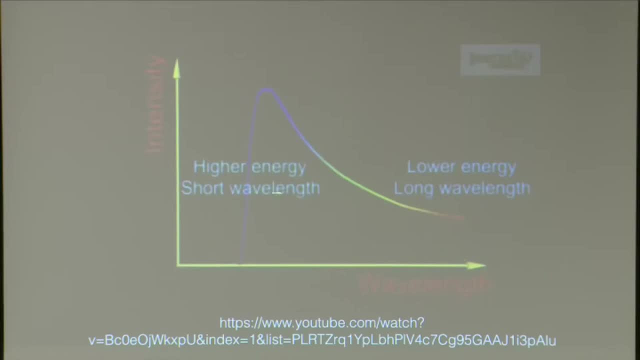 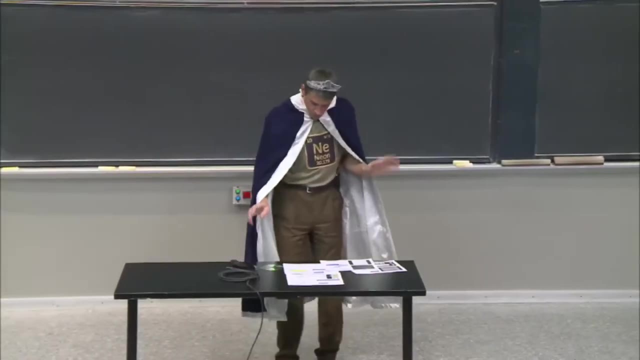 Well, it's sort of a little hard to see in this blue range, But see: higher energy, shorter wavelength, Lower energy, longer wavelength, Very nice, OK, so that's the animation of bremsstrahlung Now, OK, good. 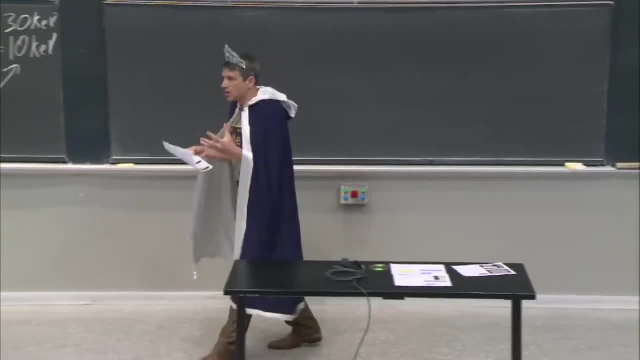 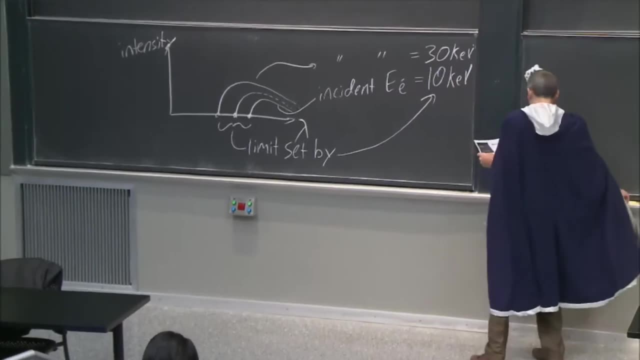 Now the thing is, what we also learned is that there's another type of X-ray, There's another type of X-ray And in fact, if you crank this up high enough, you can get that other type. So now we go higher. 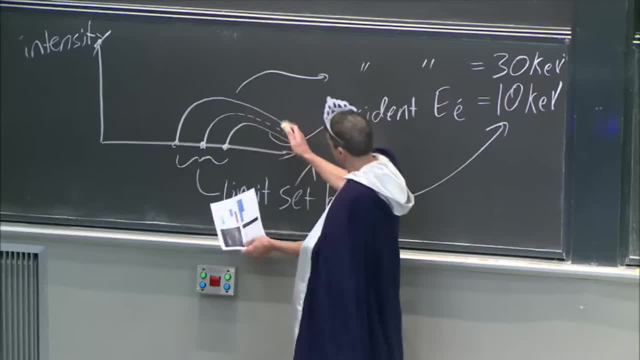 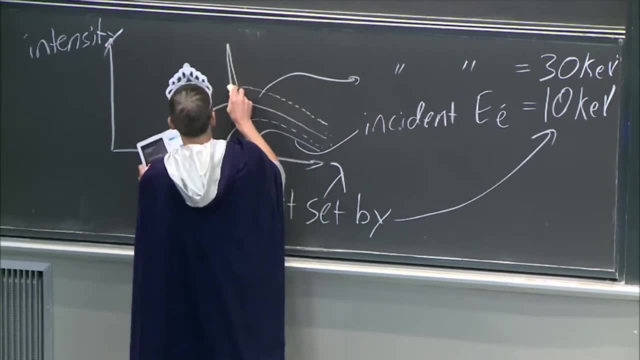 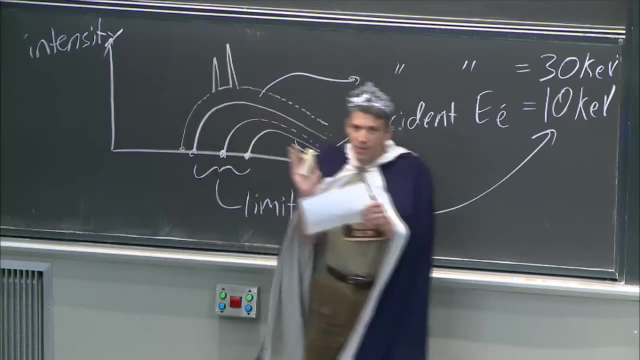 Oh, we didn't see it here. It just looks like that And that and that, And then all of a sudden we go up to 40 keV And we see this. Why What happened here And what happened here is a totally different mechanism. 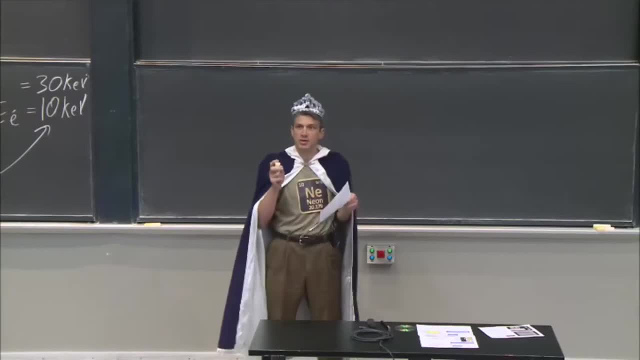 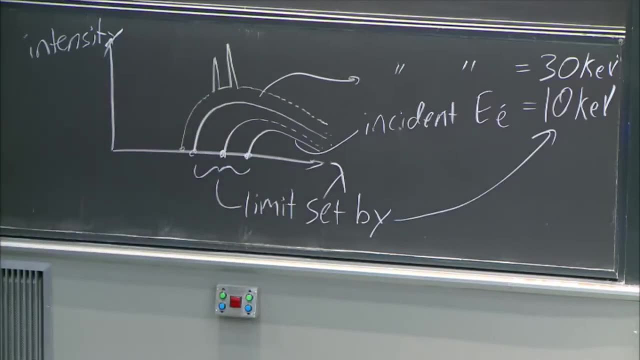 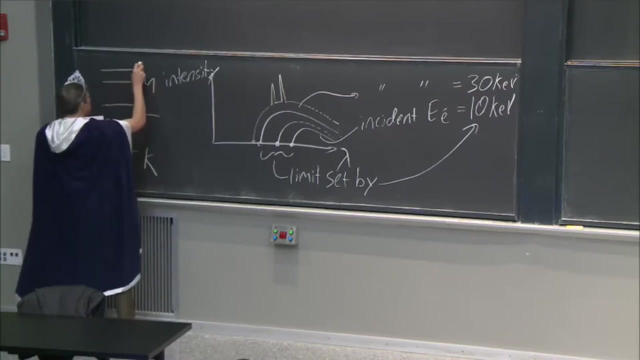 for generating X-rays, And that was the second type that we talked about on Friday. Those peaks are called characteristic And the reason is that, remember, we have these levels which, now that we are talking about X-rays, we give them letters: K, L, M, N. 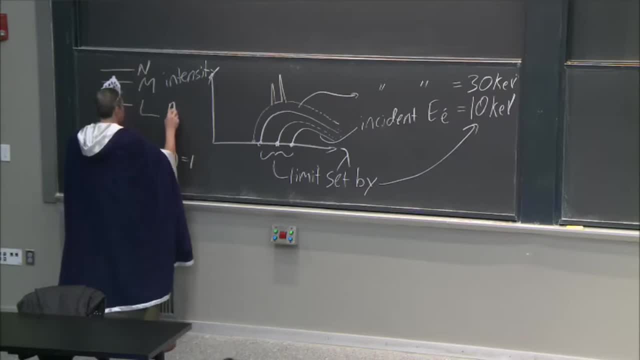 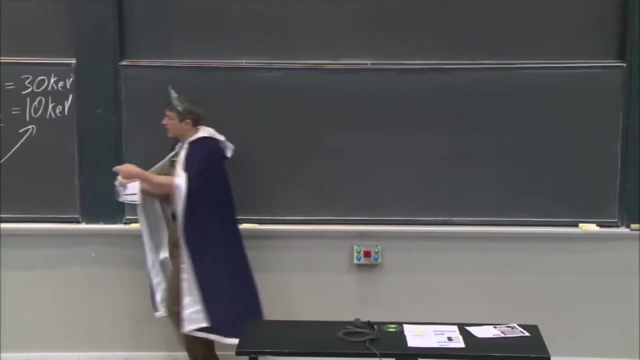 But it's just the quantum numbers: N equals 1, N equals 2, N equals 3, N equals 4.. And what we said is that the way characteristic X-rays are labeled is that if an electron is excited from this, gesundheit. 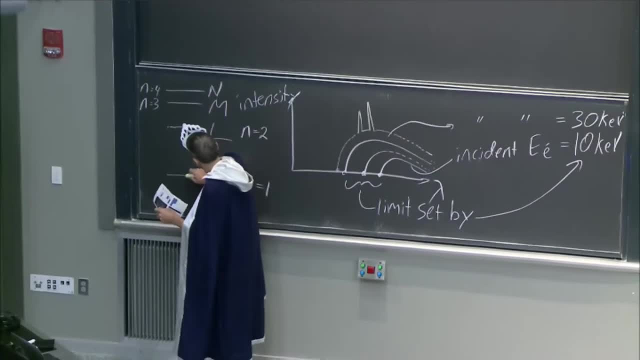 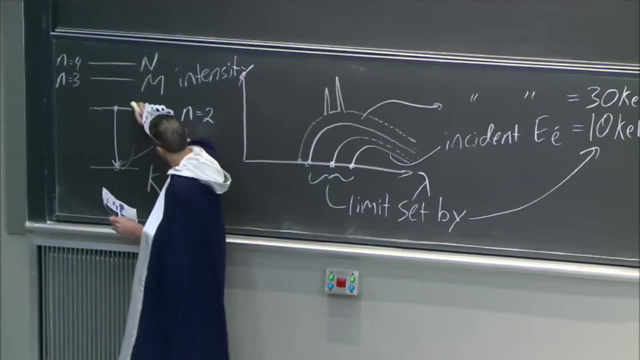 from this lower level. if an electron, if an electron is knocked out of here, then there's a place for an electron from here to go down. Maybe the electron is excited, Maybe the electron is kicked out And then something here can come down. 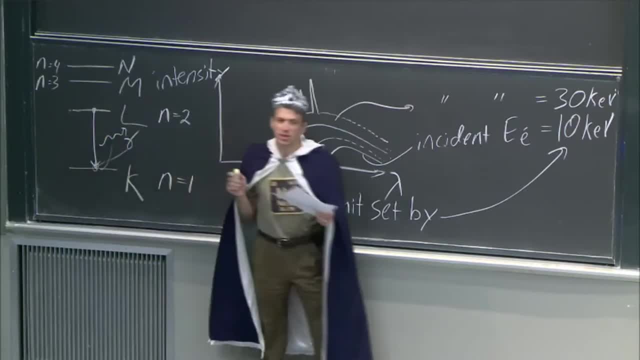 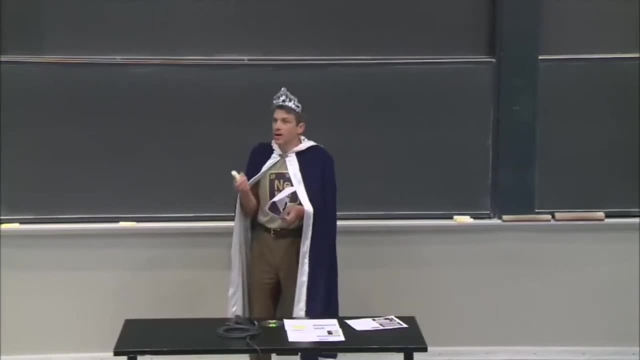 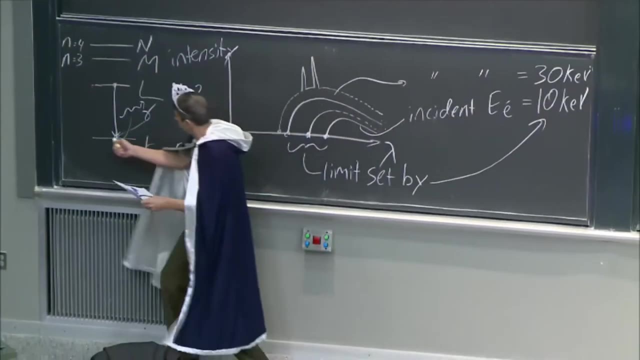 And when that happens, just like in the Bohr model, you get radiation. But now, unlike hydrogen, 13.6 electrons, these are KeV of energy. These are very high energy. Why? Because it's the 1s electron. 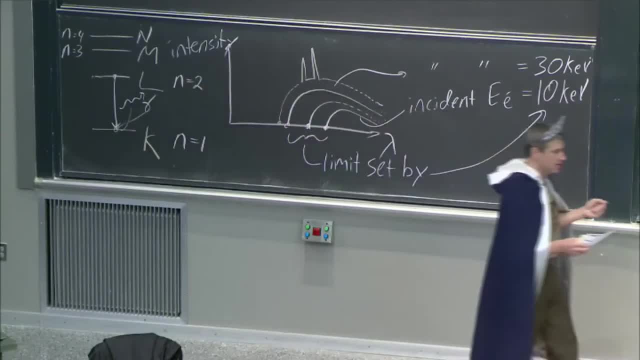 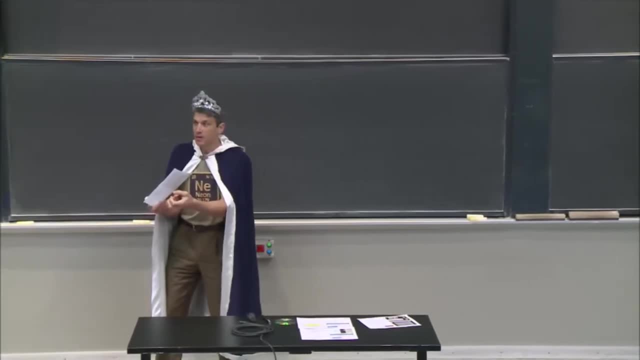 And we know that once you get down to those metals, those 1s electrons, you go further down the periodic table. those 1s electrons are seriously tightly bound And those levels have a difference down there. that is pretty high in energy. 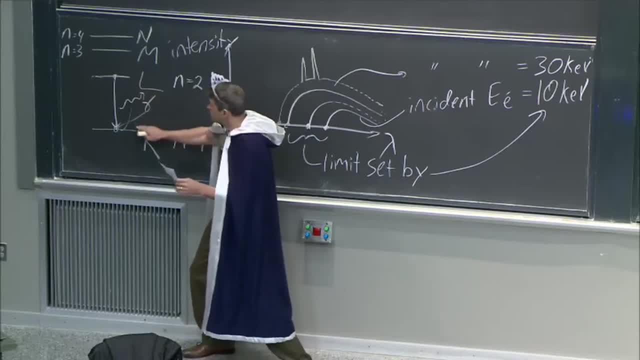 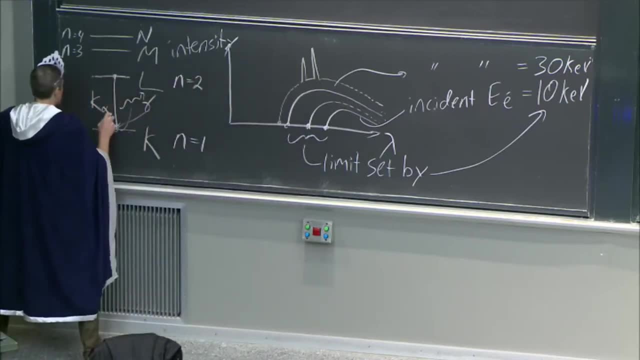 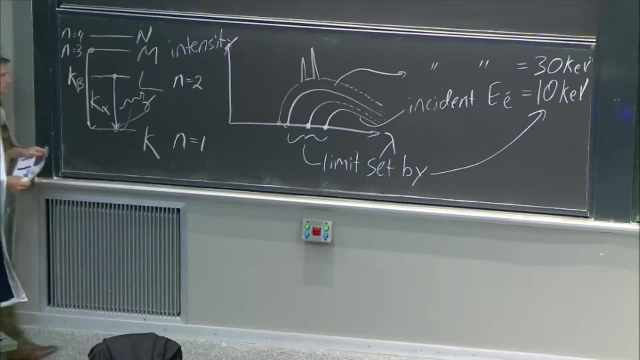 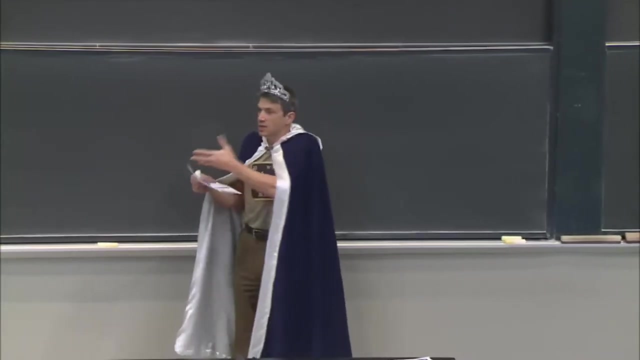 It's X-ray high in energy. That's the point. So now, when that cascade happens, we call that a K alpha, And if it were to have come from here, it would be called a K beta. right, And those are transitions that unlike this continuous energy. 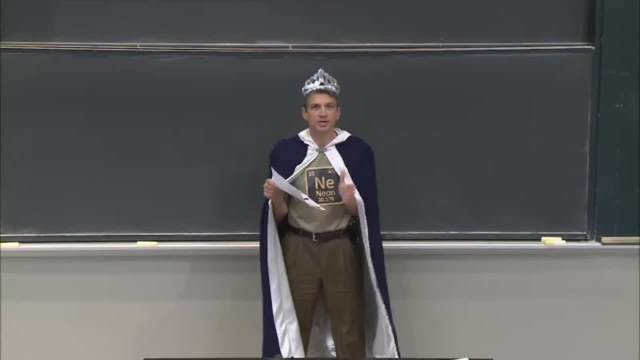 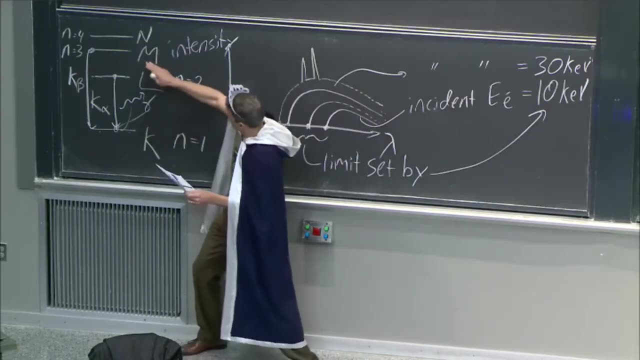 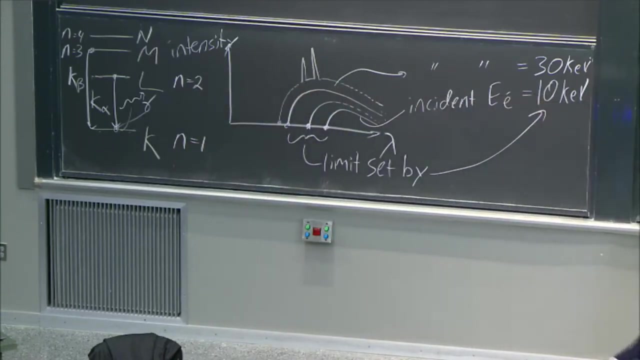 those transitions only happen at very specific energies: delta energies, right, The change in energy from L to K. or for K beta, it would be going from M to K. It's K alpha, K beta, It's the K, because that's the final place the electron goes. 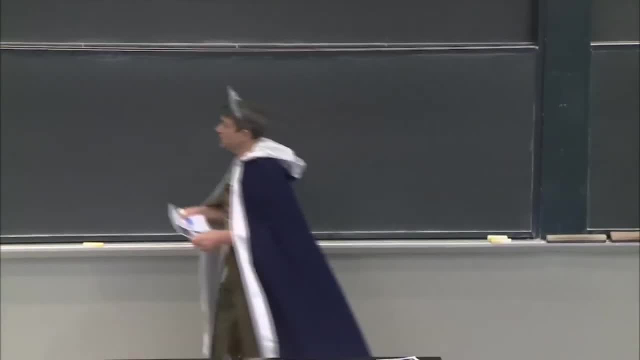 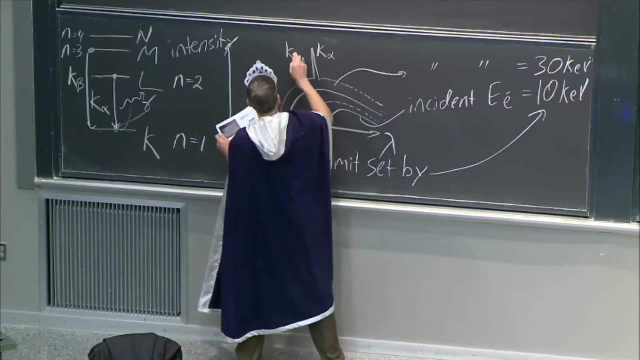 when it decays down. OK, So if you had to, if I just showed you these, I'd say: well, that would be like K alpha And that would be like K beta, because you know that K beta is going to be a higher energy photon, right. 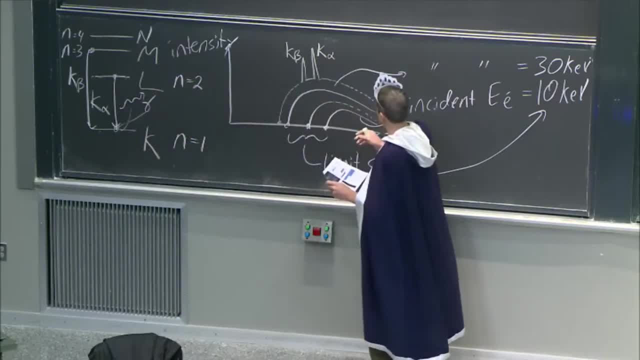 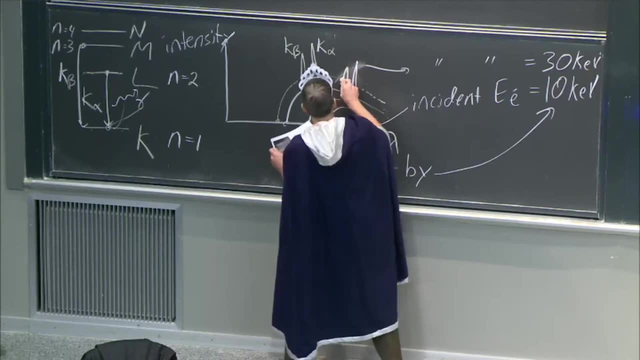 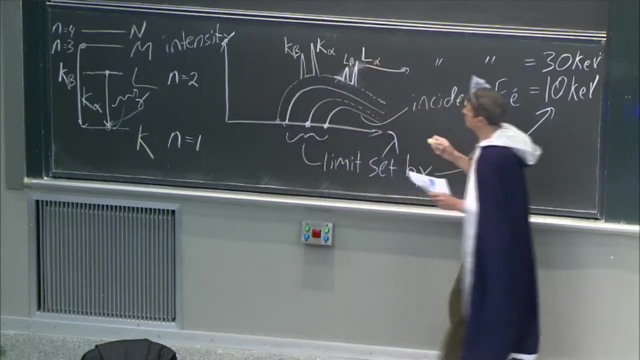 Because it came up from a higher level. OK, Well, you would also have on here some other peaks, right? You would have the L peaks right, So you'd have like L alpha, L beta, right? So as you crank the energy up, right. 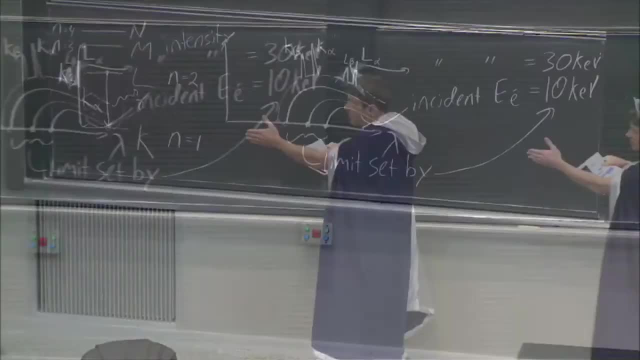 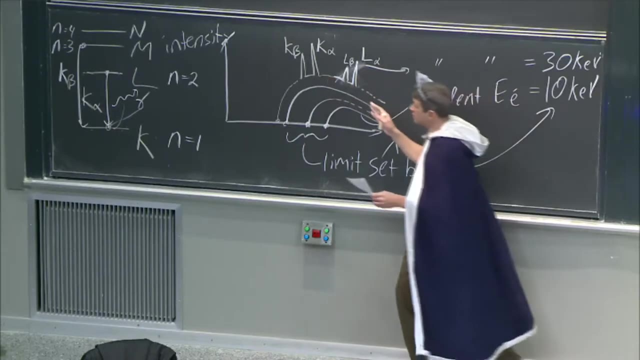 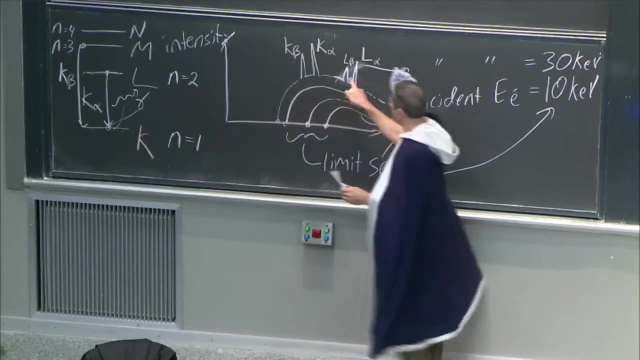 then you can knock out those core electrons And these cascades happen And you get these discrete peaks. Notice they will only come when you have enough energy in that incident electron, to knock this electron out from the core. So that's why they don't appear. 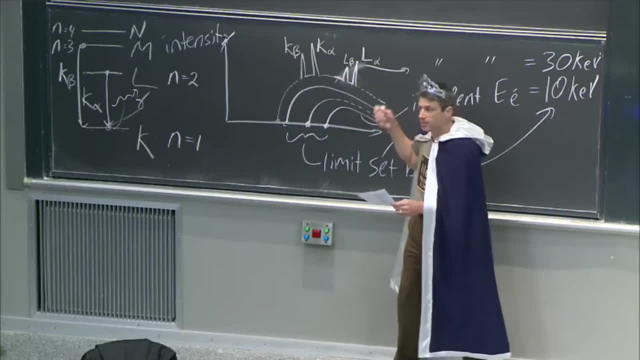 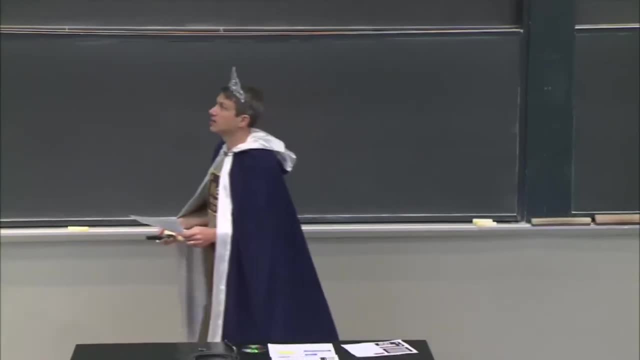 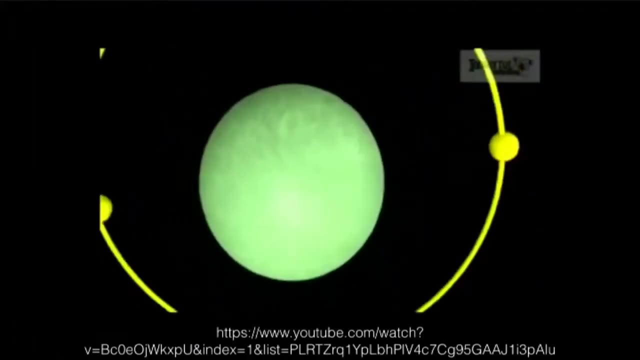 They don't appear until you get to a certain incident- electron energy, right. They don't appear until you get to that certain energy, right. And so we have a video on that, which also I will narrate. What. What Is this? it? 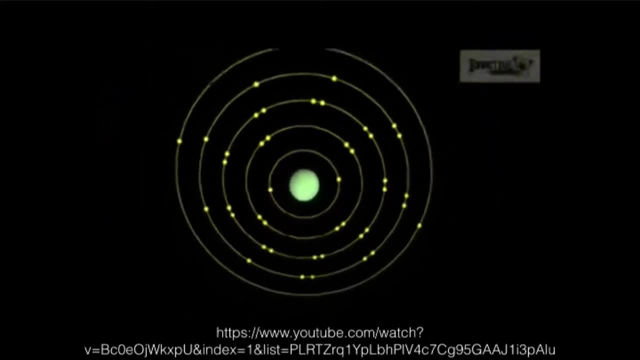 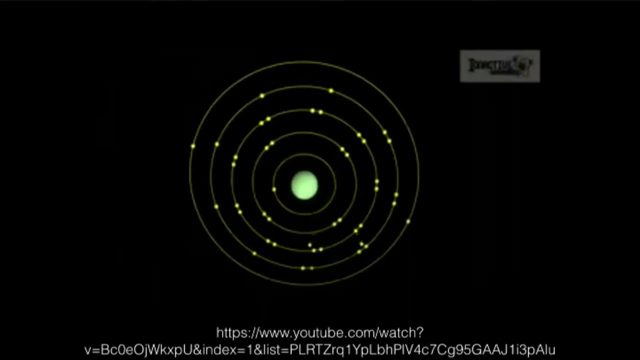 There we go, OK. So there it is. It's a metal atom, I don't know which one And what. you're OK. there's the incident: electron. You fired it And look at that: It knocked out a core 1s electron. 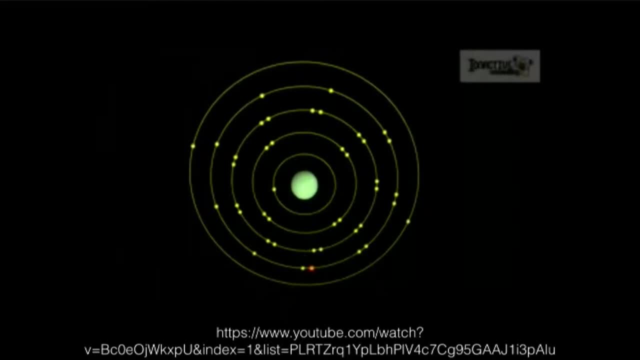 energy, very high energy. That's what Rankine did. Crank up the voltage higher, kV And there it is, A cascade down and an x-ray comes out. You see that? OK, So that very. is that all of them? 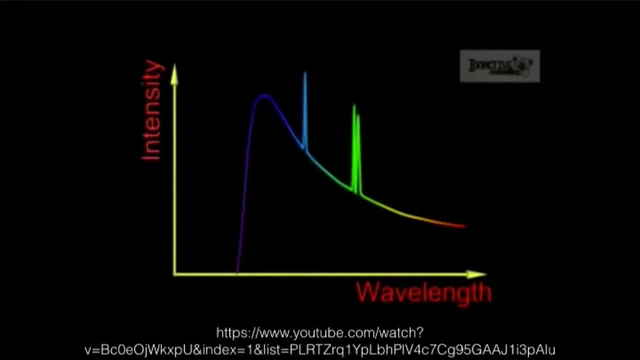 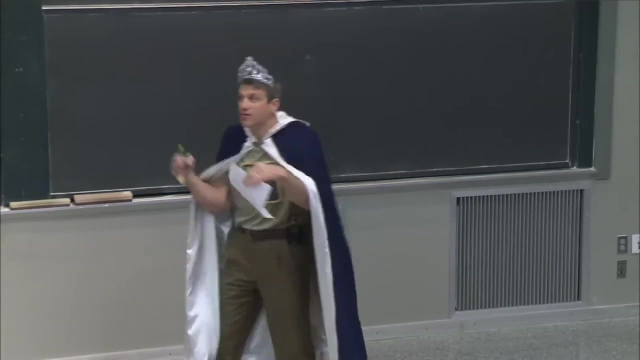 Oh yeah, And then it's going to draw. Because of those, you get these characteristic peaks. Now we call them characteristic because now you can see why. So, unlike the continuous radiation right, these peaks depend on the atom, Because they depend on the energy levels of the atom. 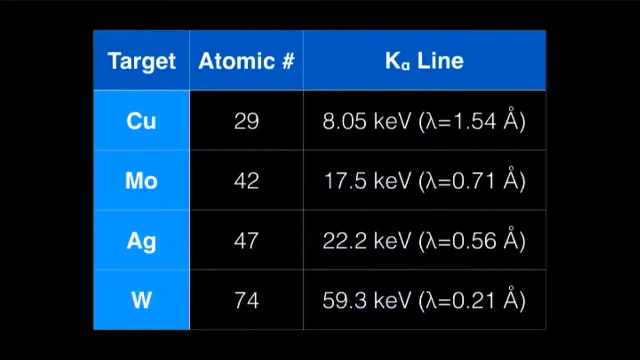 Right. And so that's why, like, if you look this up, you say, well, OK, let's look at the k-alpha radiation, Let's look at the k-alpha peaks, right, that come out of different atoms. They're going to be different. 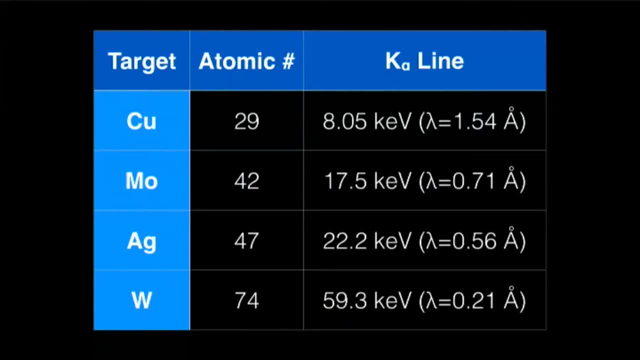 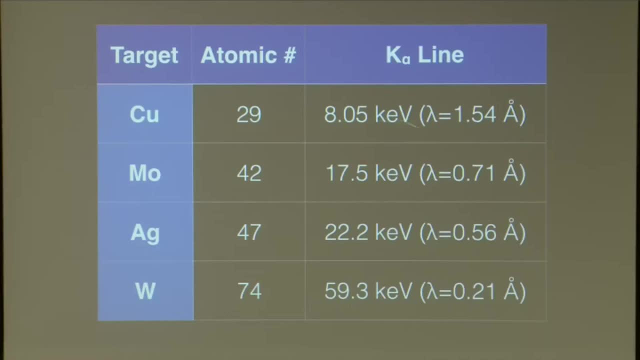 OK, So you have very sharp lines of x-rays and very specific energies. For copper it's 8kV, For molybdenum it's 17.5, right Silver, For tungsten it changes. 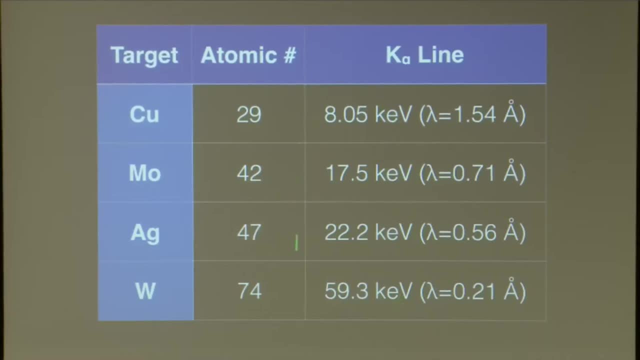 And you can see that it goes up right as that 1s electron is lower and lower in energy because I'm adding all these protons. So it all makes sense from the concepts we've learned. Oh, but see, now that's really useful. 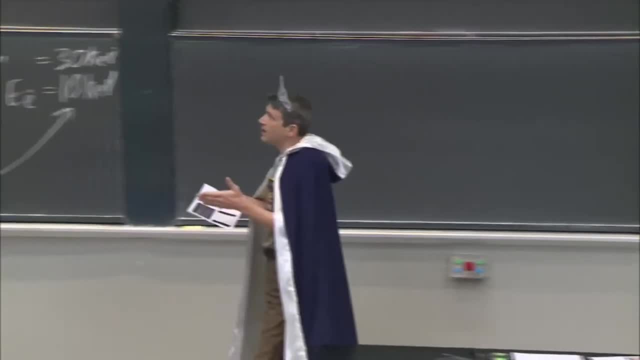 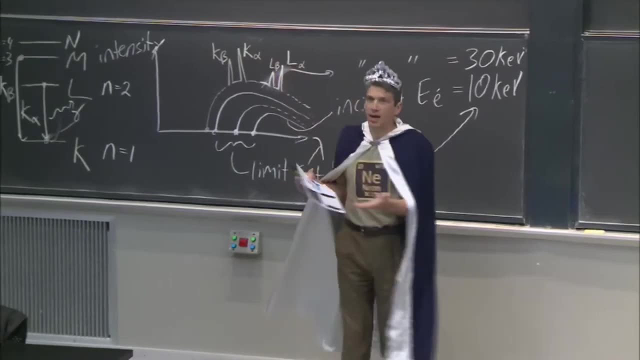 That is really useful, Because now I've got a way to have a source of x-rays that is super well-defined, It's super clear, It's always this: ah, that's so cool. As long as I have the same, It's always the same right. 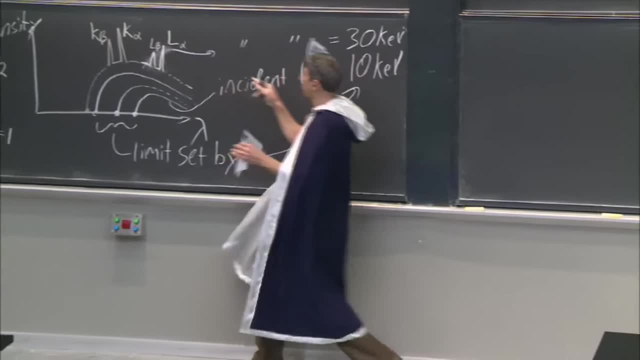 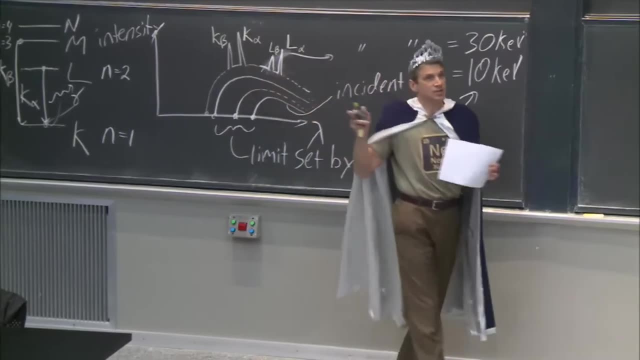 I can increase or decrease. Well, I can't go below the threshold, but I can go above it, And that peak is characteristic of the metal, So it doesn't change. That's really useful Because I've got now a flashlight. 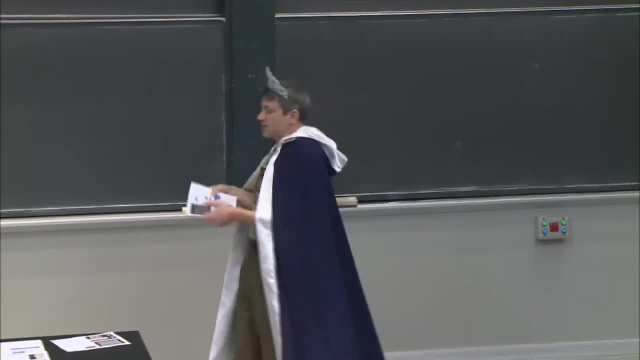 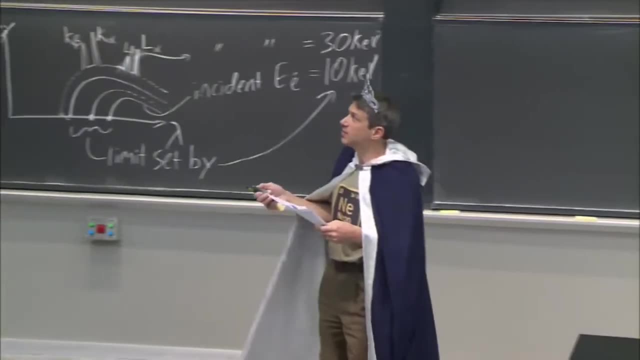 I've got an x-ray flashlight where the energy that I'm sending out is always exactly what I know it to be. I can predict what it is, and it always will be that, depending on which metal I put in there, Right? So that's a useful thing. 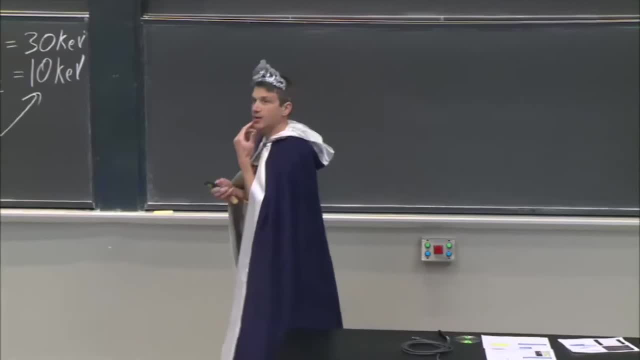 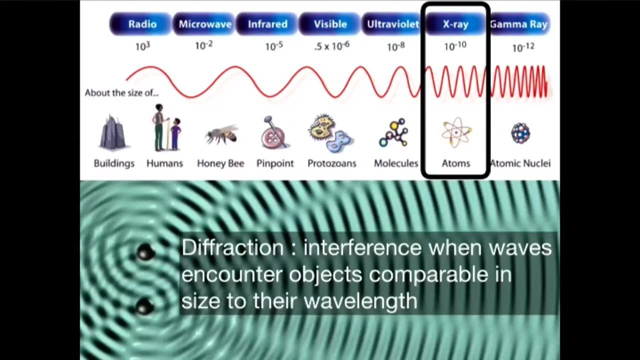 Why is that useful? Well, that gets to the topic that is the topic of today and of Friday, which is: what are we doing with these x-rays? Well, first we're generating them. So that's what we've talked about so far. 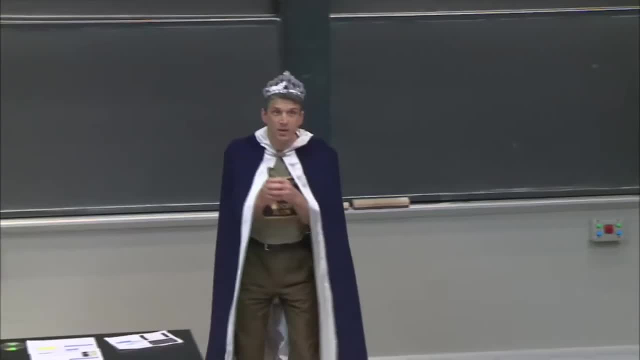 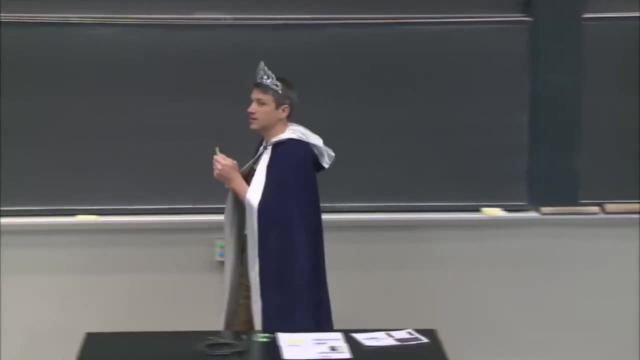 But now Gesundheit, we're going to actually use them to determine the crystal that we have. We're going to actually use them. We're going to use that flashlight, OK, And so you know, so you could. You could see why this would be useful, because here is the 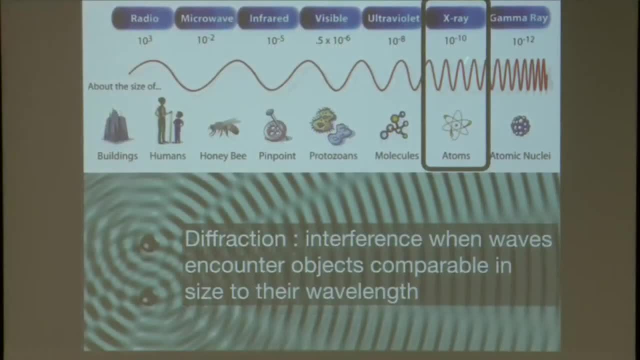 This is the range- We've showed this before right- of x-rays. So they have these energies of KeV and they have wavelengths right around a few angstroms. That is a little less than an angstrom, maybe two angstroms. 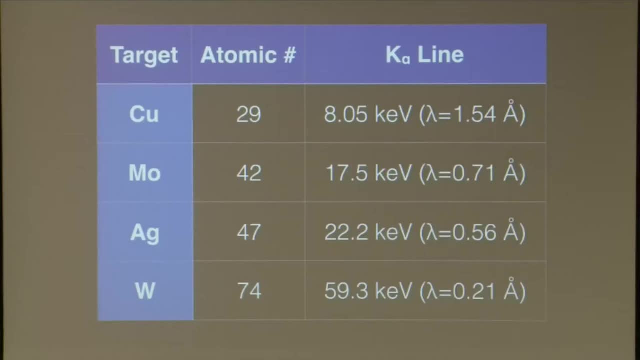 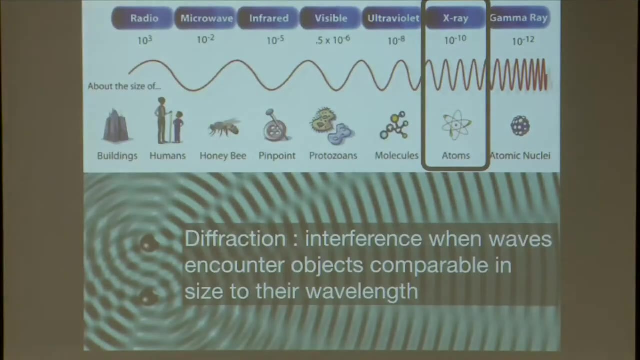 Right, See where those wavelengths are? Well, those are atomic spacings. Those are like distances between layers, right. And so if we could shine these on a crystal and somehow figure out what it is with that light, oh, there's a way we can do that. 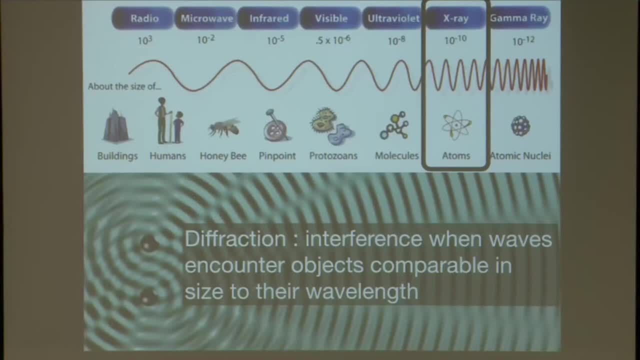 It's called diffraction, Because what happens is- and we know this from many fields- this is- you can think about this just as a water wave, any wave, OK. If the wavelength is similar in size to the features, then you get constructive and destructive interference. 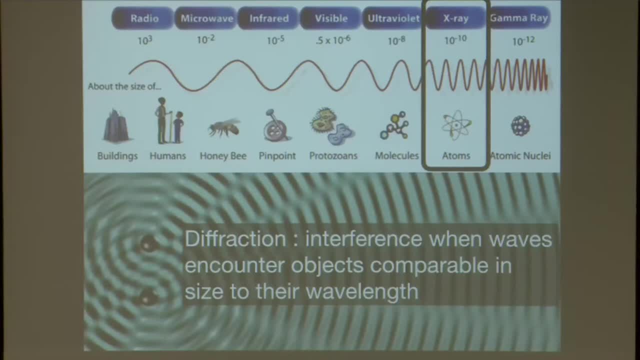 as a result of the interaction between the wave and the features. So that's called diffraction right And you can see it here with this very simple picture of, say, a water. this could be like a water wave, a sound wave, you know, and there it is. 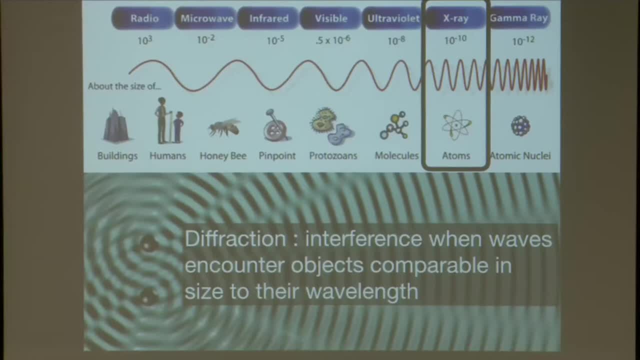 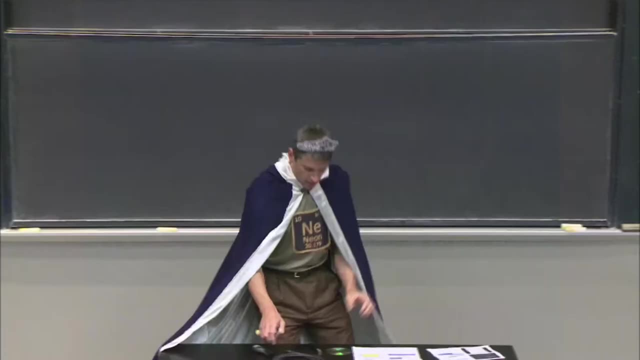 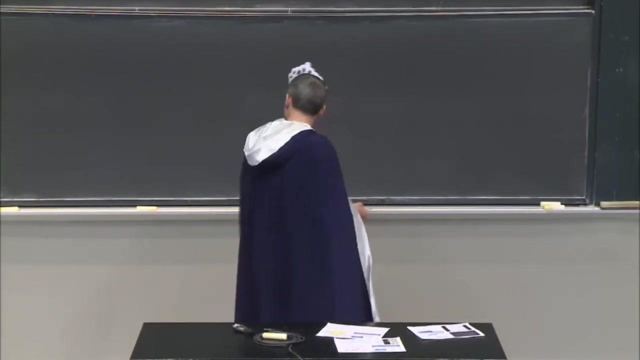 And it's interfering both constructively and destructively along these lines. right, You can do this, test yourself, You could take- I highly recommend this, take- a laser pointer. And now, if I just had a piece of metal, I don't have a piece. 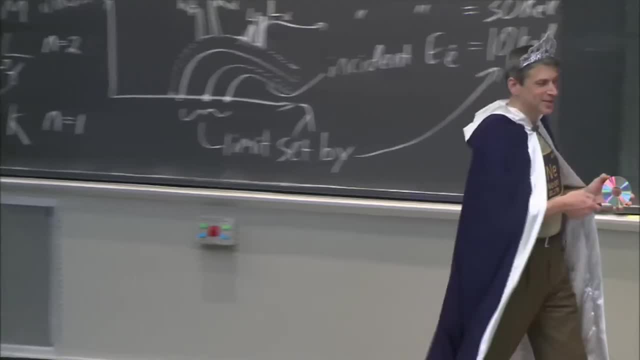 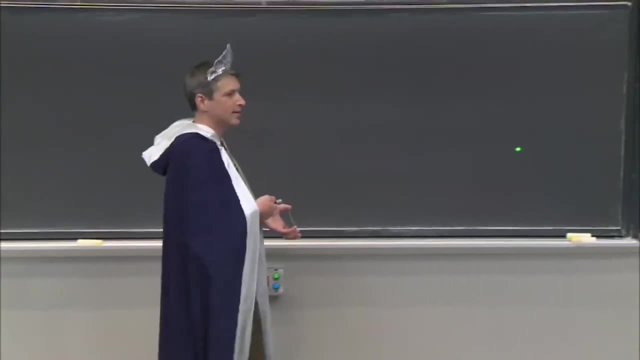 I don't have a piece of metal, But if I did, then I would shine it on it And what you'd see is that the dot would just reflect off the piece of metal. OK, So I just would get the dot back, right. 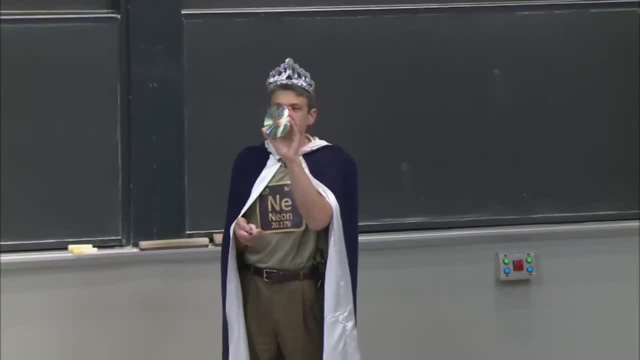 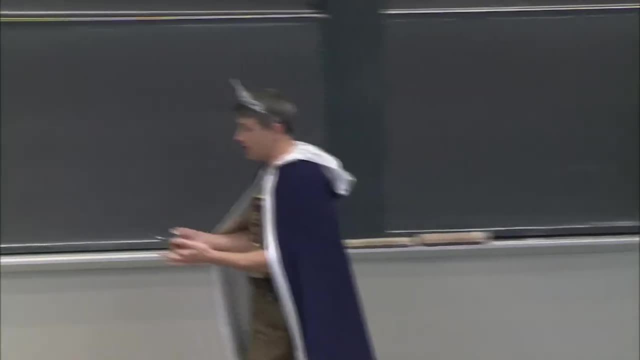 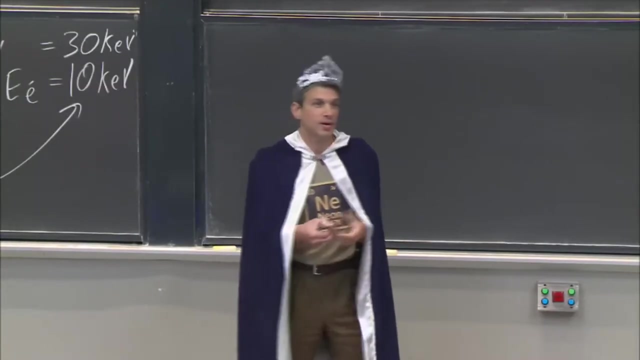 But now I've got this thing here, this we. many of you may not know what this is. This is called a CD, OK And oh, but it turns out that a CD has features and it's got trenches that are like, you know a little less. 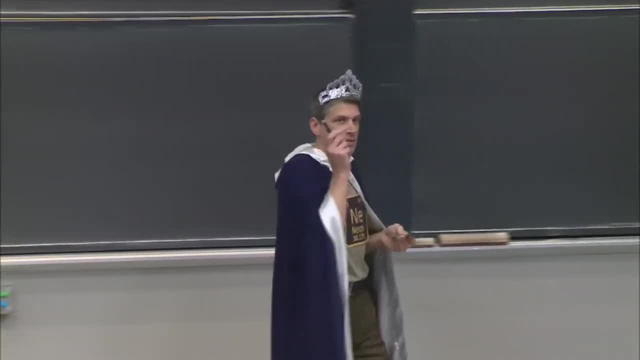 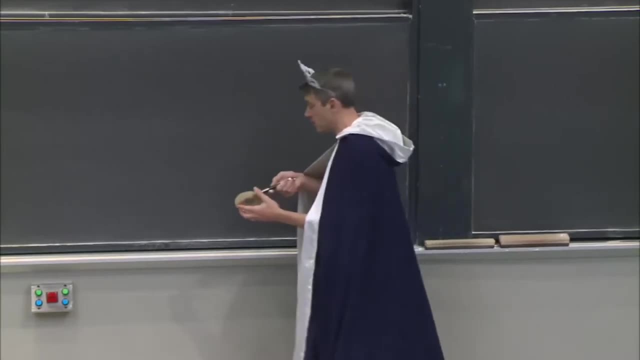 than 900 nanometers, And this is 500 nanometer light. So you would expect there to be diffraction, You would expect there to be constructive and destructive interference, And when I bounce it off of this, look at that. There it is. 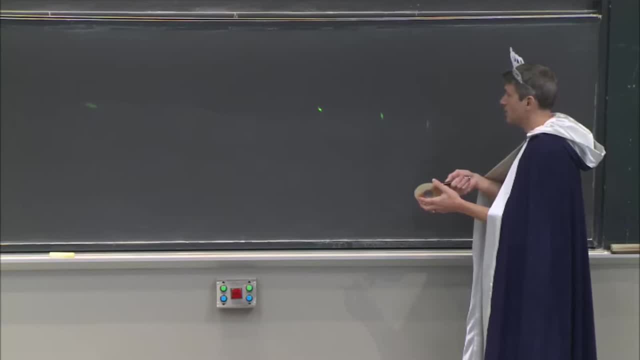 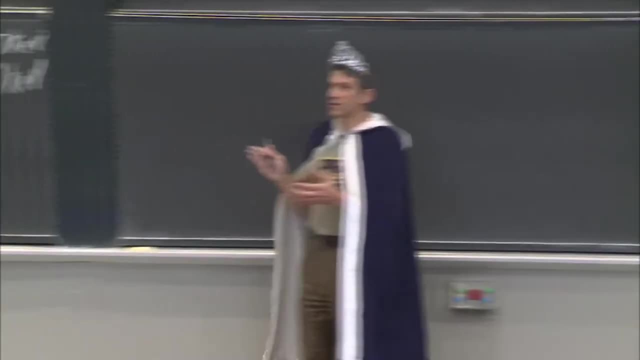 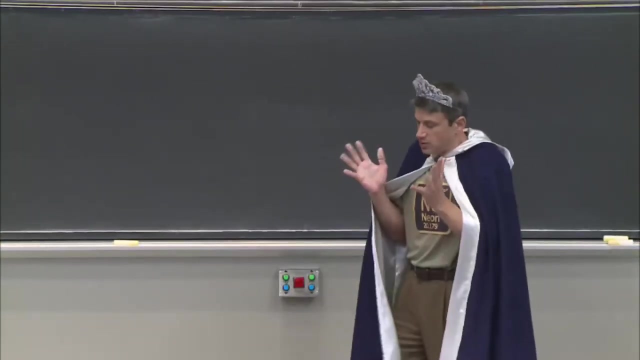 This never gets old. I'm not getting just one reflection here, I'm getting a whole scatter of them that have constructively interfered because of the feature sizes being the same as the wavelength. OK, but now I want to do that with X-rays. 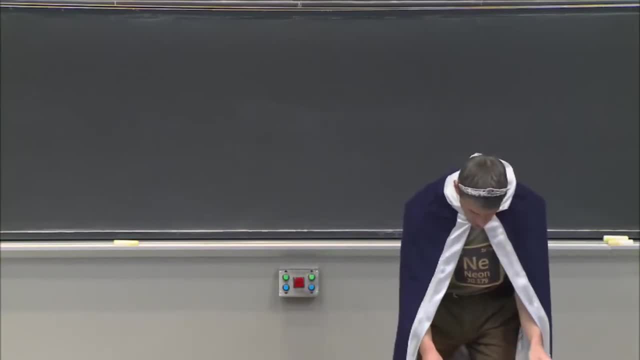 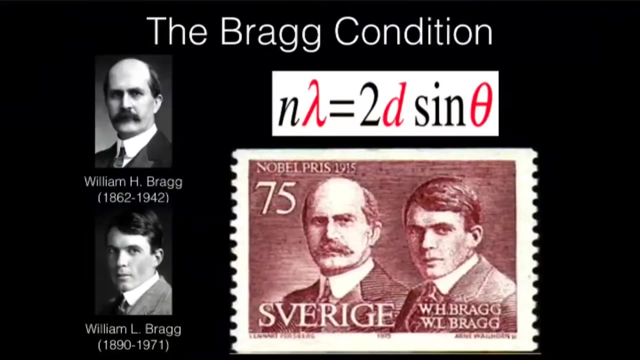 And I want to do it onto crystals. So how do we do that? OK, so let's think about that, And we're going to think about it in terms of what the Bragg father-son pair, who won the Nobel Prize and are on a stamp. 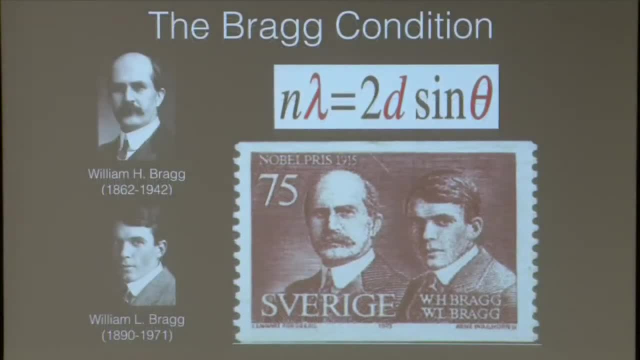 That's what you get when you win a Nobel Prize, I guess. And what they did is they figured out how to do this. OK, So let's go through that, just so we understand it conceptually. OK, so I'm going to say that I have a set of atoms. 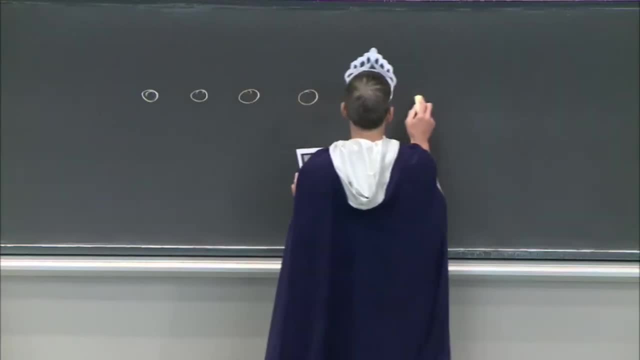 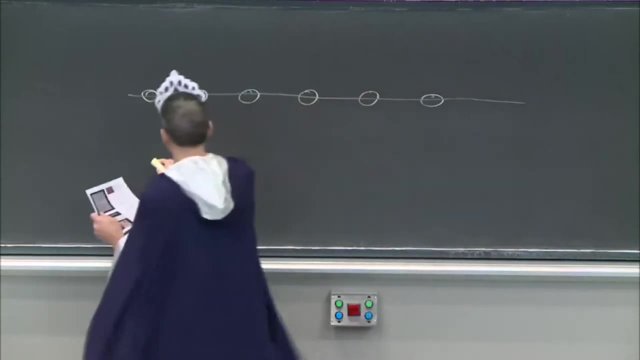 Now, right now, I'm not going to worry about what they are, But I'm just going to say that there's some plane of atoms here And there's another plane of atoms beneath that. OK, So there's another one, and so on, and so on. 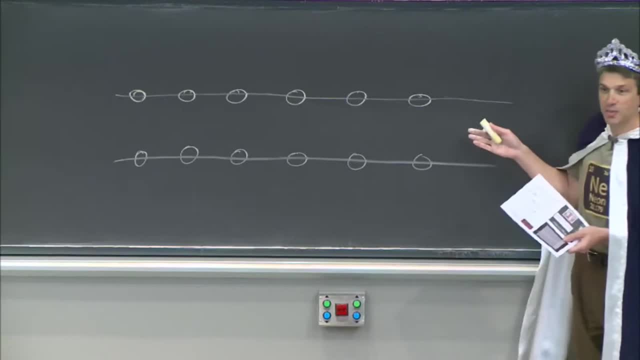 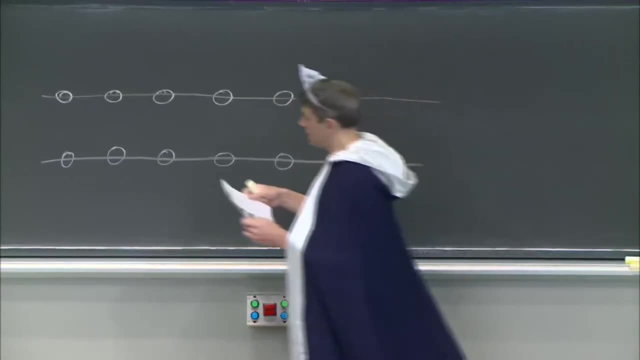 And now, these would be Miller planes, Right, These would be Miller planes in the crystal, And let's just assume they're very, very simple: this plane and that plane, And now what I'm going to do is I'm going to have some X-rays. 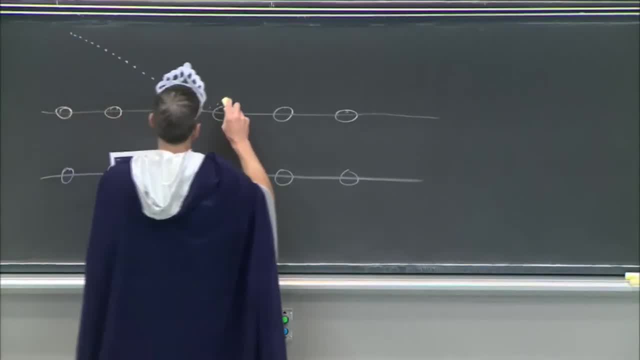 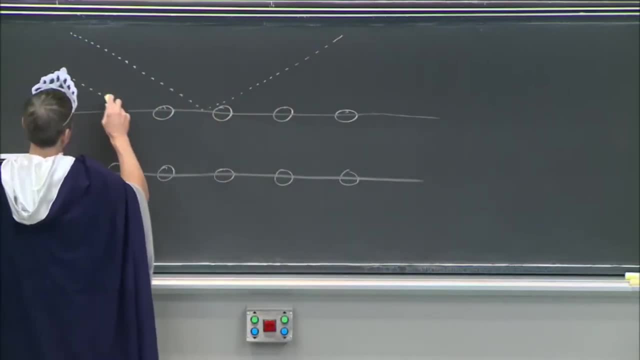 I'm going to have some light shining on this And it's going to be incident and it's going to be reflected. But see, I'm going to have another wave here. OK, let's see if I can get through this drawing. 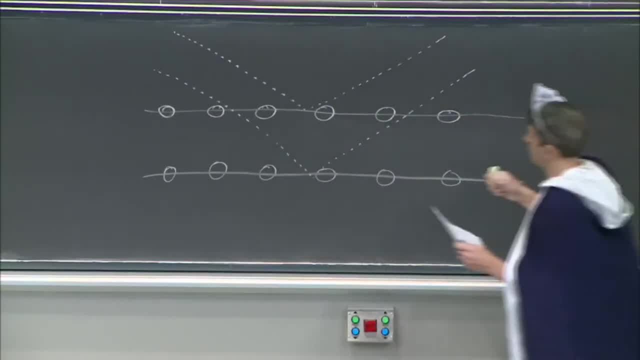 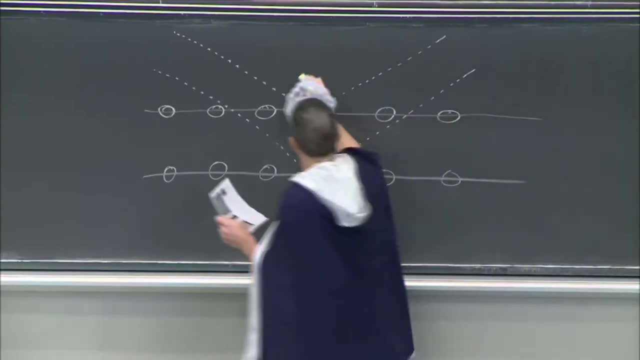 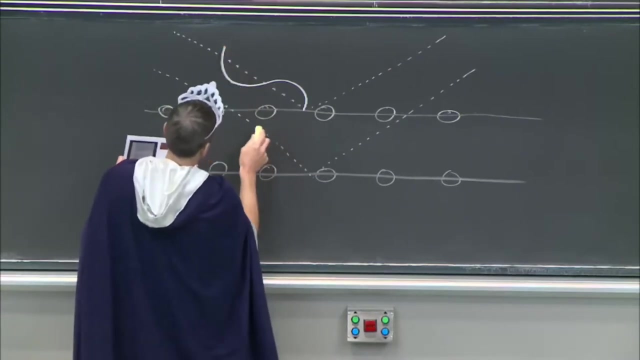 Sort of almost kind of. Now, Here's the deal. OK, These are waves, right, These are waves. So if I want to draw this as a wave, I might draw it like that, And if these waves are constructively interfering, 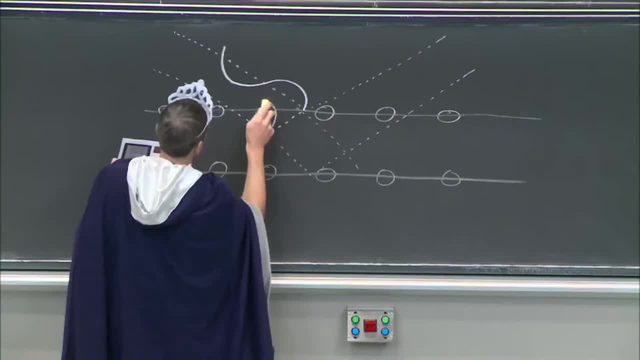 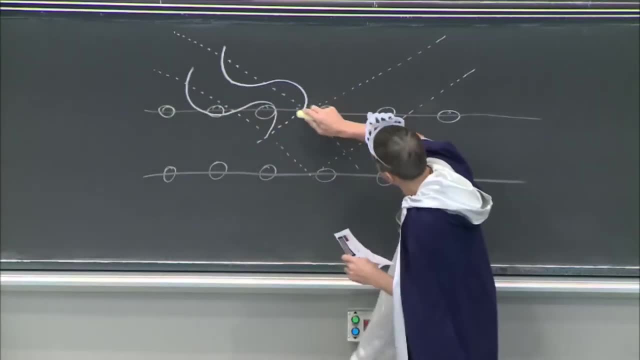 let's just complete that. then this wave would look like that. If they're in phase, then that's what they would look like. Now this one's getting reflected off the surface, right, So I'm going to do that reflection here, OK. 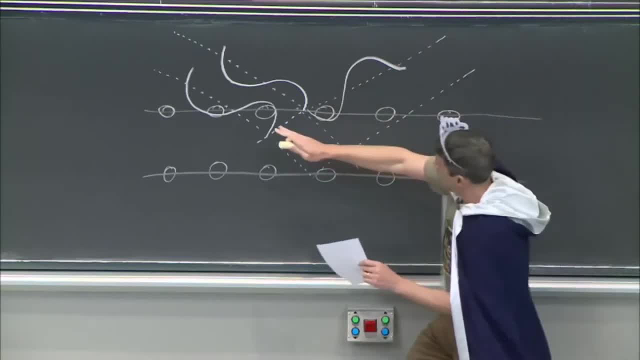 And if I want it to come back off of the surface- and this one got through the first layer- this didn't get reflected. It's going down, And if I want it to come back up, then this one must also look like that to be in phase. 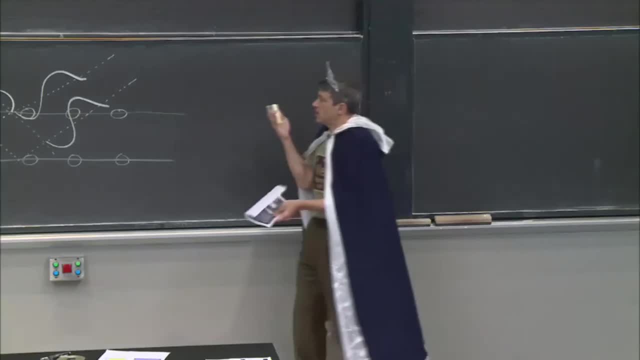 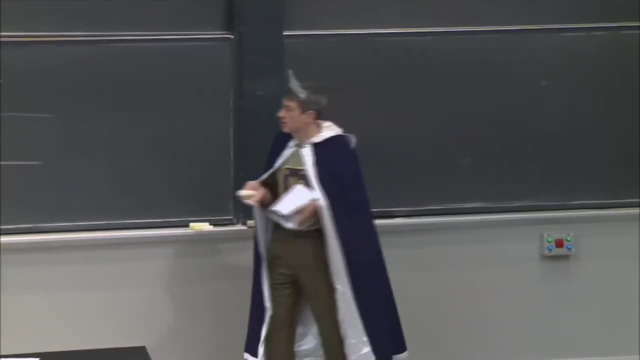 right, They must be in phase as they come out, or else they're not going to interfere constructively. See that? So those are my X-rays, right, They're waves, They're just waves, right? Oh, But this is the whole secret, right? 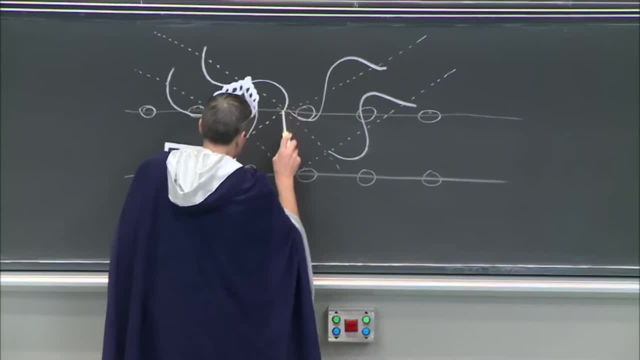 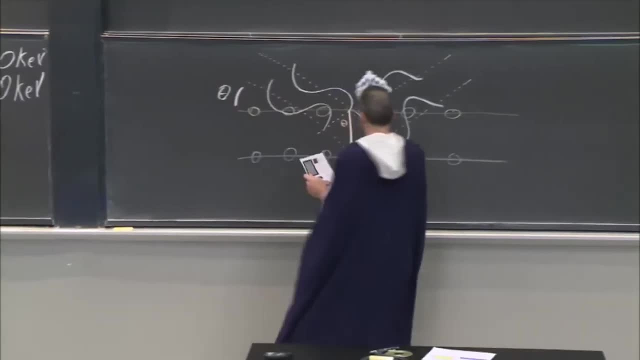 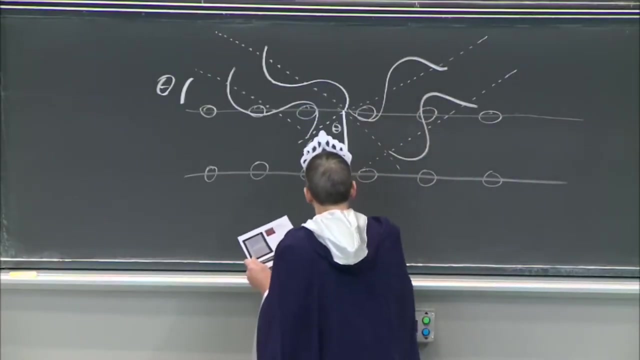 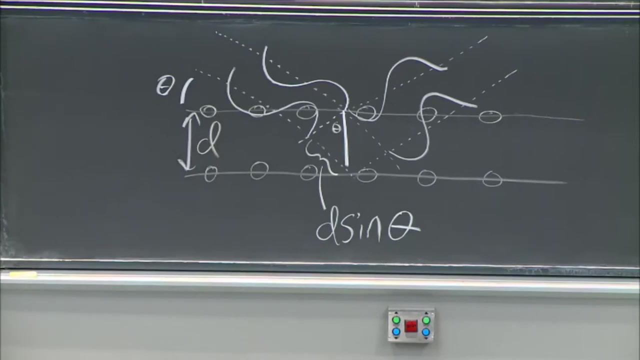 Because if this angle here is theta, then what that means is that this angle is theta, OK. And if that's true, then this distance is d sine theta where this is d. That's just some simple geometry, OK. So what you know then is OK. now we're getting somewhere. 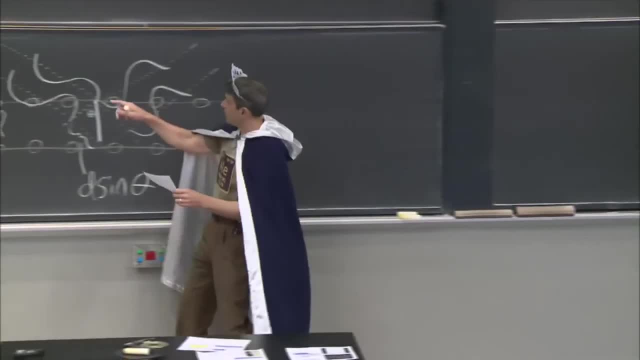 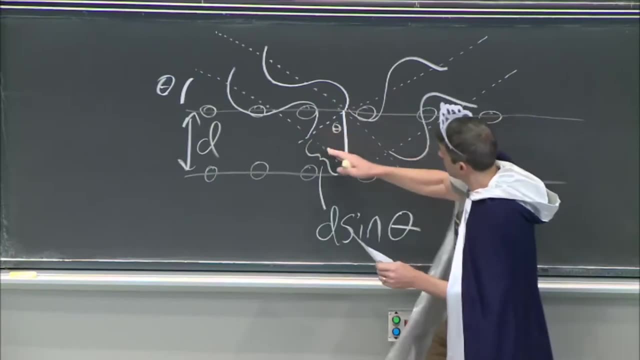 right Now we're getting somewhere Because you know, if I had a wave, this is one wavelength right, And so if I had a wave, come in like this, and one of them is going to get reflected off of this lower surface and the other one 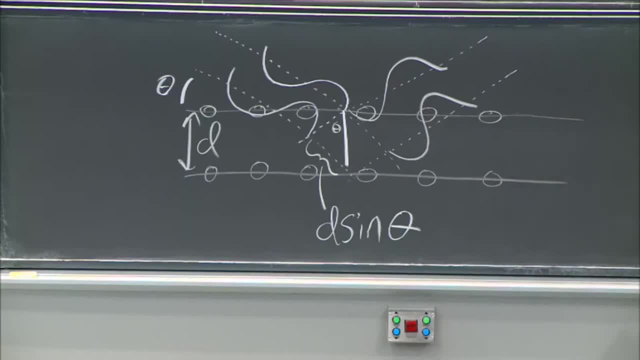 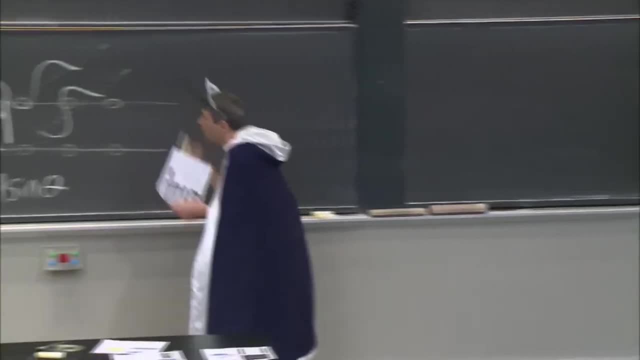 got reflected off this, but I don't want them to interfere in any way, but constructively. That's what Bragg said, Bragg and Bragg. That's what they said, Then the other one, And the only way for that to happen. 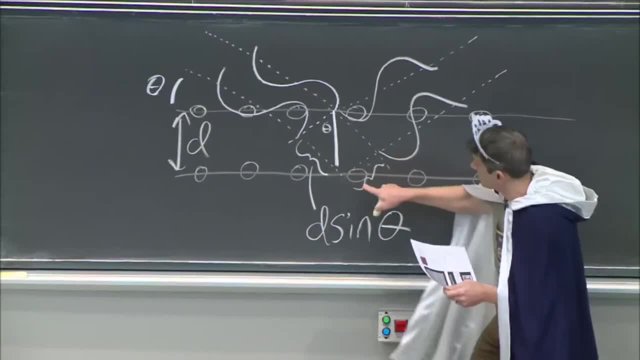 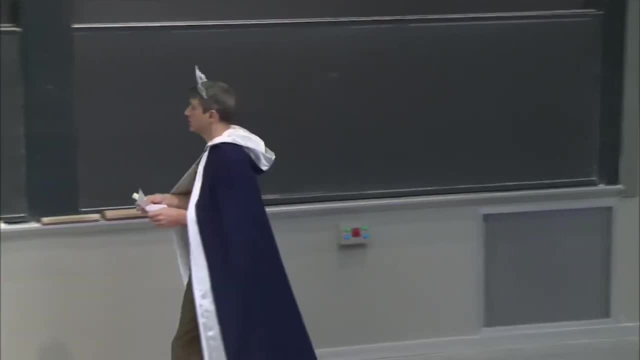 is if this distance plus that distance, so d sine theta plus d sine theta, is equal to some multiple of the wavelength, It has to be right, And so what you get is: well, that's what they have there, And lambda, some multiple of the wavelength. 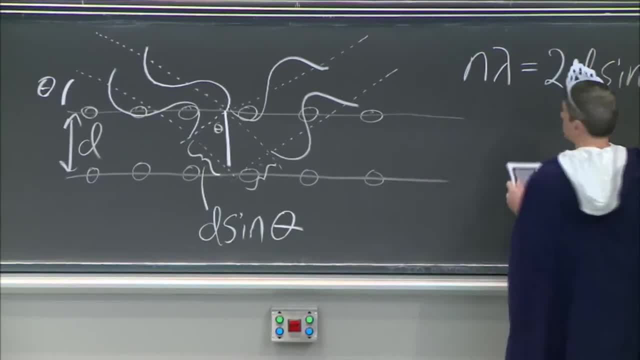 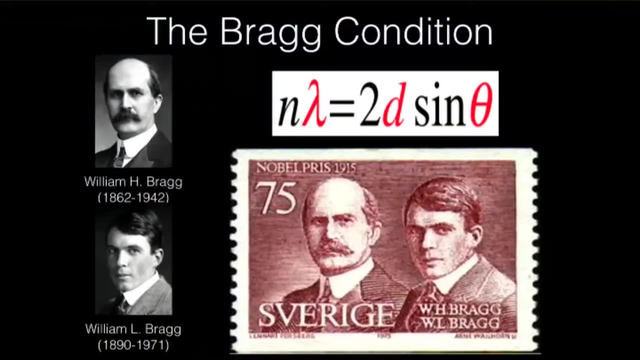 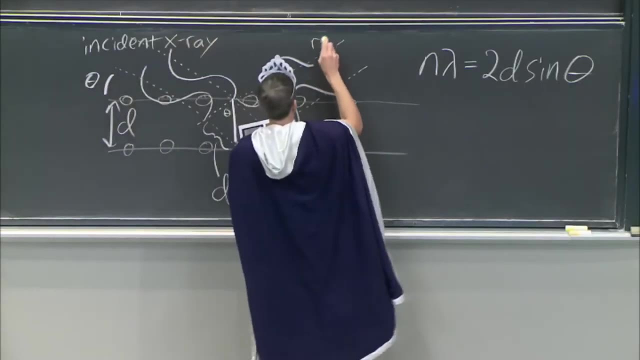 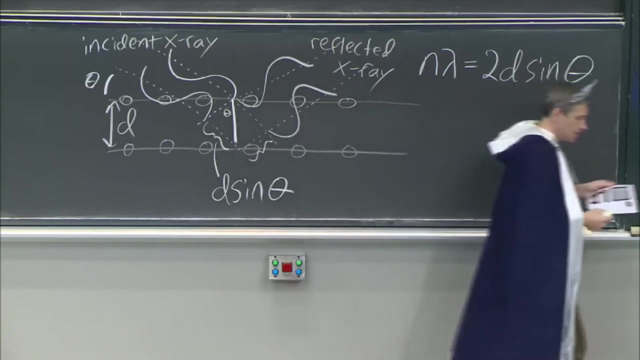 equals 2d sine theta, where theta is the incident angle of that x-ray. OK, So this is incident, Just to be clear, incident x-ray. and these are reflected, Reflected x-rays. OK, Now to keep it simple in this class. 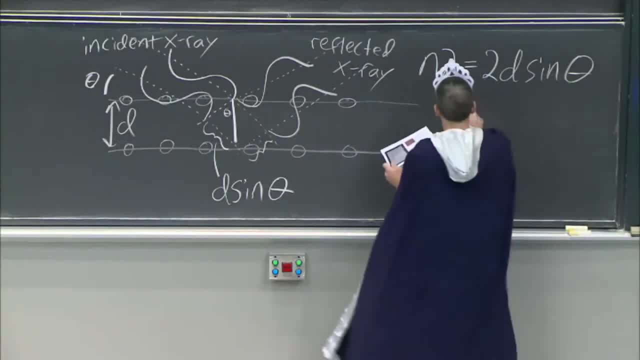 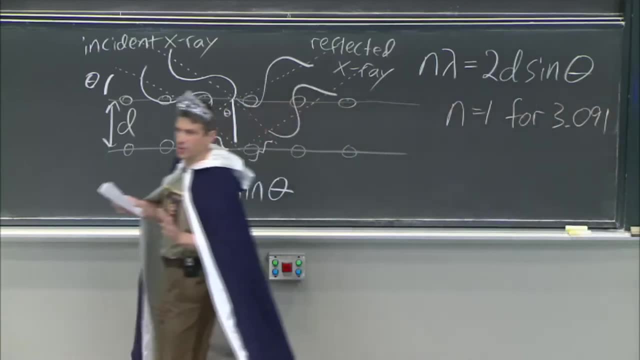 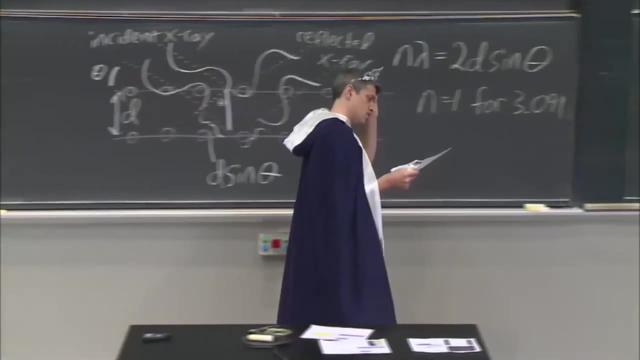 we're just going to say n equals 1.. n equals 1 for 3091, just to keep things simple, Because we're really just. I want to grasp the basic concepts here. All right, We're not using x-rays to get the structure of DNA. 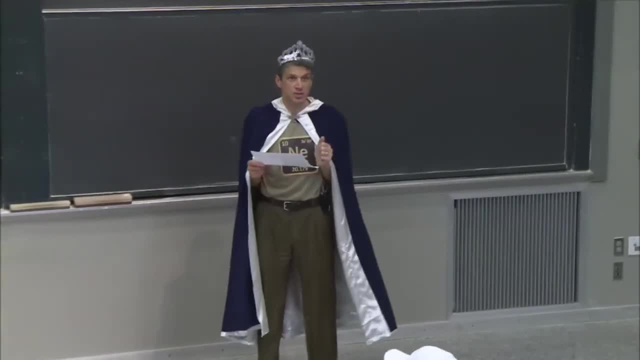 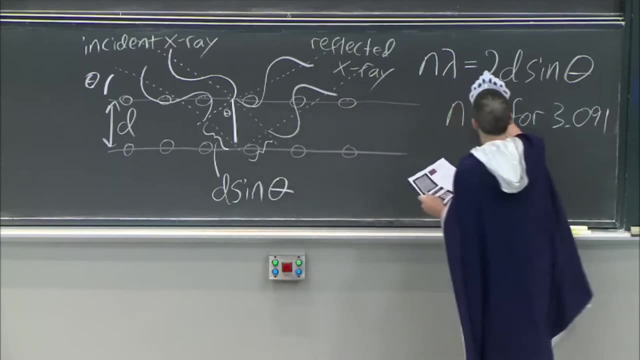 but we're going to use x-rays to figure out cubic crystal structures. We're going to show how that works Now. so this must be true, for so this is in parentheses for constructive interference. Constructive interference, Those dots that you saw- interface. 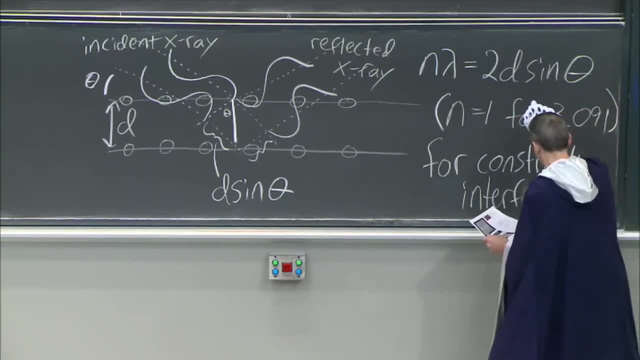 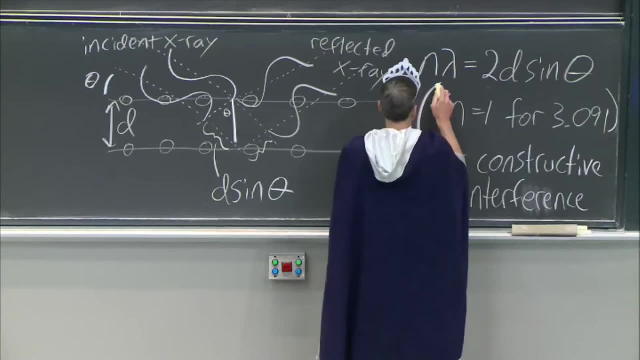 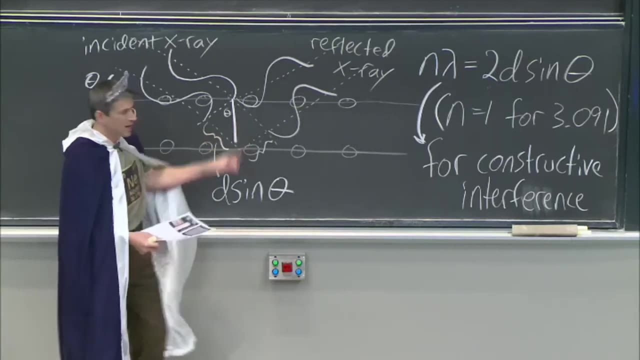 Interface, Interface, No Interference, Interference Right, For this is true for constructive interference. Of course you could write any equation you want, But if you want them to be constructively interfering when they come out, that has to be true. 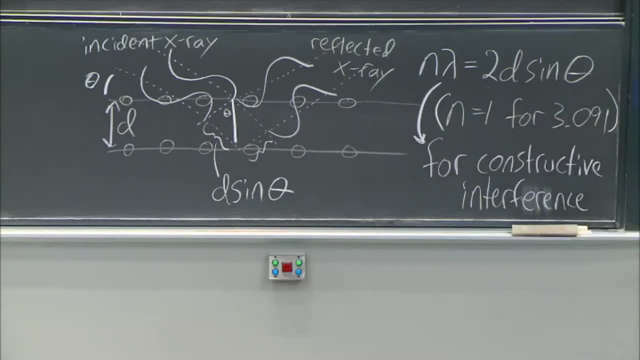 And that's what the Bragg said. But see, we're not there yet, right, Because now we've got to do experiments. OK, So, we've got to do experiments. So what does this mean? Well, OK, OK. 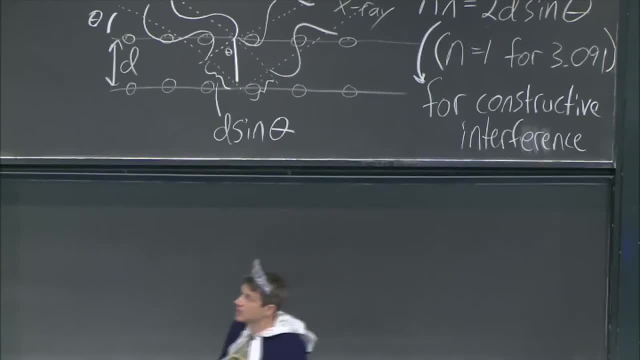 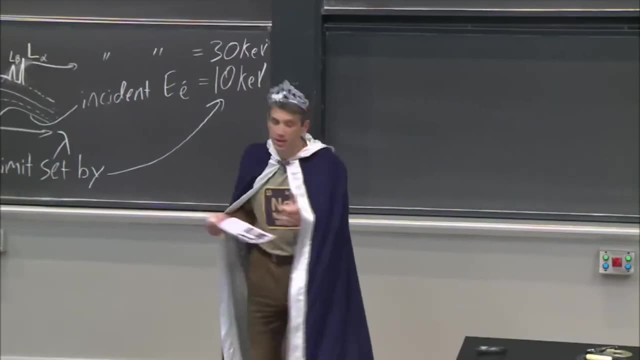 I'm going to take x-rays of some lambda- OK, And I'm going to shine them on a sample right, OK, And I'm going to measure. So what I'm going to do, oh, I think I have a picture. 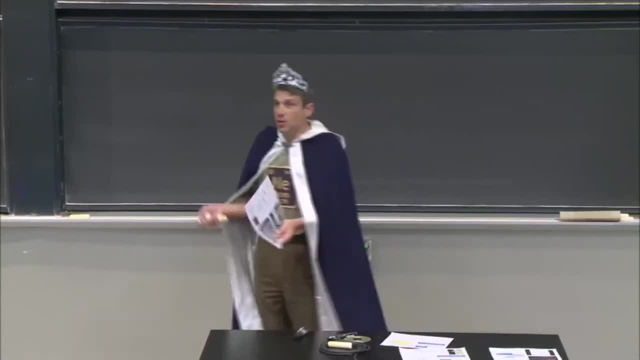 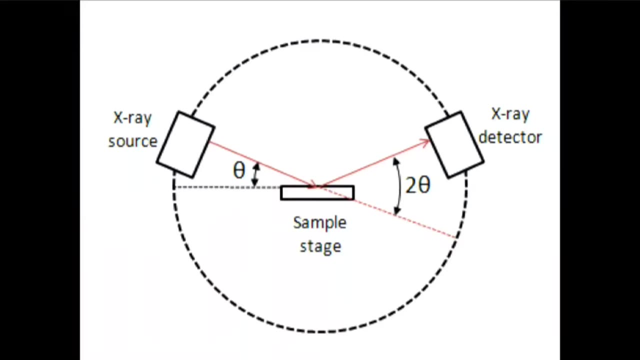 I'm going to measure. There it is. This is what an x-ray diffraction experiment looks like. OK, So I've got some sample And I shine x-rays. I've got a source of x-rays. We now know how to make that source right. 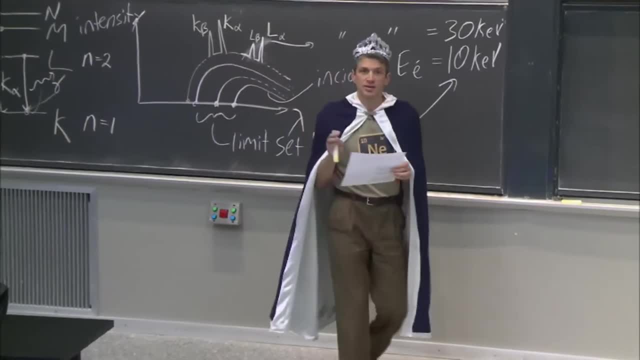 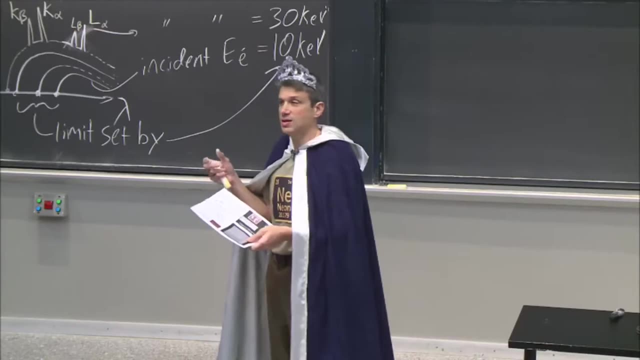 And we'll just filter out one of these lines, right? Oh OK, So I've got that source And I can change the angle, And then I've got a detector And I can measure: did I get interference or not? 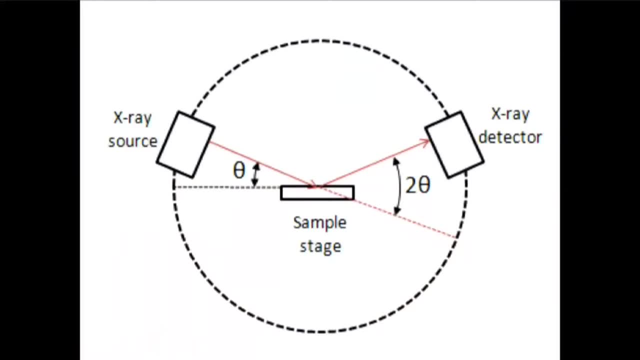 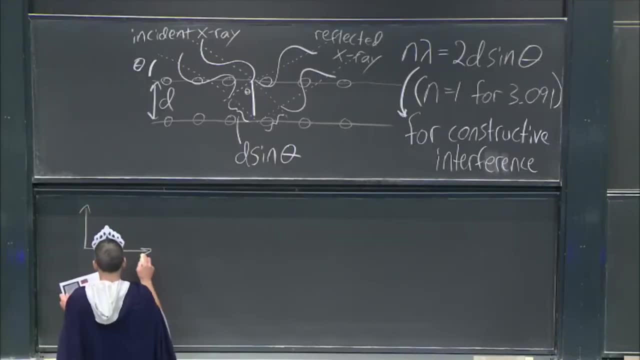 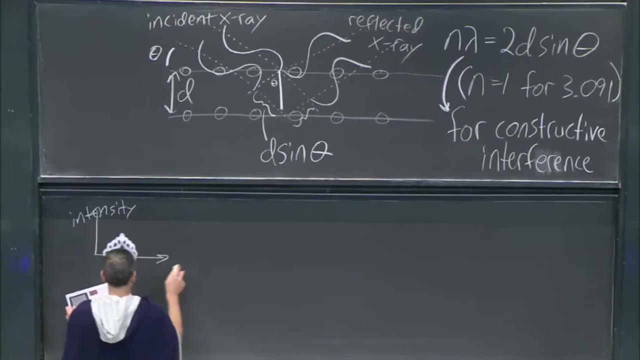 It's just like the dots, right. So now we know that if I do that and I say I scan the, I'm like OK, so I've got intensity And now I'm plotting it with angle. So now I'm moving this intensity. 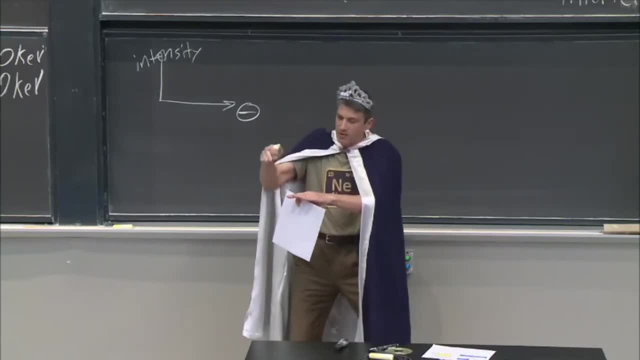 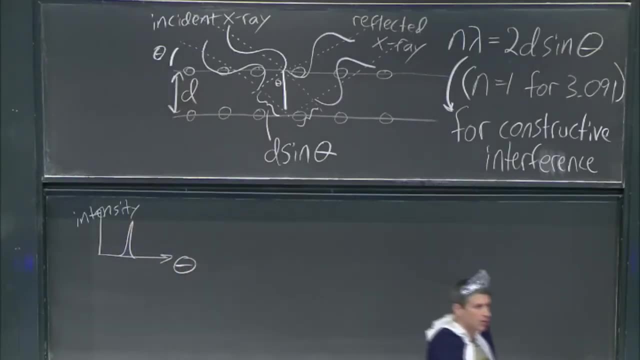 I'm moving the angle around And I'm changing it and bam, I get interference And I see a spot in my detector. So literally it would look like this: right, You would get some angle where there's interference And the detector would say ding ding, ding, ding, ding. 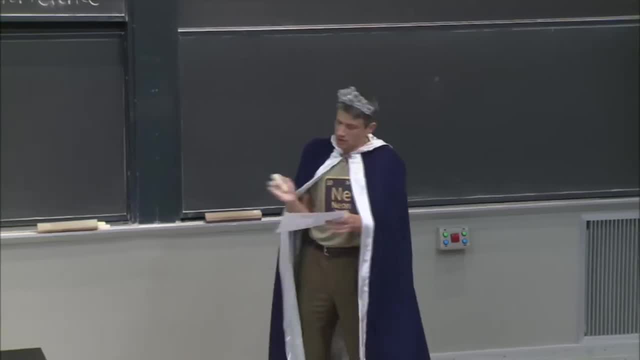 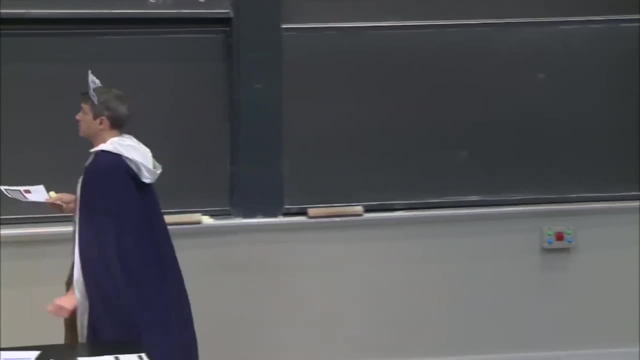 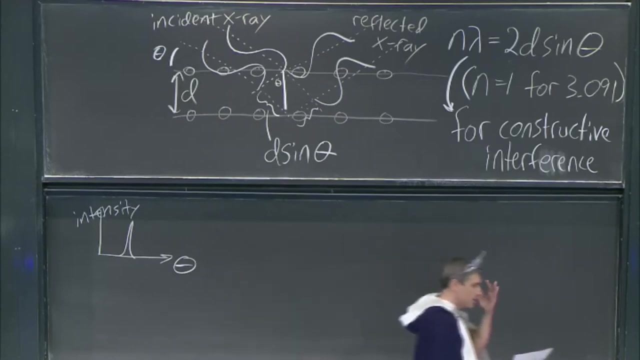 I see a lot of x-rays coming off, And now you change the angle by a few degrees and I don't see anything right, Because it's all destructive from these crystal planes. OK, OK, So it seems like then, if I just vary theta, am I there yet? 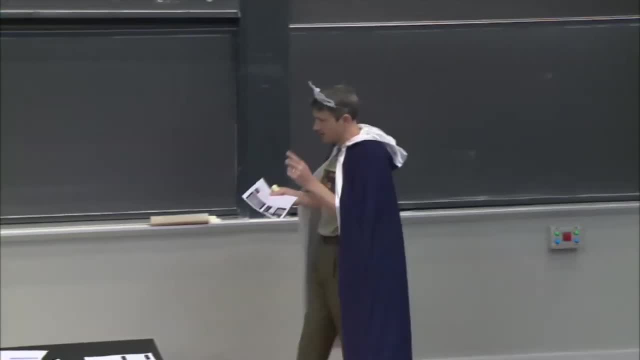 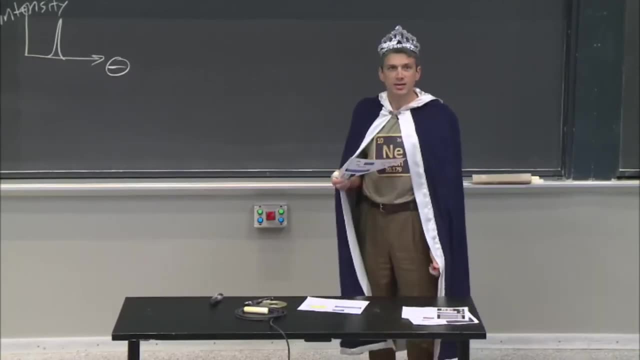 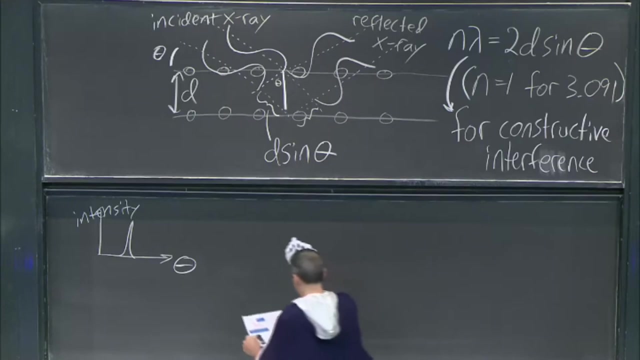 The problem is that I might not know d, I might not know d, Aha, but we do know d. We do know d because we learned about d For cubic crystals. we know d Because, for cubic systems, we know that d of h, k, l. 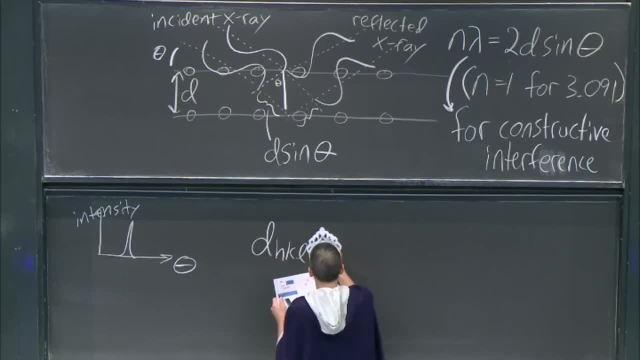 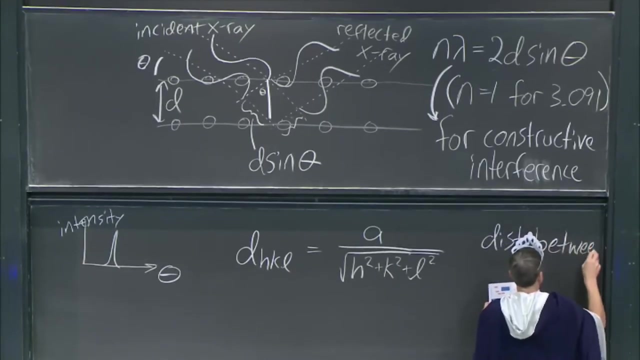 of any plane. the distance between those planes is equal to a over the square root of h squared plus k squared plus l squared, And that's something that we learned. This is distance between Miller planes. Miller planes, Gesundheit In a cubic crystal. 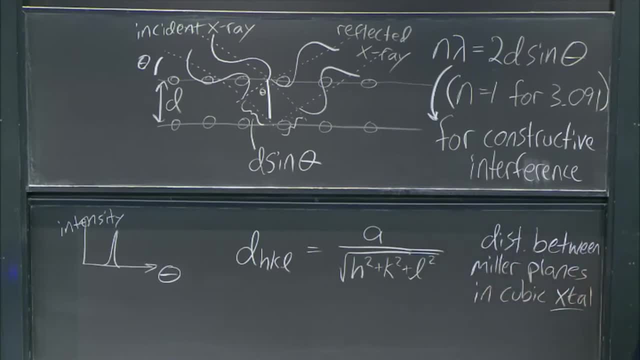 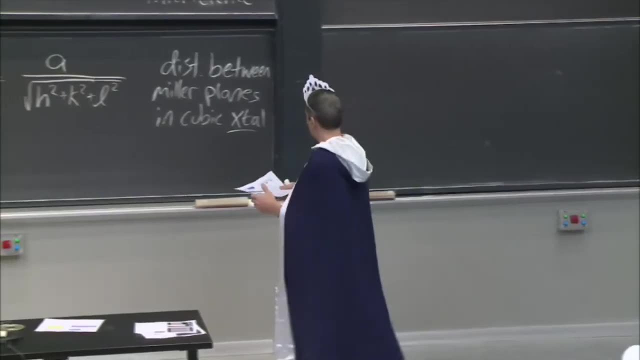 Oh, I'm saving time. I wrote extal. I saved a lot of time, which I just wasted by being so proud of it. OK, So I know d Well. OK, so what does that mean? Well, let's take a look. 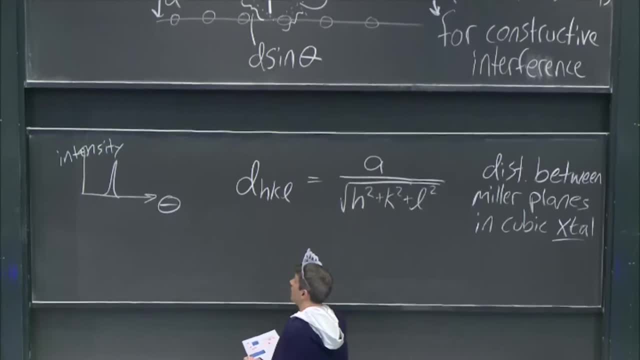 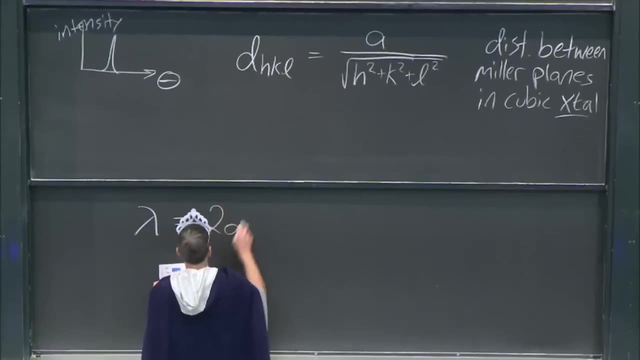 Because now I'm going to go back. I'm going to go back to my equation And I'm going to say, OK, lambda equals 2d, And I'm saying n equals 1, OK, And I'm going to be very specific. 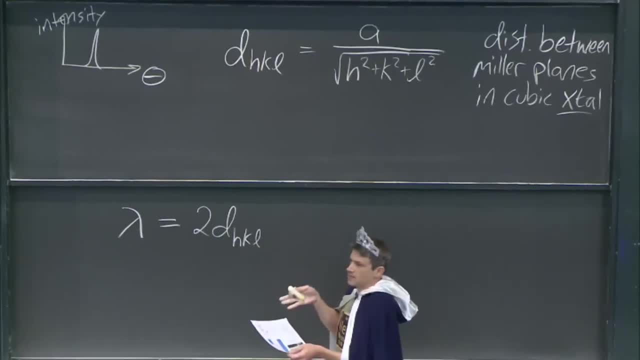 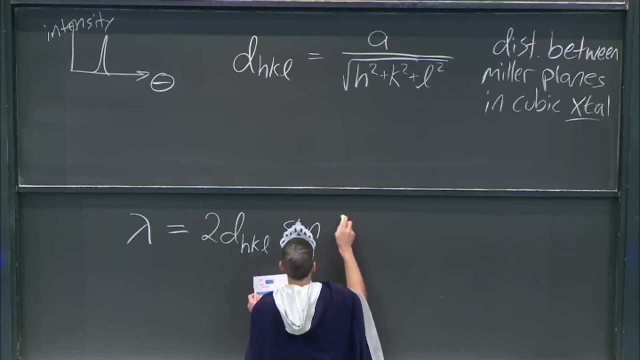 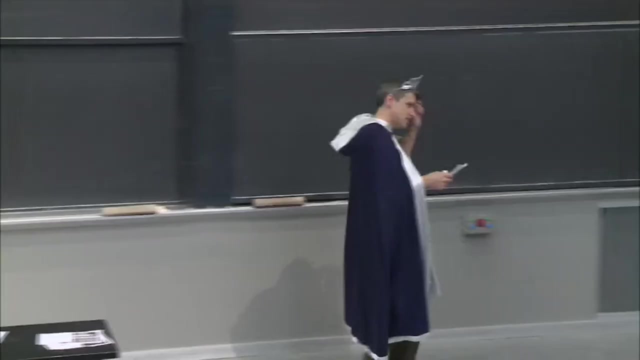 This is now a d that comes from the spacing between planes that are specified by the Miller indices. times the sine of theta, And I'm putting h k l on the theta as well, And you'll see why. Because here's the thing. 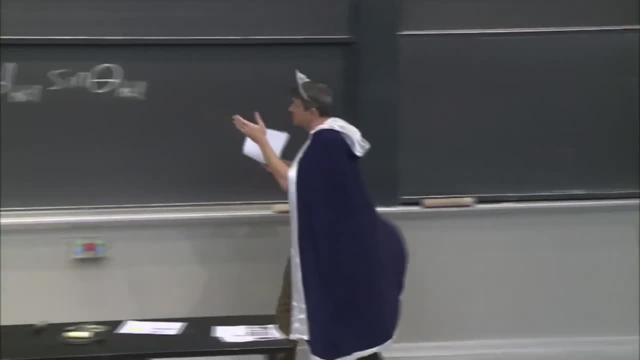 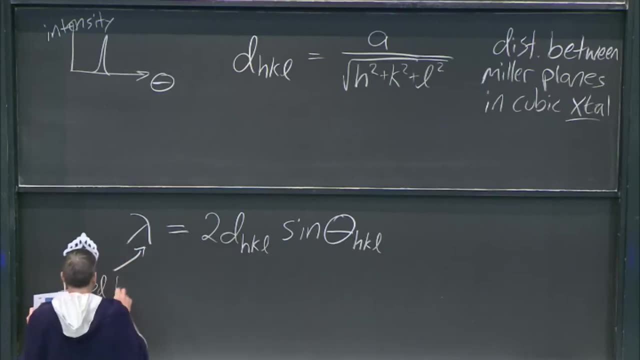 Now I've got constants. Now I've got constants Because, look, this is fixed, Fixed by the source, by the source. So this is a constant. If I have copper, then it's 1.54 angstroms. 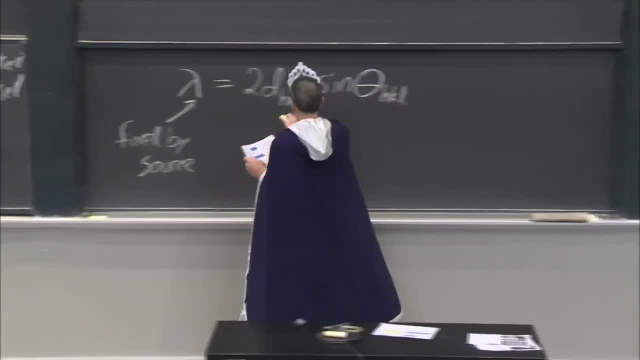 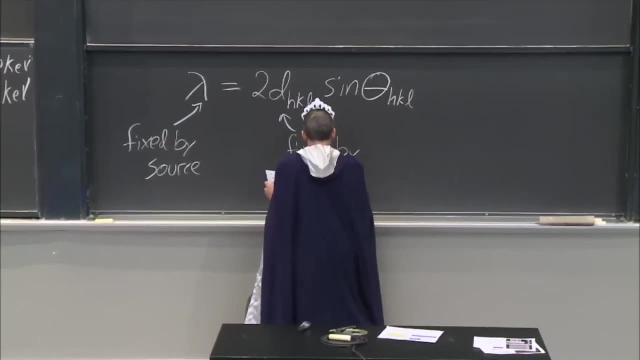 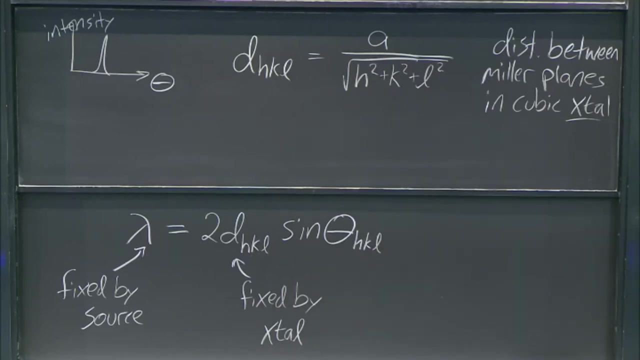 This is a constant. This is fixed by the crystal. That's also a constant, Fixed by the crystal. because that's also a constant, Because it's the lattice constant, right, We're not changing that. So for a given set of planes, that 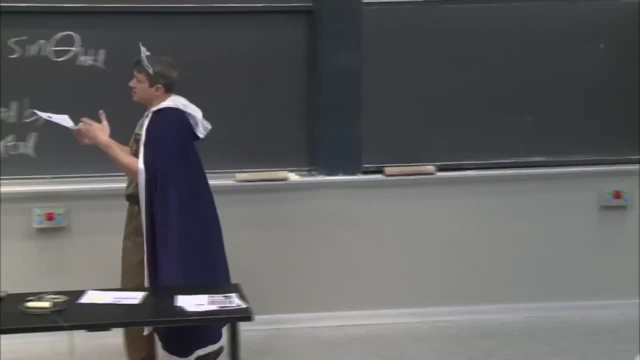 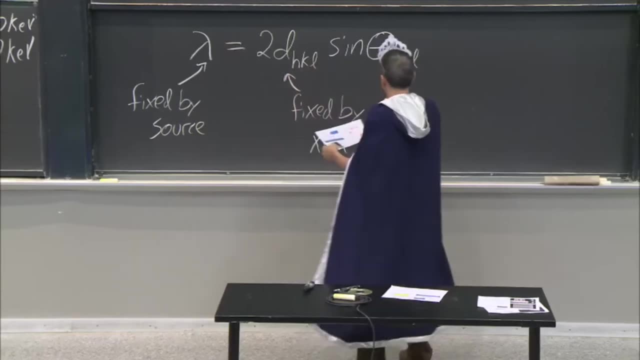 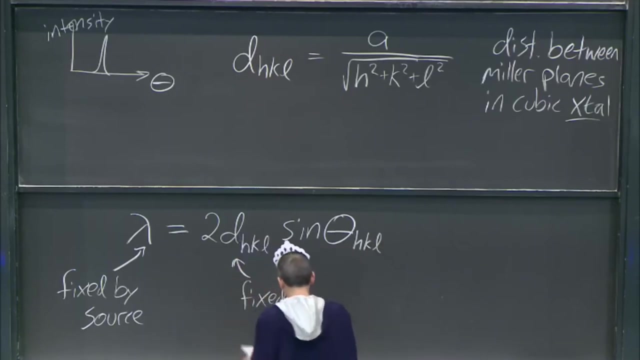 these waves are bouncing off of and maybe constructively interfering with, depending on the theta, then these are constants, right? OK, So if I regroup them, so I'm going to regroup them right, And so I'm going to say that let's see. 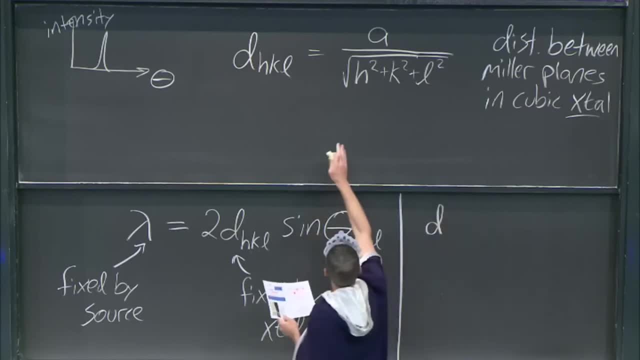 d. so I'm going to substitute in that expression up there down here, OK, And I'm going to use a copper source, right? So I'm going to say, well, let me go through this one step at a time. 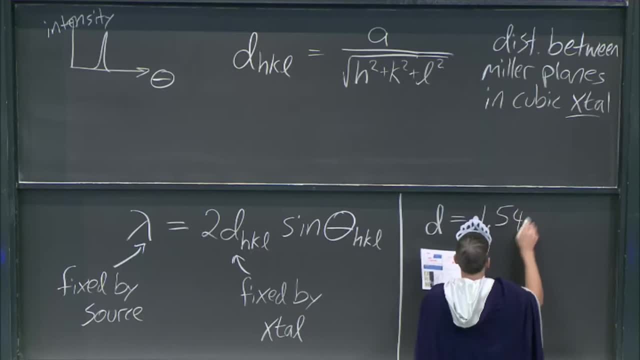 So d equals 1.54 angstroms over. let's see 2 sine theta hkl. Now what have I done here? This is for a copper source, So I'm now adding in, I'm fixing in the constant, OK. 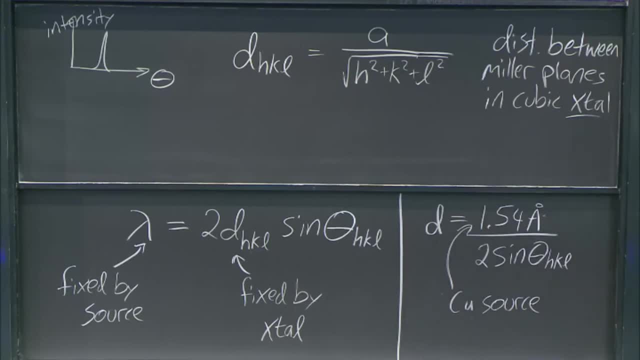 Fixing in the constant. OK. So that's the Bragg condition, But I also know that d is equal to. it's also equal to ah. I don't want to write it again. It's also equal to that, OK. 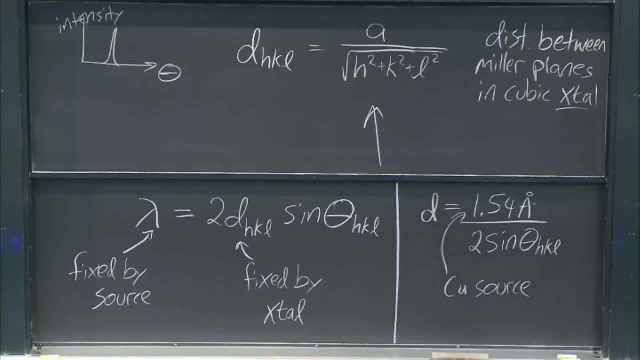 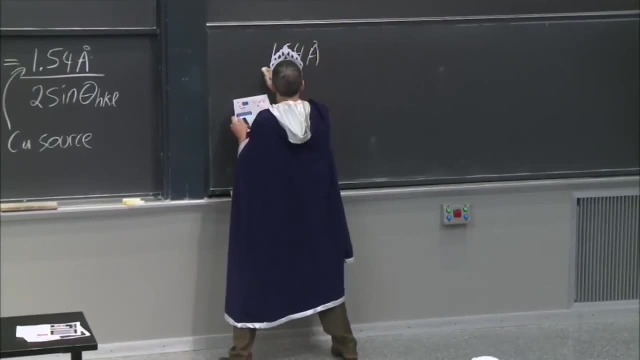 Good, OK, So let's put that together. We'll do a little division And what we get is 1.54 angstroms over 2a squared. The whole thing's squared. I'm squaring it. I don't want the square root. 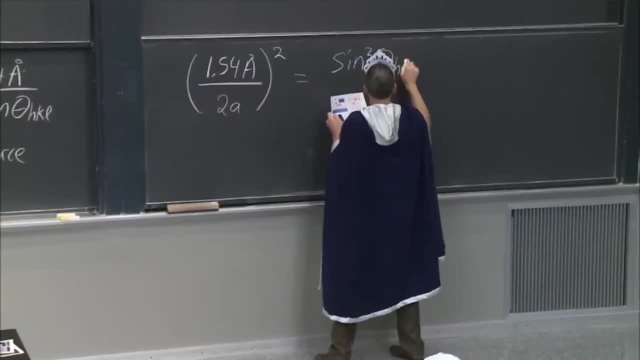 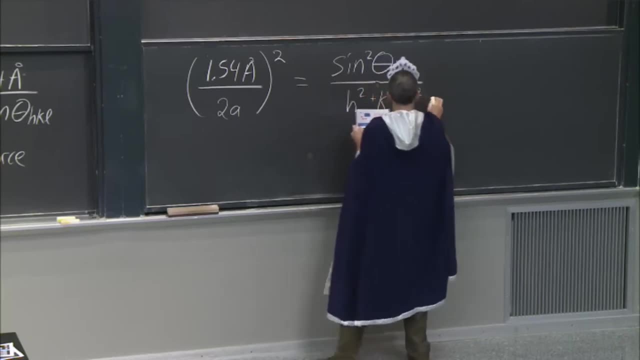 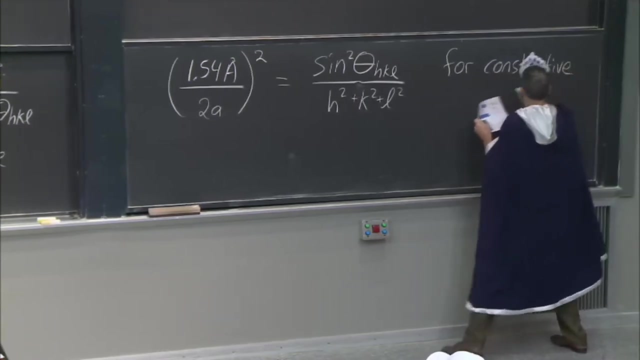 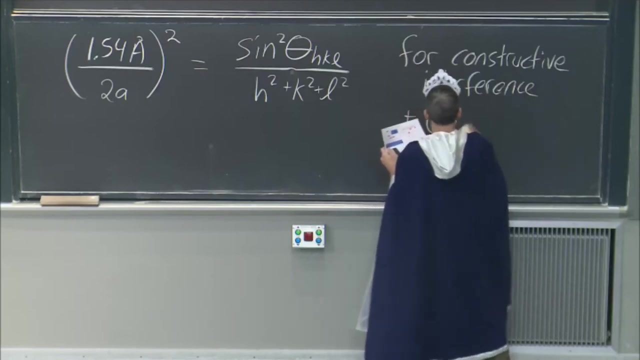 Equals sine squared theta: hkl over h squared plus k squared plus l squared For- let's be very specific- for constructive interference, OK, Constructive interference and a copper source. So now I'm getting specific, because this is how experiments work. 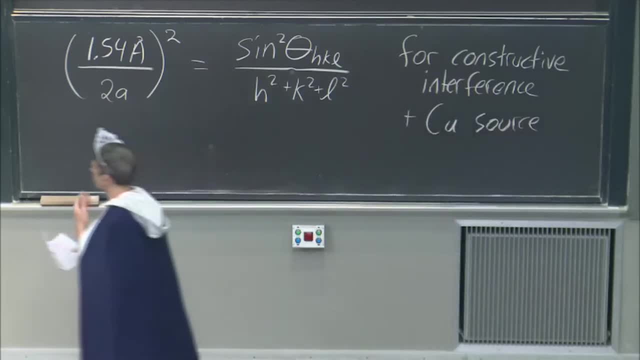 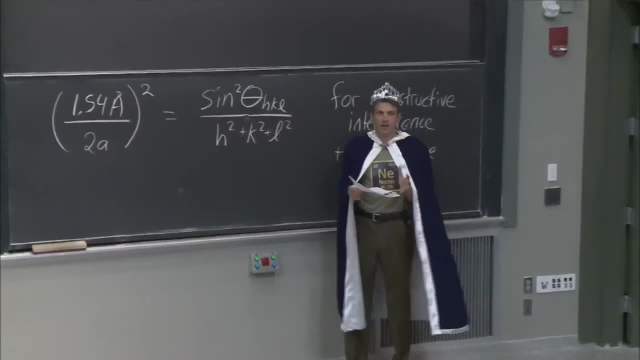 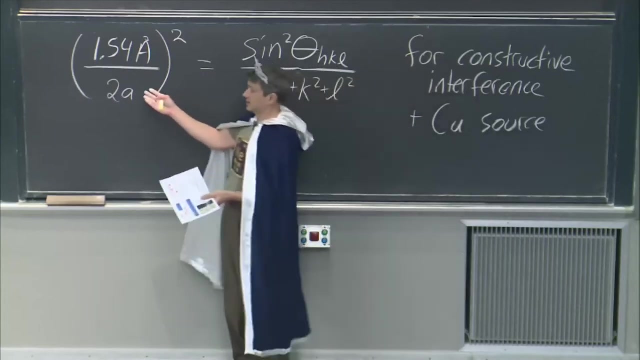 Experiments with x-ray diffraction are done right. So now, the last time I checked, if you got something equal to a constant, then that something also is a constant right, And this is a constant, And so what I need to do now is figure out right. 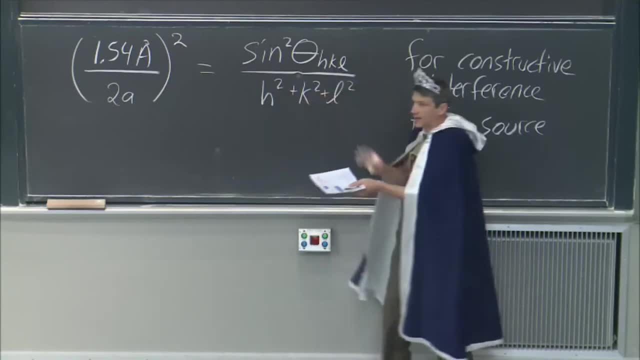 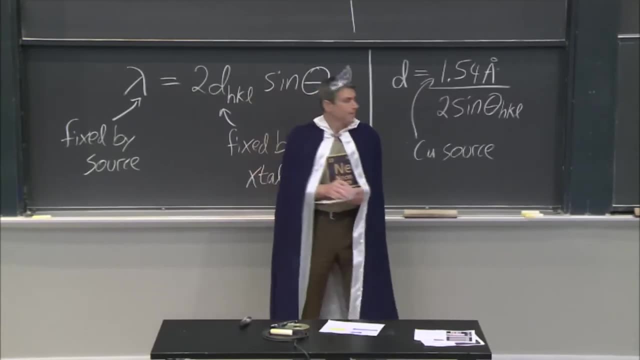 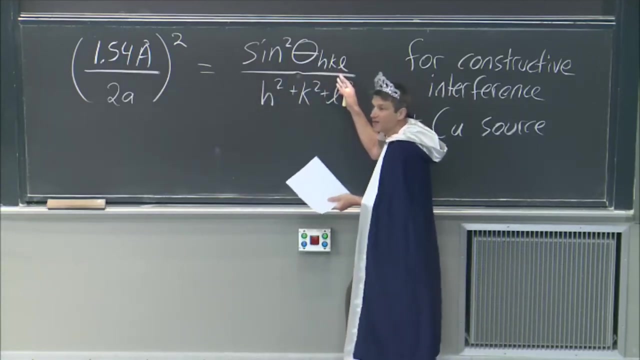 I'm going to measure these thetas where I get a signal. Remember, I'm going to now change theta So that I see where I get signals. right Now, those thetas divided by the plane, by the hkl that they are bouncing off of, must be a constant. 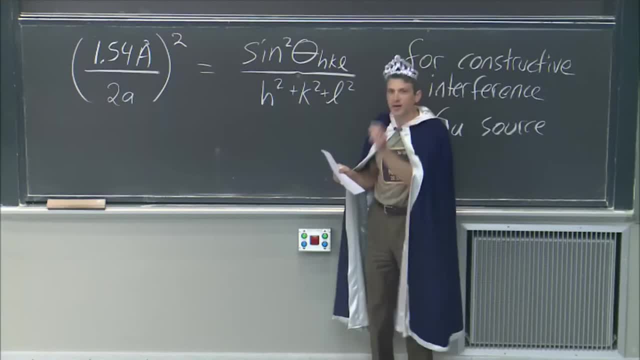 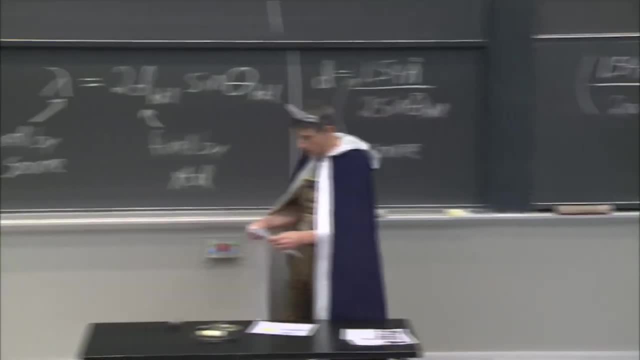 They must not change. That is at the heart of x-ray diffraction. That is at the heart of it, right? So we're going to do that with a specific example today and Friday. But before we do that, There's another thing that we can observe. 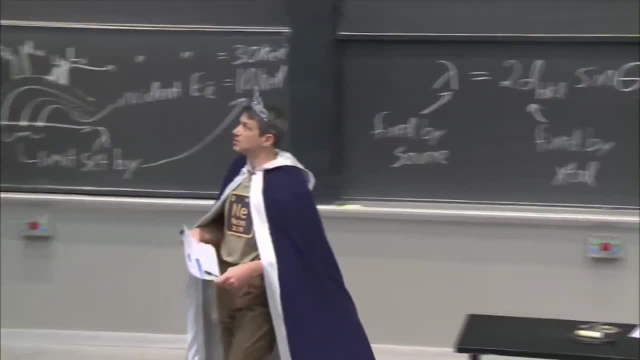 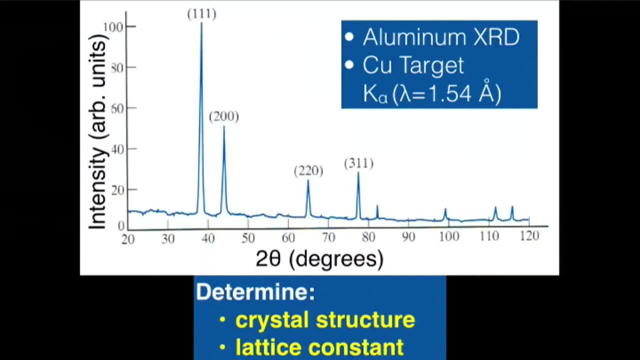 There's another thing that we can observe. Oh, this is what it would look like, So here it is right. So now I've changed. Now why do we do two theta? It's kind of historical, You plot x-ray diffraction spectra. 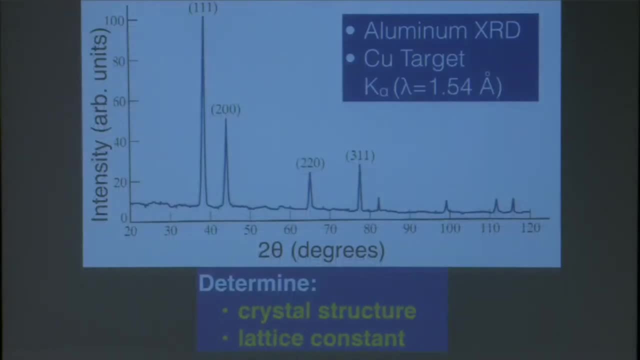 So this is an xrd right X-ray diffraction spectrum. This is the intensity of the peaks right And these are the peaks. This is a beautiful thing. I'm seeing a crystal here. I'm seeing a crystal And by Friday you will be seeing. 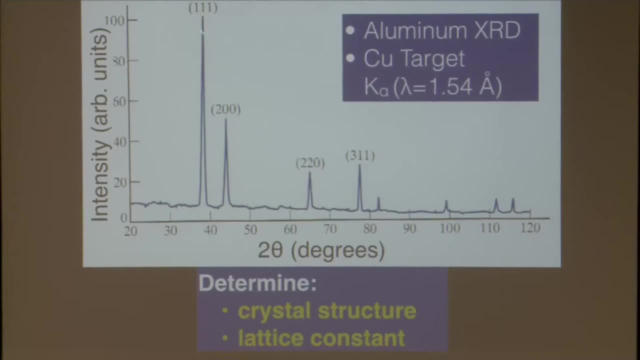 a crystal. Those aren't just peaks, Those are planes in a crystal. Those are planes in a crystal, Which tells me not only that I have these planes, but it tells me what crystal I have. That's not how we start. The way we start is we do these measurements. 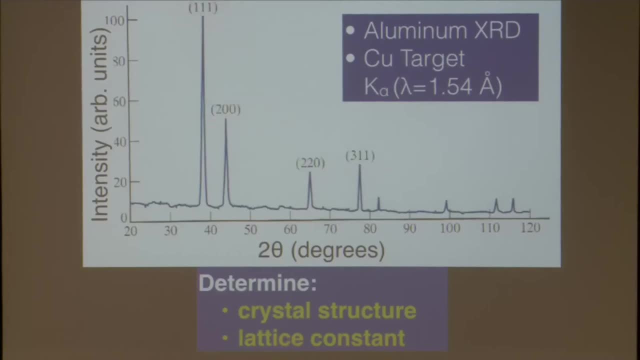 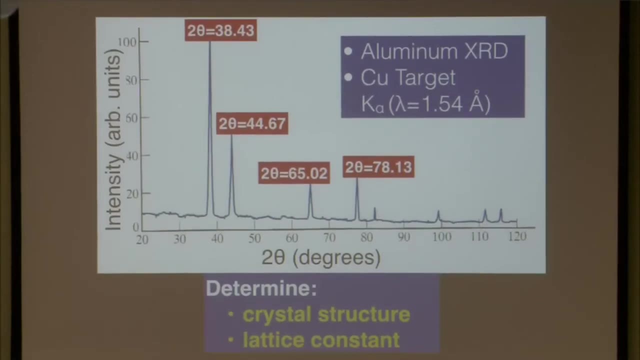 and we just read off angles. So we got to get from there to there, to crystal structure. So what I want to determine is the crystal structure and the lattice constant. That's my goal. What I have is a spectrum that looks like this, where all I've 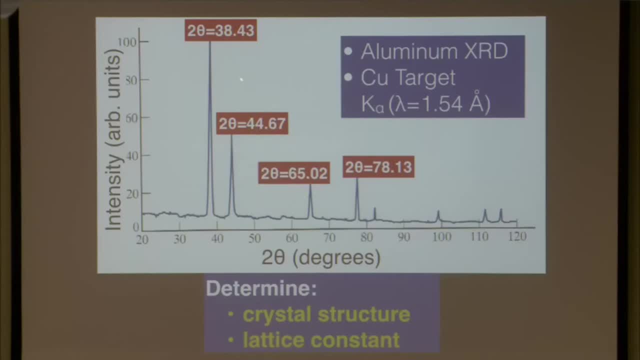 done here is: put these specific angles here And you have to be given: OK. so this is the aluminum xrd spectrum. So if you shine x-rays on aluminum, this is what you get, if you know also that those x-rays are from copper, which means that lambda is fixed right. 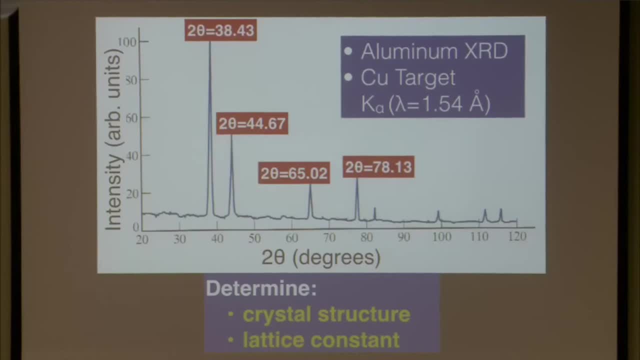 So this would be like the information you'd get to start: You'd be given this spectrum, You'd be given these peaks and you'd be given this information here. It's a copper target And from that we can determine the crystal structure. 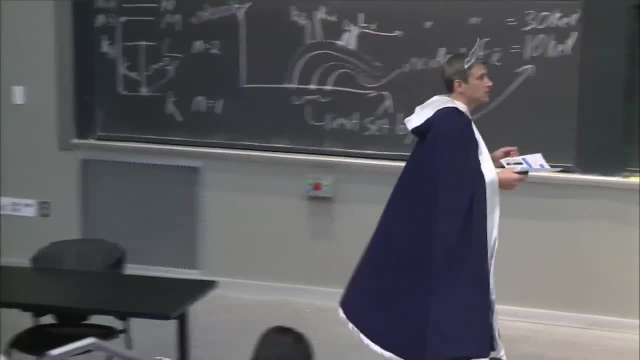 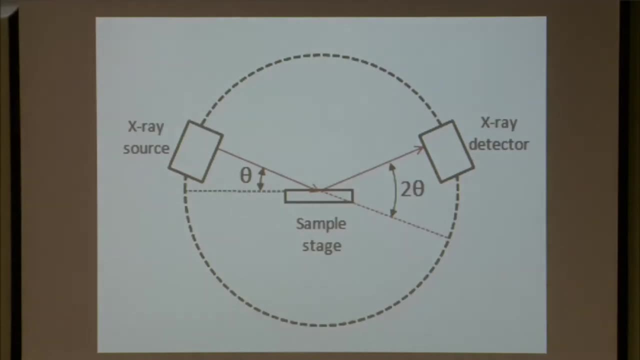 and the lattice constant. Now there's something: Oh, why do we do 2 theta? Well, it's historical. It could have been theta to make all those dividing by twos go away, But instead you can see that as I rotate this. 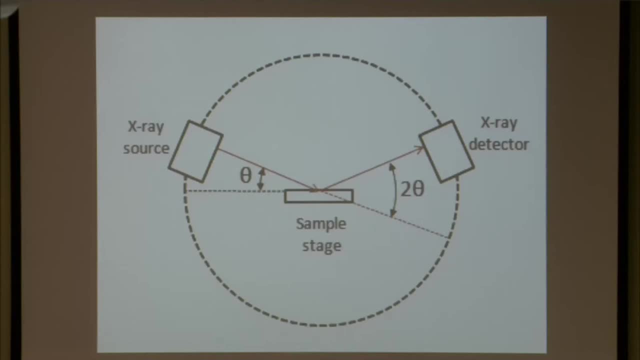 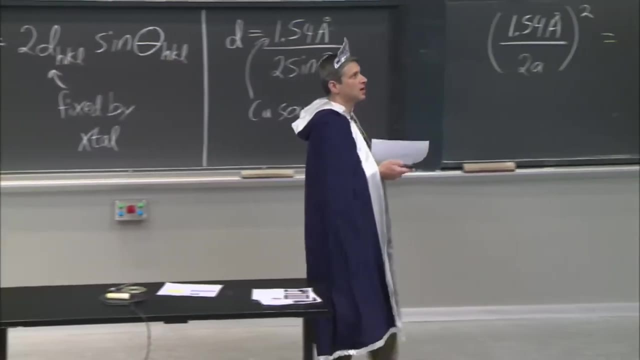 this changes by theta. The detector changes by 2 theta. So that's why x-ray spectra are given in 2 theta. There's no other real. There's no good reason for it, Even though in the Bragg condition it's not 2 theta. 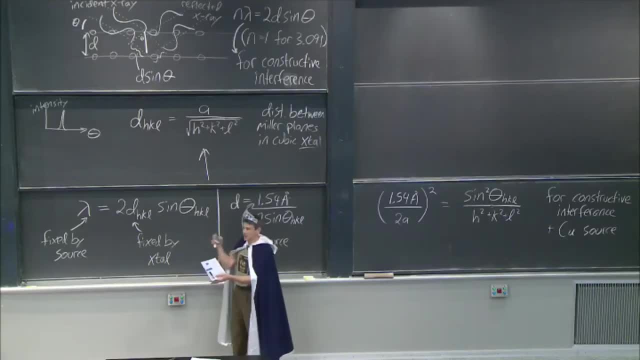 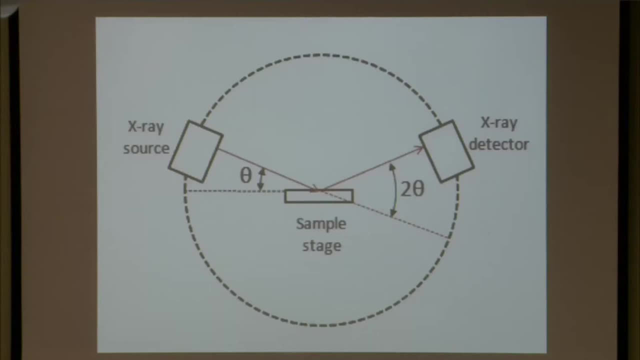 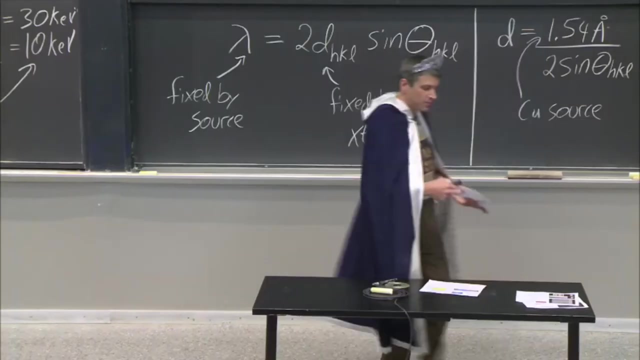 It's theta right. This comes from geometry of the planes And this just comes from historical setups and how you move the detector. So what's measured and plotted is the 2 theta. Now, before we go, before we do this transformation, where 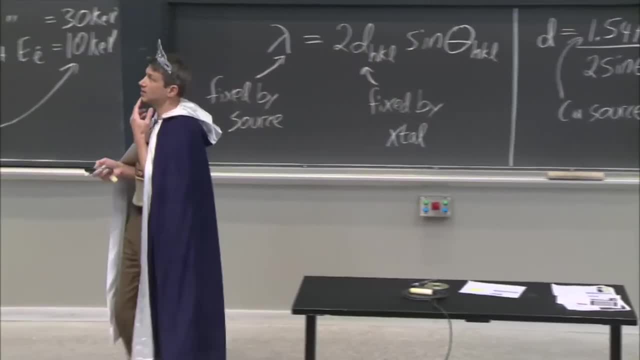 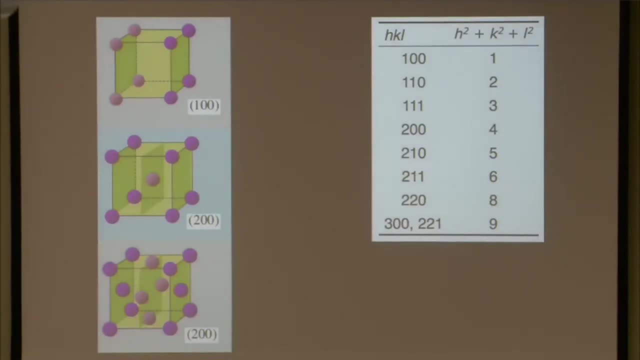 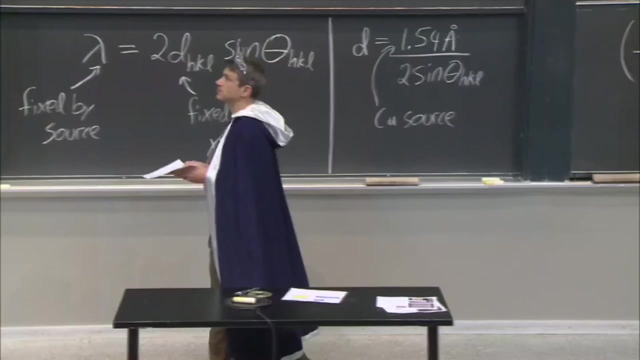 we take an x-ray spectrum like this and we get the information we want. there's one more thing, And that is: not all reflections are allowed. Not all reflections are allowed, And so let's talk about that, And then we'll come back to this spectrum. 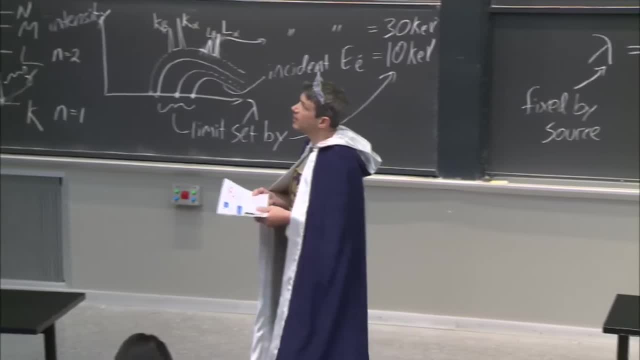 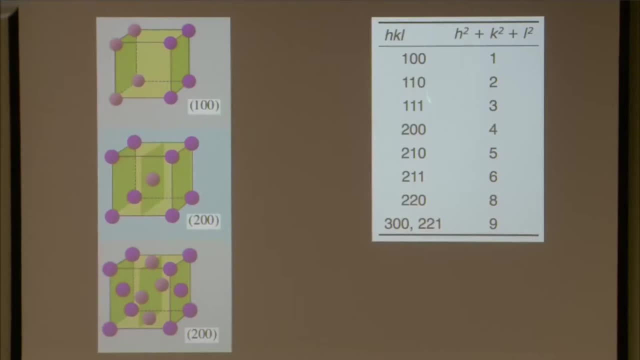 Now you can kind of understand this by looking at just a simple kind of comparison here. Simple comparison, If I take. so these are the hkls. Remember that's the hkl for a Miller plane. This is h squared plus k squared plus l squared. 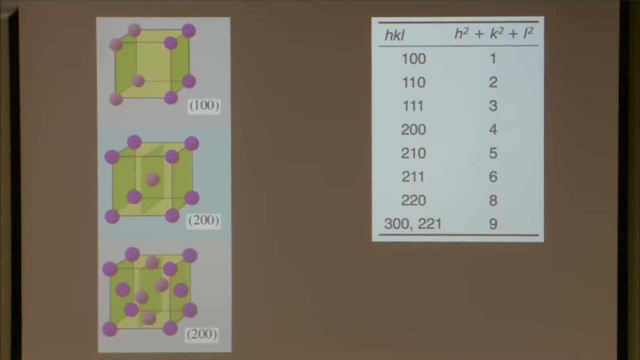 Why do we put that? Because we know we're going to need it There. it is right there, So we know we're going to need it. But if you look at the simple cubic, that simple cubic, any combination of hkl is OK. 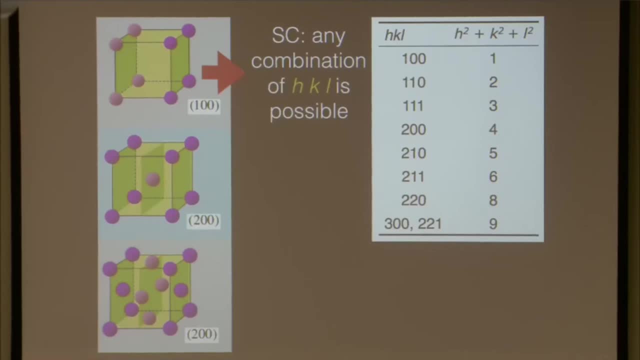 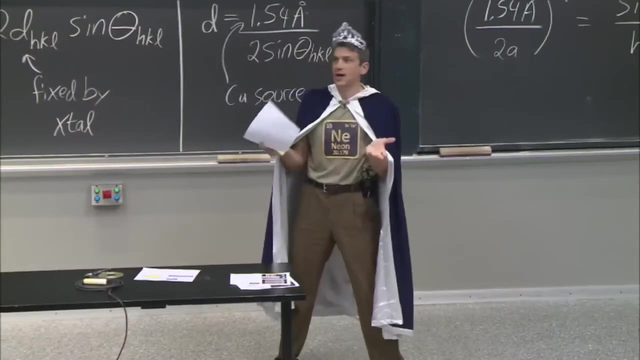 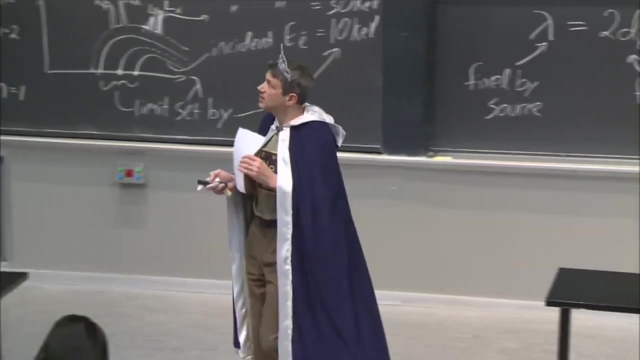 There is no combination that would give you interference along those planes stacking. You say, well, OK, yeah, what are you talking about? Why are you even bringing this up? Well, if you look at the other two crystal structures, you'll see what I mean. 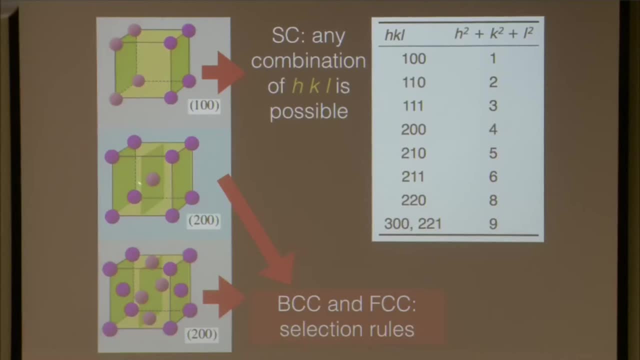 So now we have the case of BCC. When you see this, you see BCC and FCC, And what I'm showing you here isn't the 100 plane, It's the 200 plane. So this is the family- Remember the family- of 200 planes. 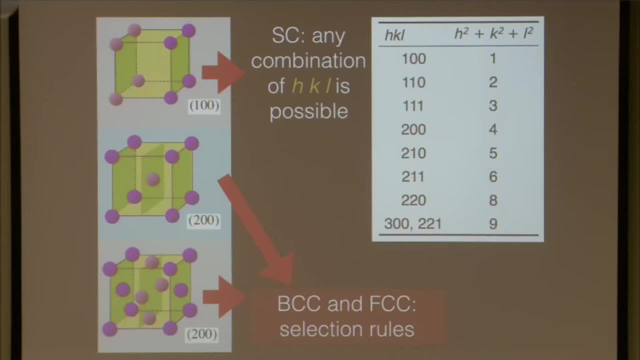 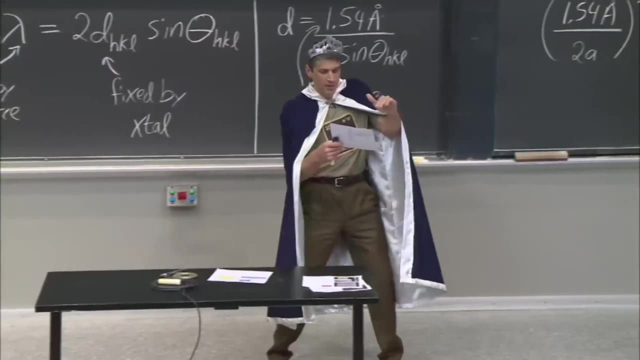 There they are. There, they are right. Oh, but now you see that what happens, and I have a picture here to show you. but I'll tell you first. The light comes in, so there's those squiggly x-rays, right? 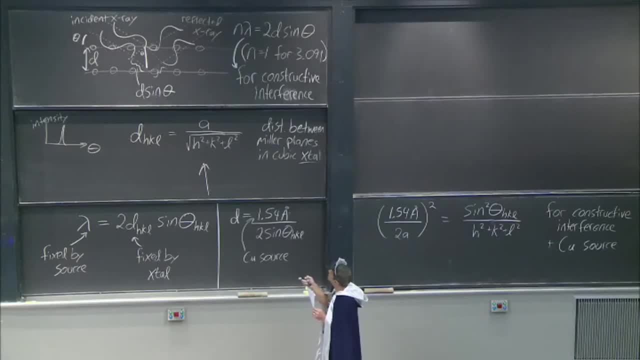 And it comes in, And there's the OK d, which depends on the lattice constant, is related to the lattice constant. But look, now there's another plane in between, There's another plane in between And in fact, with the 200 planes, 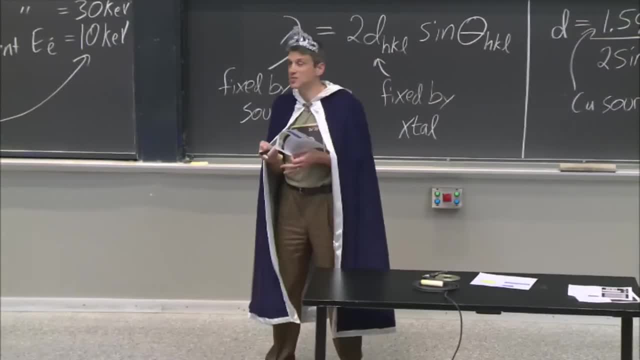 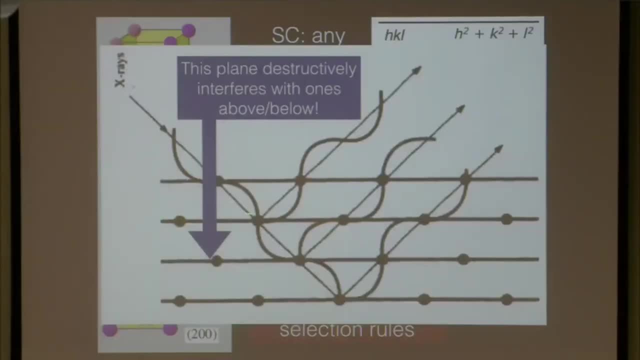 that plane in between exactly cancels out the constructive interference Here it is right. So there's what I would have had, right, If you want to think about this as the 100, 100, right, There's the 200.. 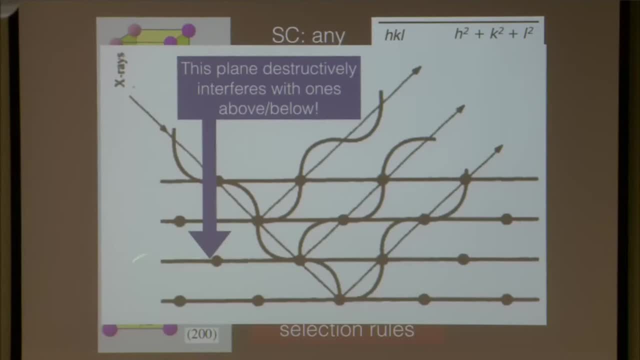 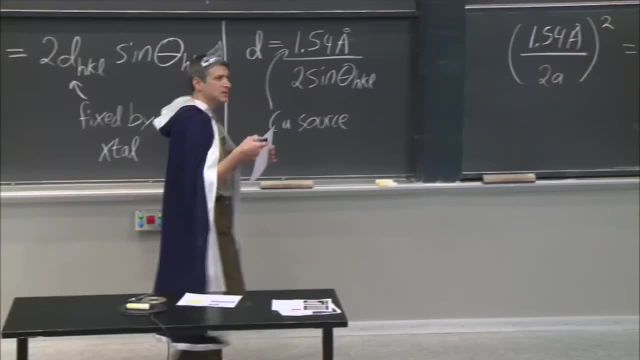 There's the 000s, OK, But notice, when I go from 100 to 200s, I add this plane in here, And because that plane has atoms in it, because that plane has atoms in it, it acts like a mirror. 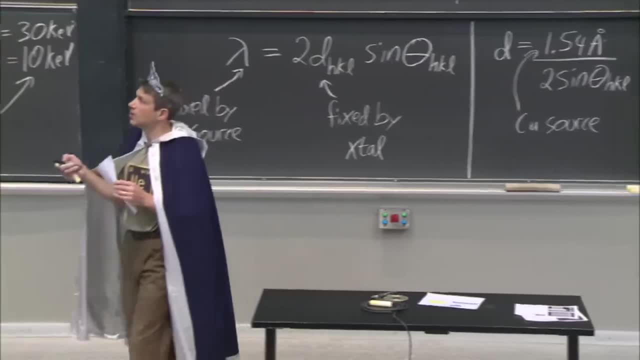 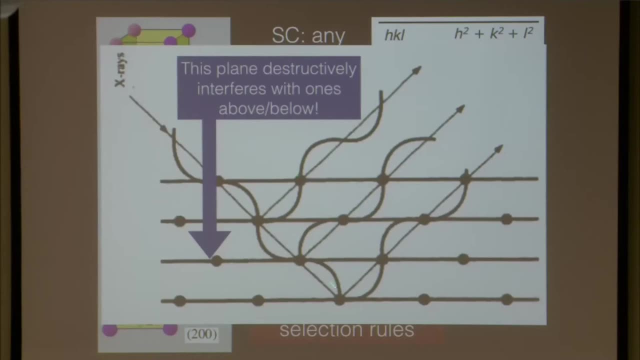 And it can also reflect. right, It can also reflect. And so what happens is, I would have had this nice there it is. there's the picture I drew. There's that first x-ray bouncing off. There's the second one bouncing off. 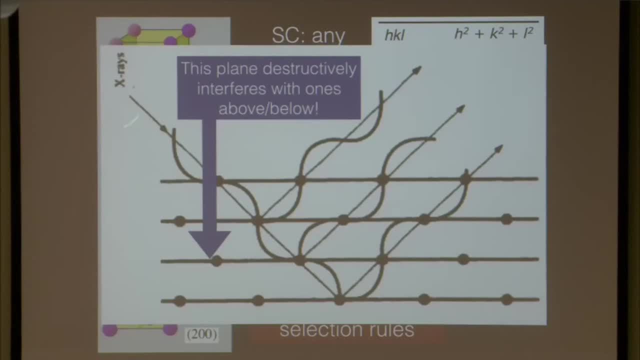 And those are nicely in phase. So I would see that. The angle that gave that to me, I'd see that in the detector. But now for BCC or FCC I've got something in the middle And that something in the middle is exactly canceling out. 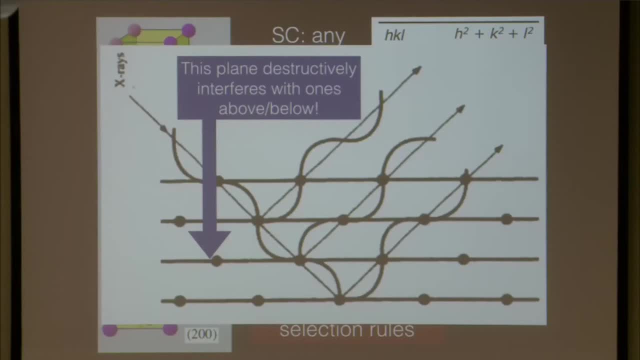 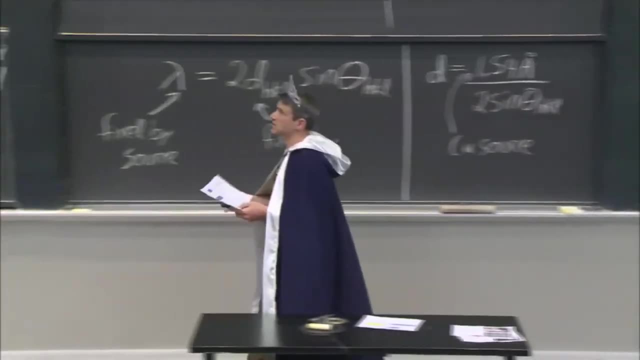 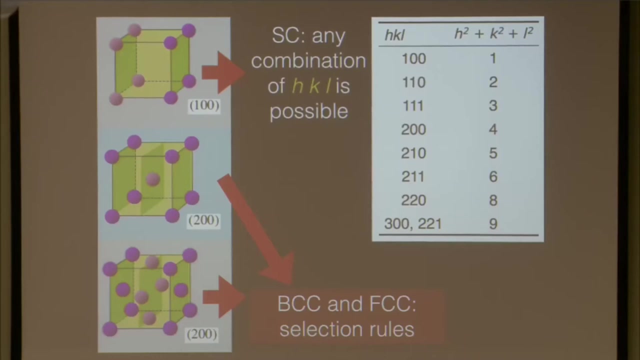 You see that. So now it cancels that out And in fact that's called forbidden. You won't see a signal, right? And so these are called selection rules. right, These are called selection rules. And for simple cubic you can see. there's nothing inside. 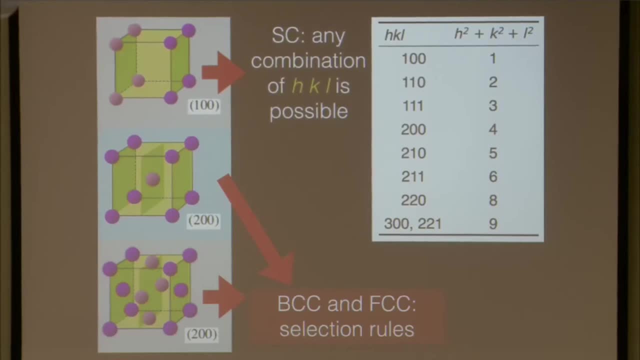 So there's nothing in this, There's nothing in this unit cell that could do this, So everything's allowed. Whether there's a plane in there or not, it doesn't matter. The selection rule is whether it's ever allowed. whether it's ever allowed. 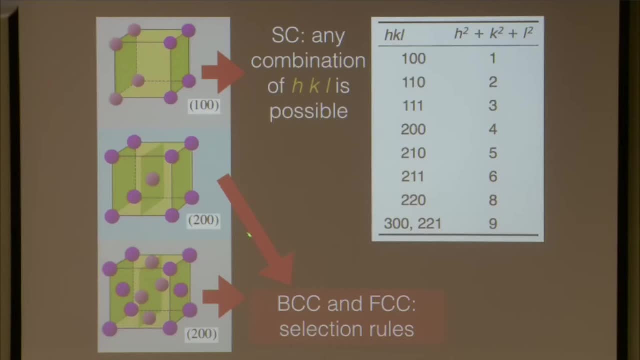 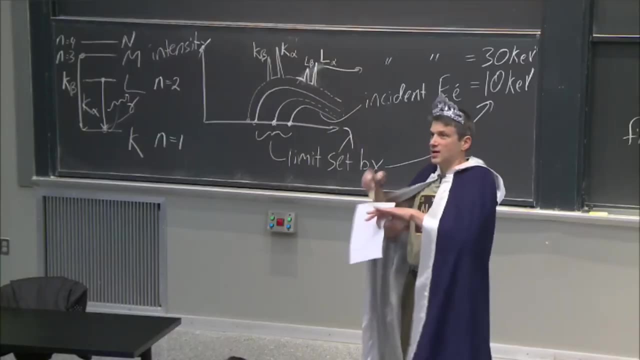 And for simple cubic everything's fine Because nothing would cancel out. But in here you see, in this 2-oh case you can see very clearly from that picture how it cancels out. But there's many other kinds of angles or planes. 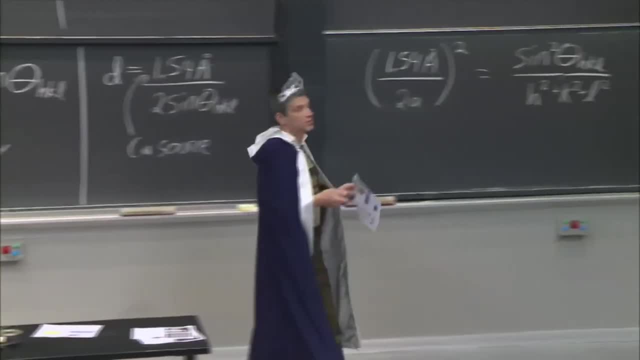 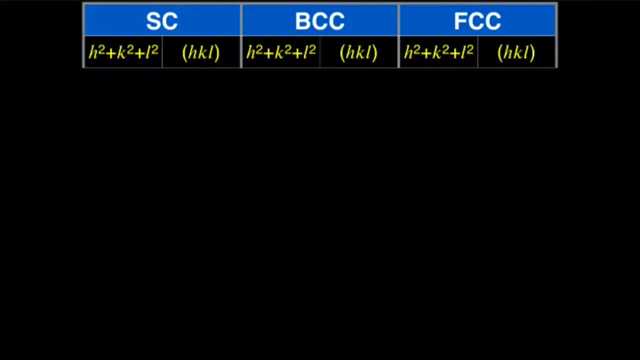 that might also do that Right. Give you what the selection rules are. We won't go through and derive them all, But let's see They are actually quite simple, And so I'm going to write them down, Right? So if we look at allowed reflections, 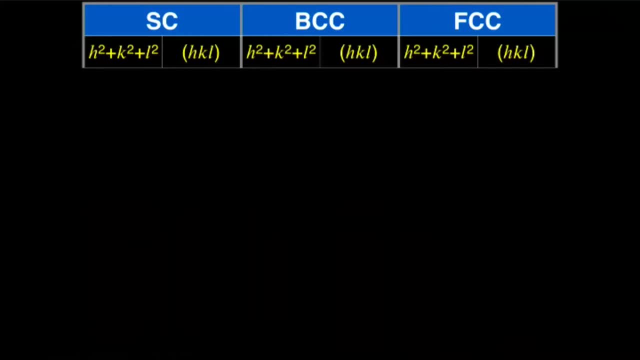 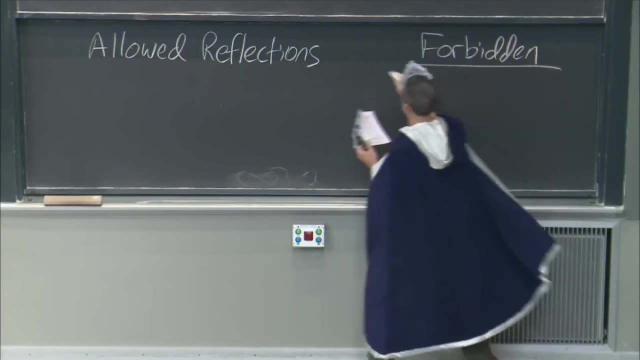 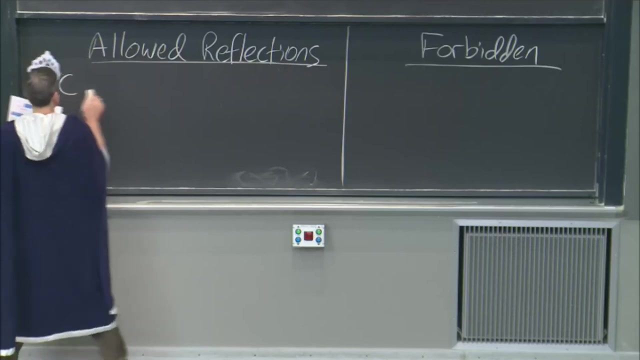 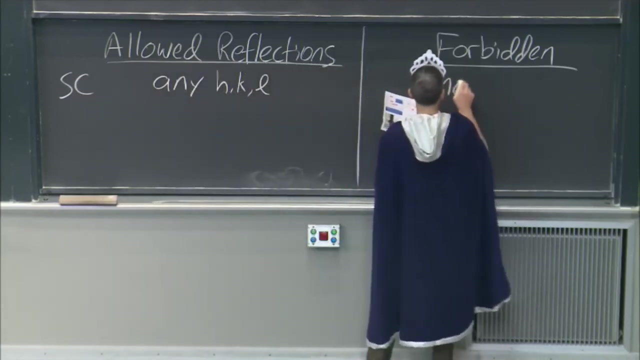 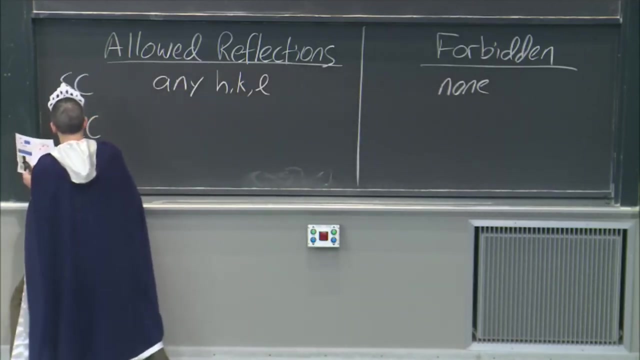 and then we look at forbidden Reflections. So this is what the selection rules tell us. OK, So if it's simple cubic, then it's any h, k and l And there's no forbidden reflections. But if we go through BCC and FCC, then what we find 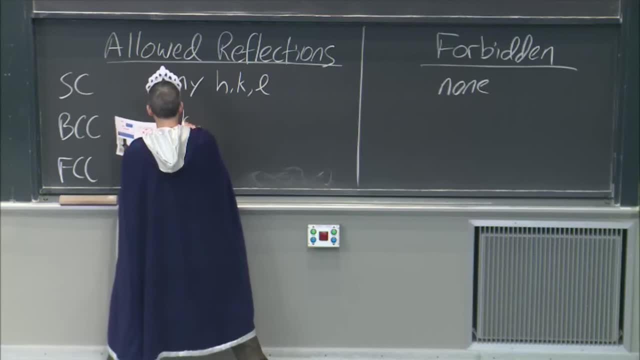 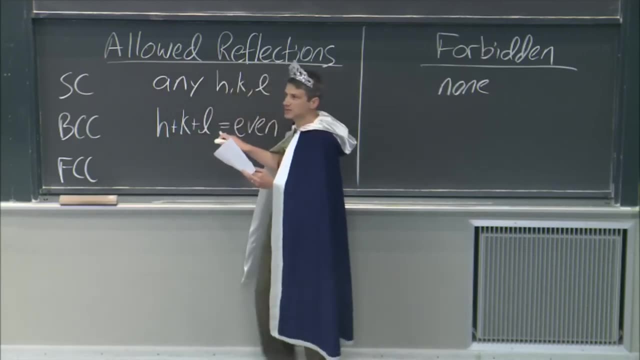 is that for BCC, the selection rule is that h plus k plus l equals. even If that is even, and we won't derive these, but it comes from the same very simple picture I just showed you. If something is in there that can cancel out, 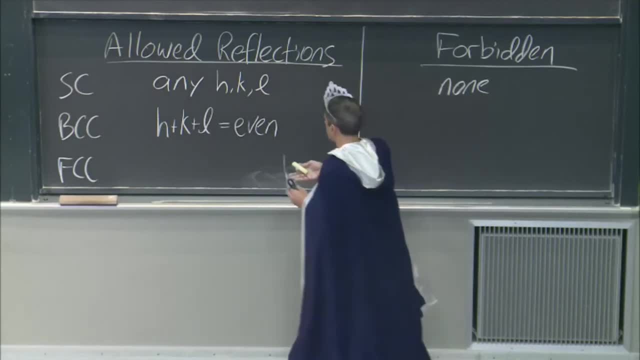 the constructive interference it's going to be forbidden. Otherwise it can constructively interfere, And that's what this tells us. For BCC, it turns out to be h plus k plus l, And so here, what's forbidden for BCC is h plus k plus l. 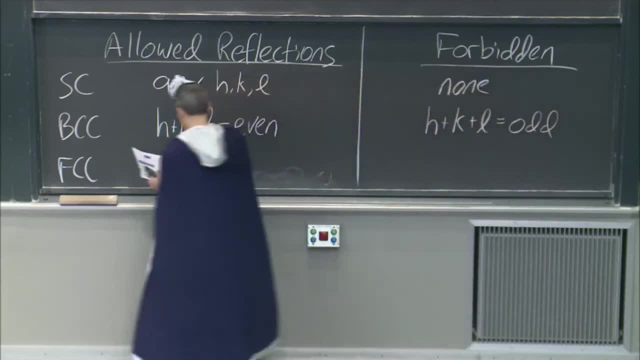 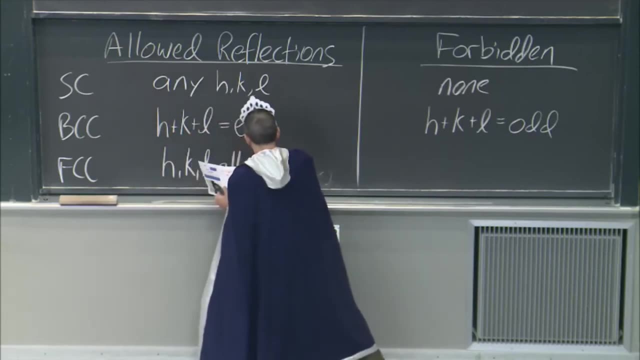 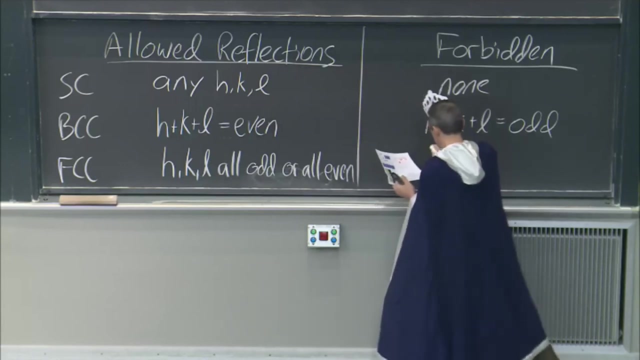 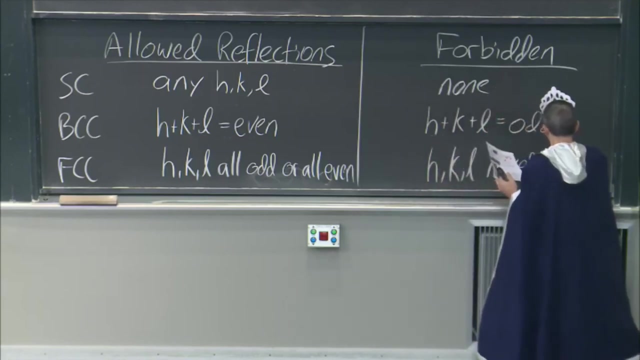 is 0.. It's odd And for FCC it's h k l- all odd or all even Or all even, And the forbidden FCC is h k l- mixed odd even. These are the selection rules. 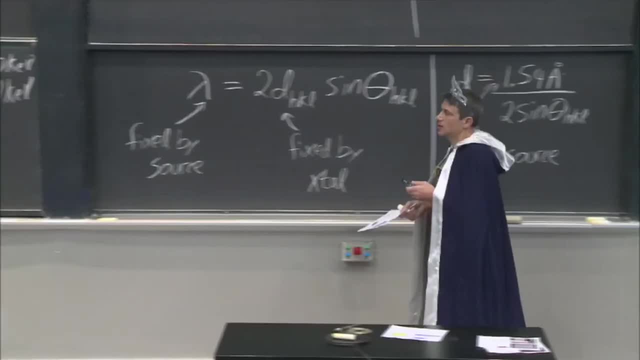 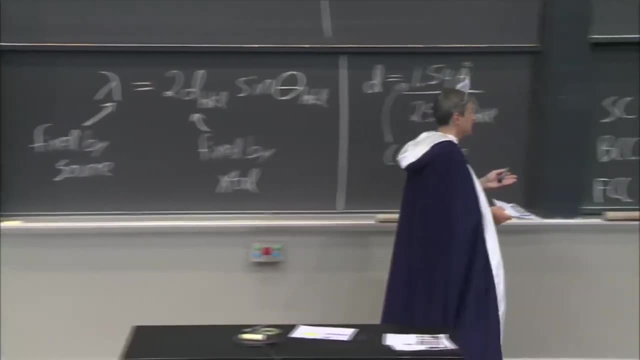 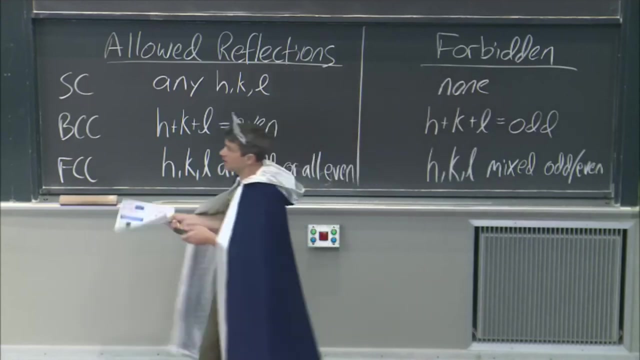 OK, All right. So if I were to give you the planes that you see, then, right away from an x-ray spectrum, you could just use these selection rules right away to know something, to know something about it. And if you work this out and you look at, OK. 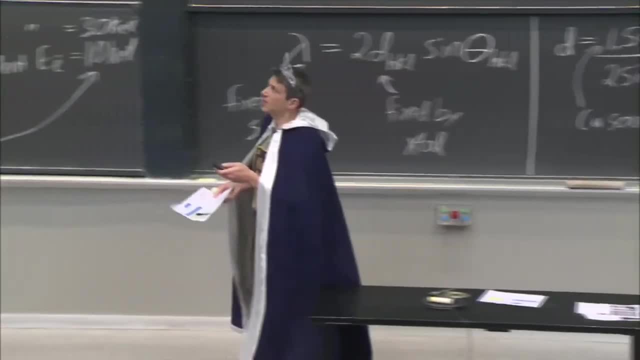 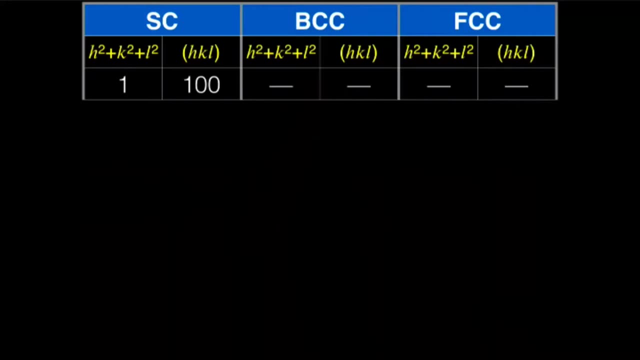 so we have simple cubic There, it is OK. so h squared plus k squared plus 1, 100, BCC, FCC, you're not going to see it. That doesn't mean That doesn't mean that there's no 100 plane in those crystals. 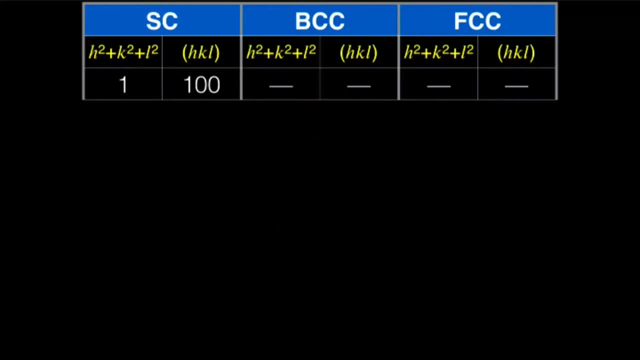 It just means that if you shine x-rays on it, you will not see it, Right, You will not see it. OK, so the 110, though now here. OK, so we see our- oh, by the way, mixed, even odd, right. 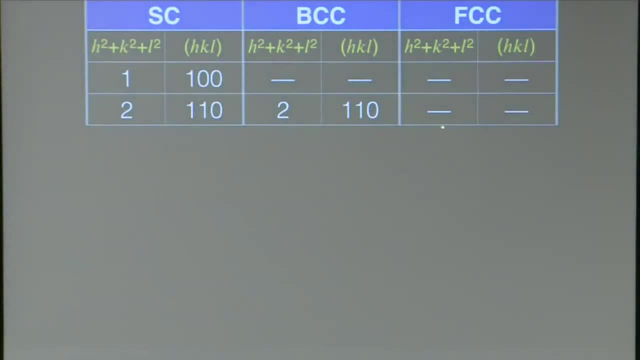 And it adds to odd. That's why neither one of these works. Here we go. Adds to even BCC: OK, but it's still mixed. even odd Won't be FCC right. 3, right, It's not mixed. 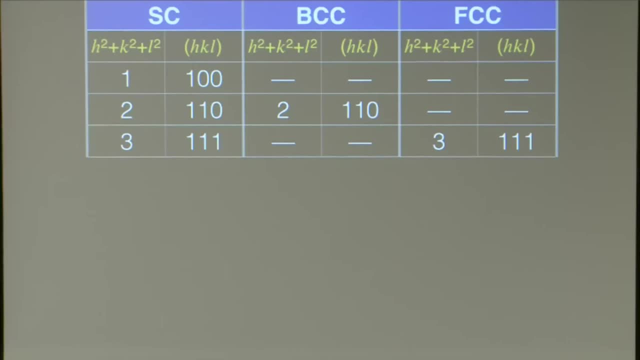 So it can be an allowable reflection for FCC but not for BCC, Because if you add them up it's odd and so forth and so forth. And look at, 7 doesn't exist, because you can't do it. 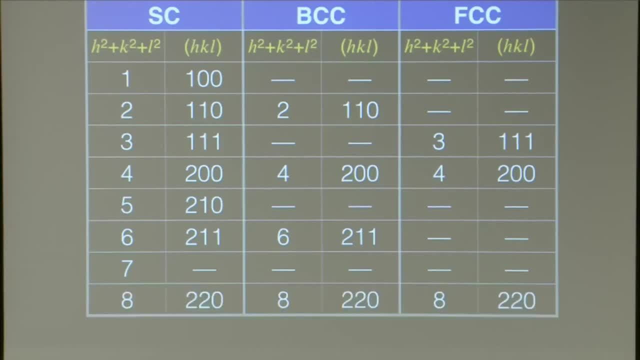 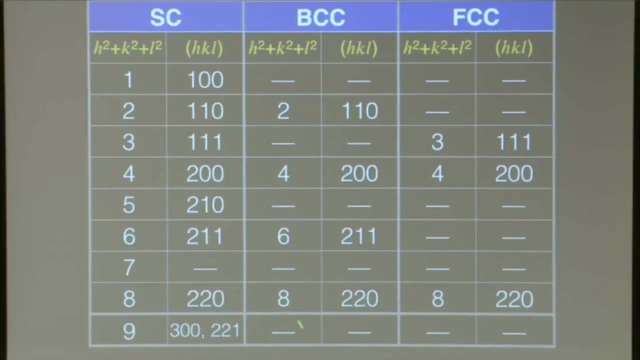 No matter how hard you try, you can't get 7. That's OK. And there's 8 and 9 and so forth, So 9 also. so here it's allowed, but it's not allowed in either of these, because you can't get. 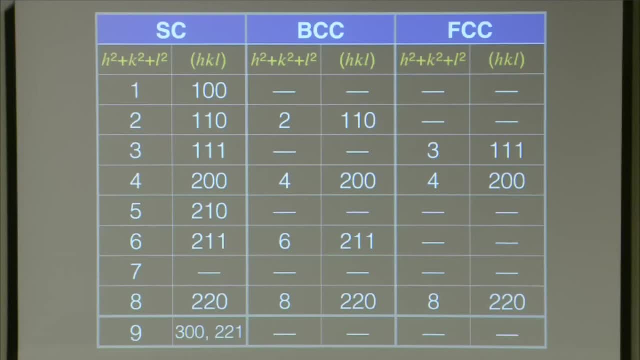 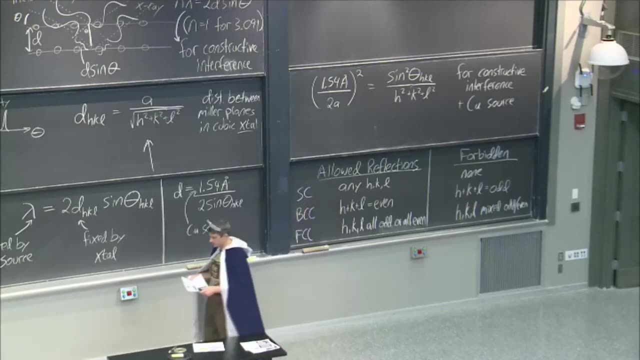 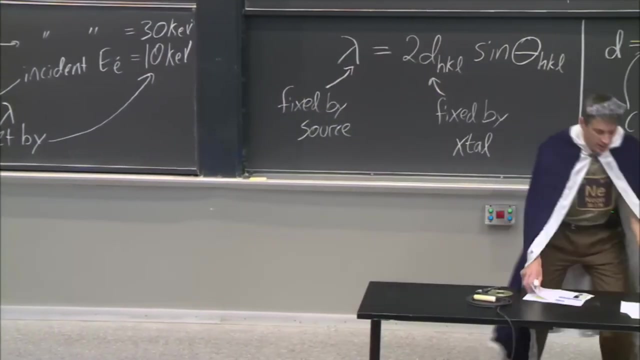 you can't get the. you know you can't get either of these to be satisfied. OK, This is what selection rules give us, And it comes again from simple, oh. OK, well, that's another thing. As it's simple, I have to tell you something. 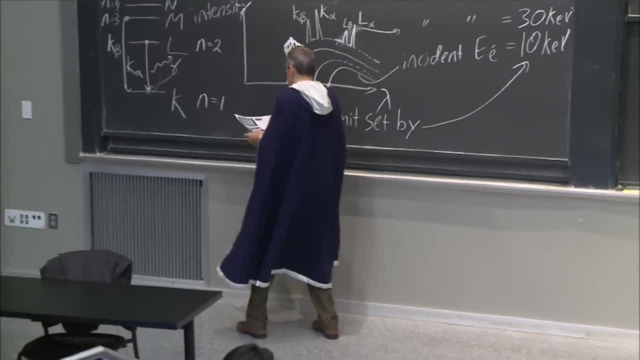 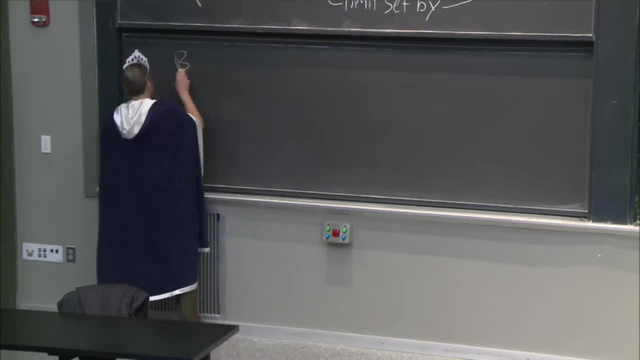 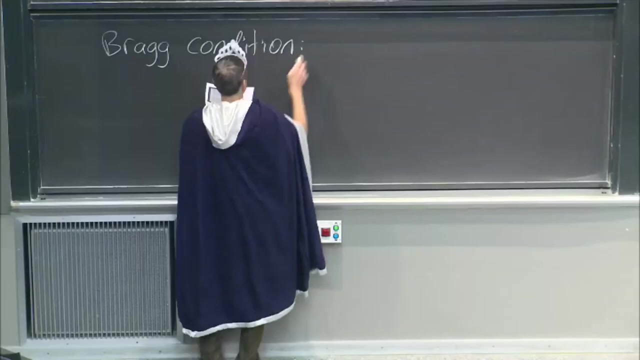 Because the Bragg condition, it relies on an assumption. That's mostly true, but you know the Bragg condition. the Bragg condition requires that the reflection is independent. Some of you may be thinking: did I, did I draw that onto the atom? 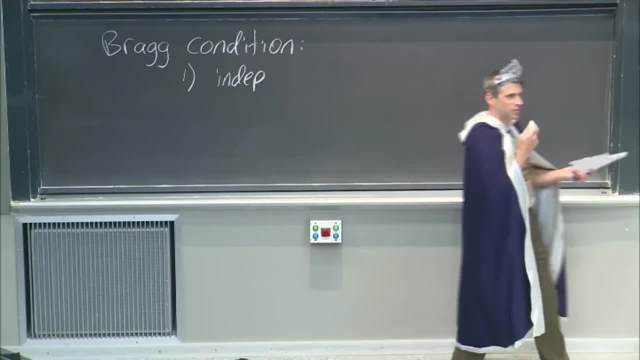 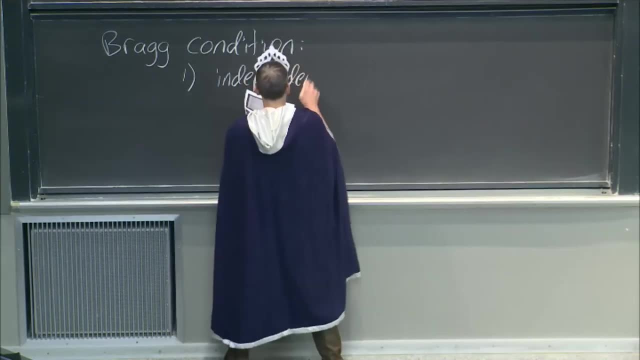 Or did I draw it in between the atoms? Where did that thing reflect? It doesn't have to reflect off an atom. We're not going there With the Bragg condition. it's independent, independent, OK, of the atoms. So the atom positions in a plane. 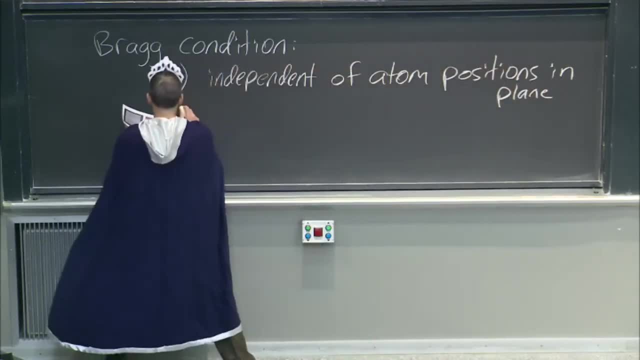 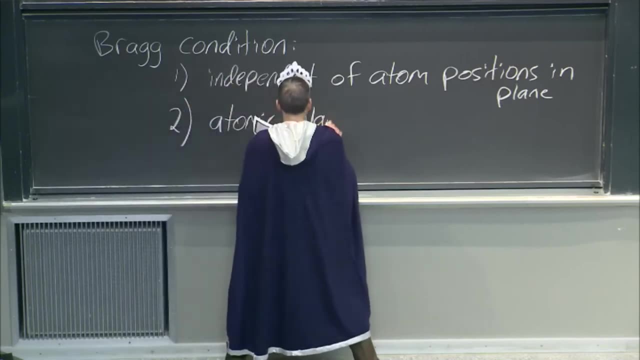 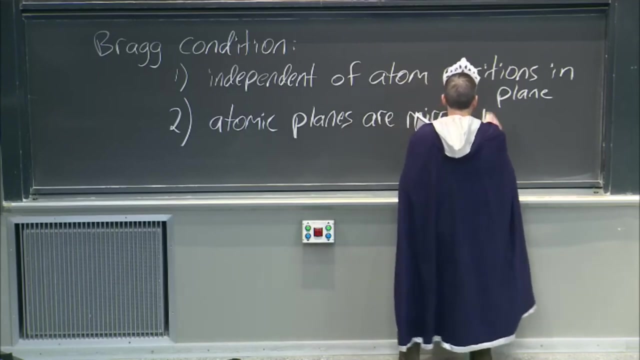 And the second thing, which is what I've been sort of alluding to, is that the atomic planes are mirror-like, Are mirror-like. I mean, this is sort of an obvious assumption, since I've been assuming they've been mirrors. 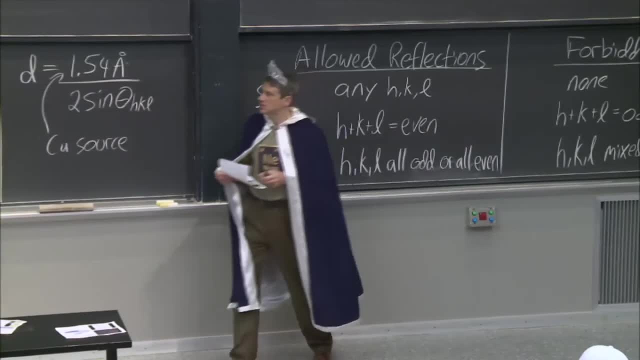 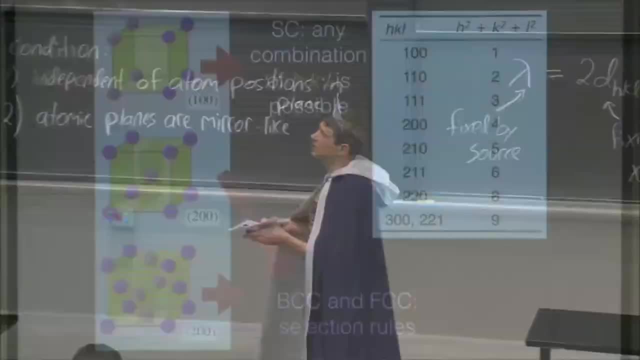 But you know it's not. so if you start thinking about atom position then you might go back to that- you know that selection rule picture and say, oh, wait a second why, you know, does it always have to hit the atom there? 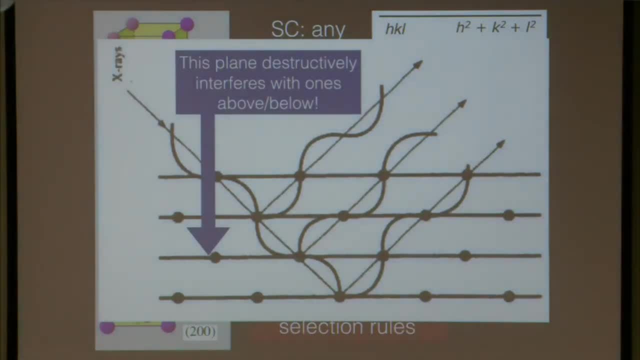 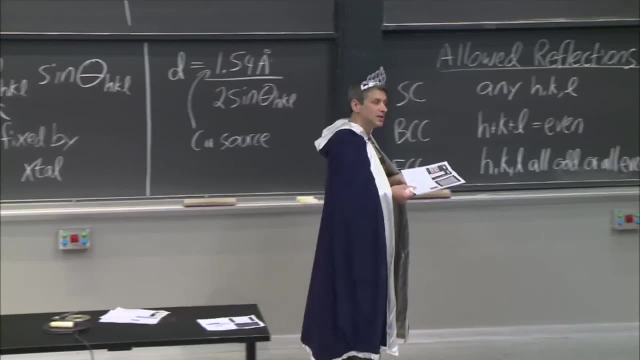 Or what if this one was over? or something like that. No, no, we assume it's just one continuous plane If there are atoms in it. if there are atoms in it, right. if there's no atom in it, then it's not a reflective plane. 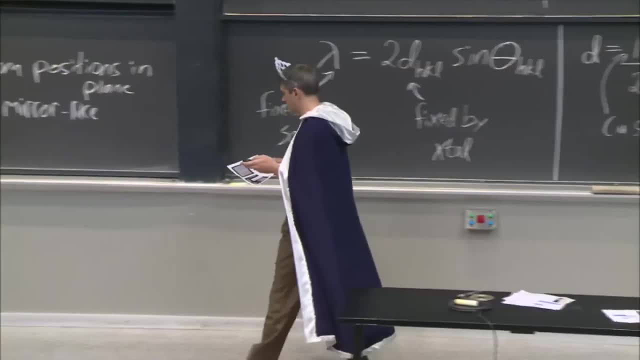 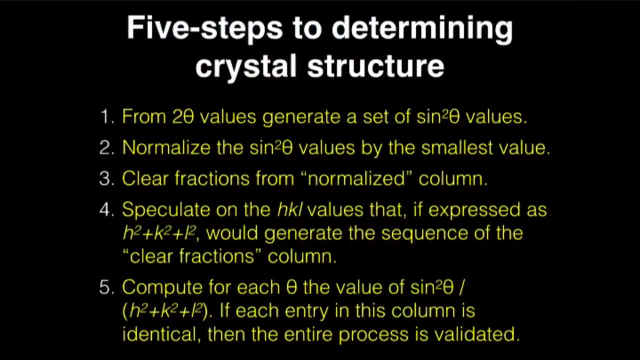 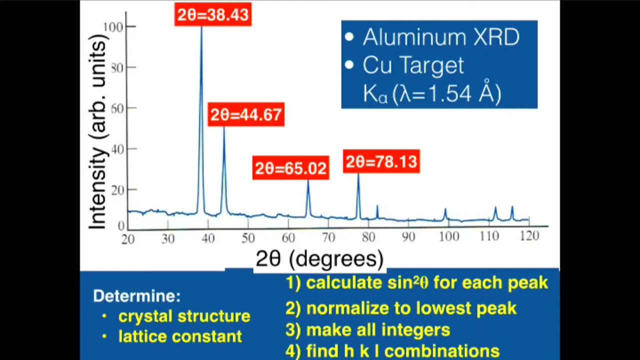 OK, But it's continuous. It's continuous in the assumption of the Bragg condition. OK, now we go back to our picture. OK, so what we want to do is again our goal, Our goal. should we choose? should we choose? 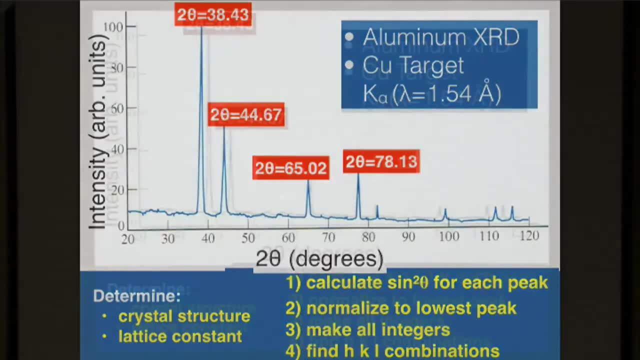 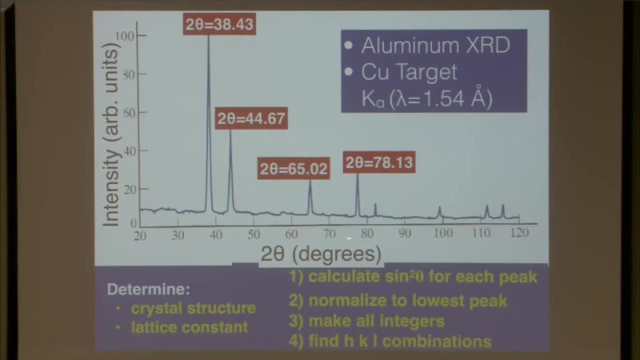 our goal is to go from this spectrum, knowing this information right- it's a copper target- and being able to read off the peaks. our goal is to do: determine the crystal structure and the lattice constant. That's our goal, And let me just write this again: 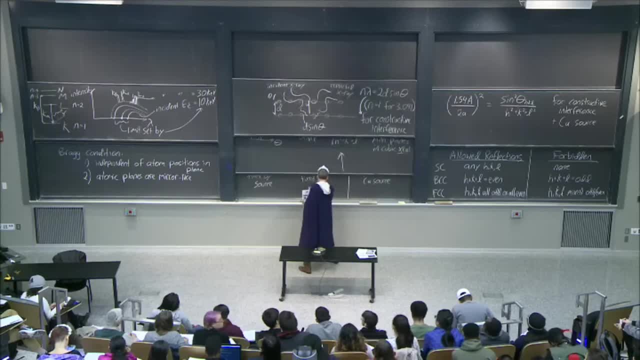 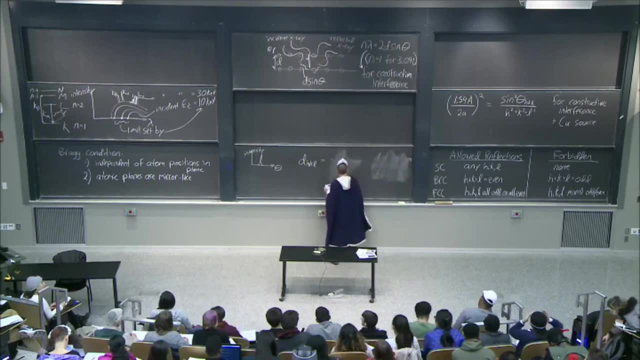 because it's extremely important. So I'm going to- maybe I'll keep that one. I'm going to erase this and put it right in the middle, because this is what drives XRD. This is what drives XRD. OK, which is that our goal? 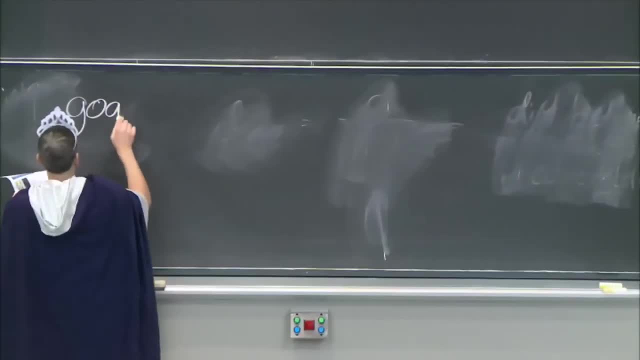 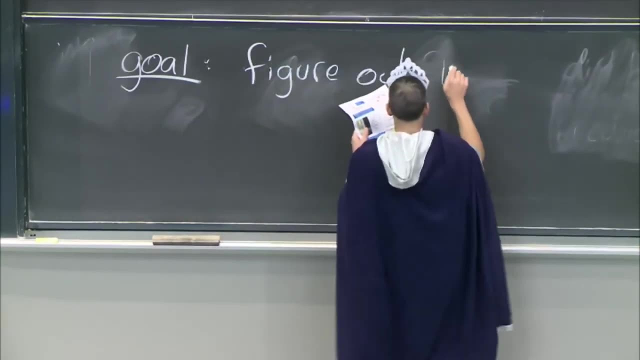 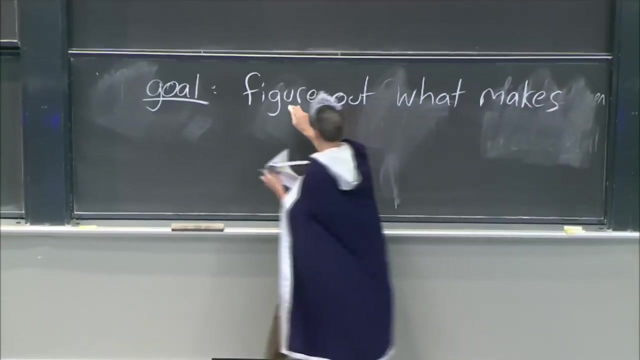 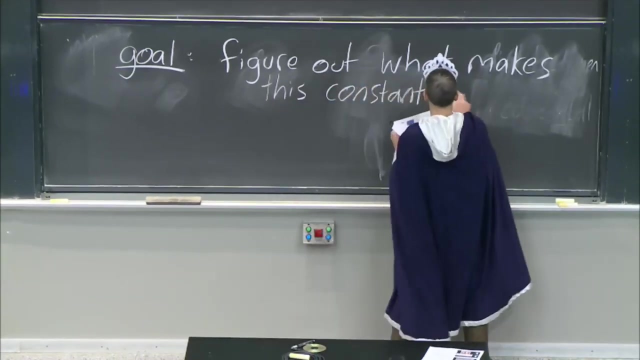 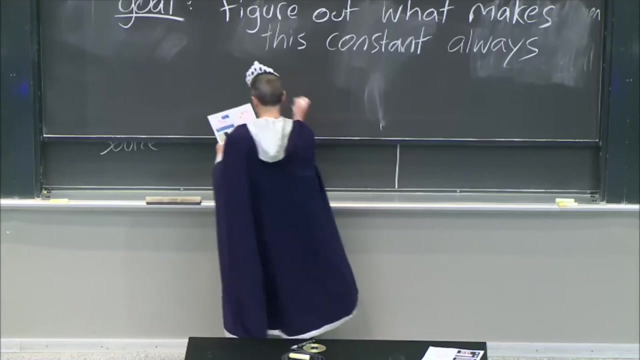 is figure out what makes this constant always constant. Now you say, what is this constant always? OK, this is the expression Which I'm going to write again, just for So what I have if it's a copper source. 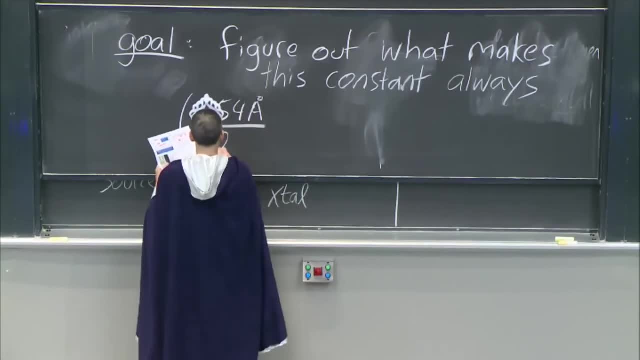 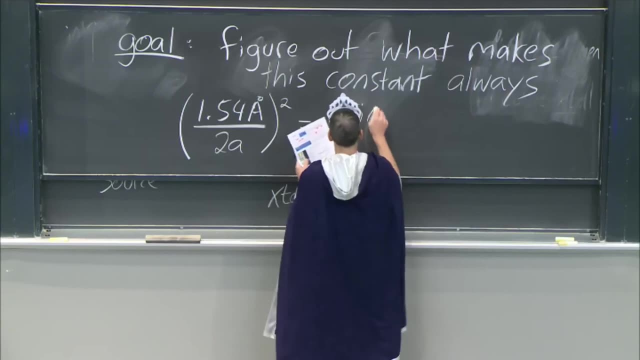 is 1.54 angstroms divided by 2A squared, That's a constant Gesundheit. That equals sine squared of the theta for some plane divided by H squared plus K squared plus L squared. So I'm just kind of repeating what I've said. 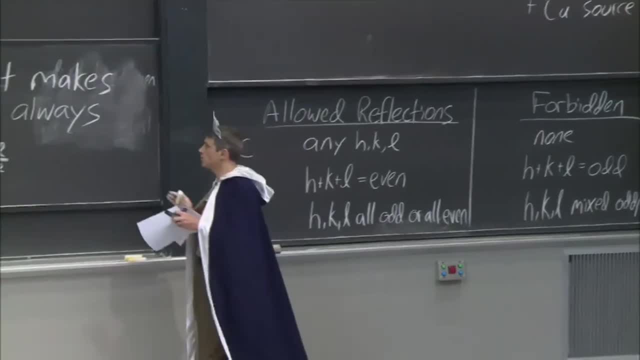 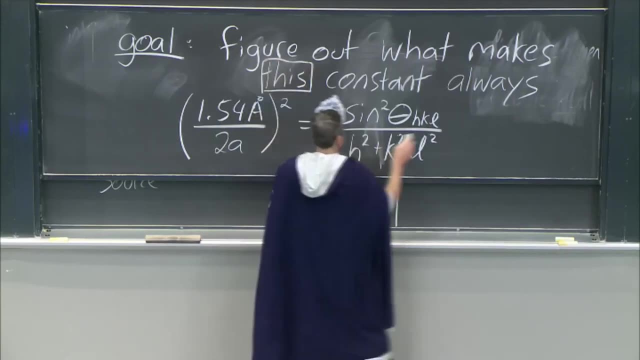 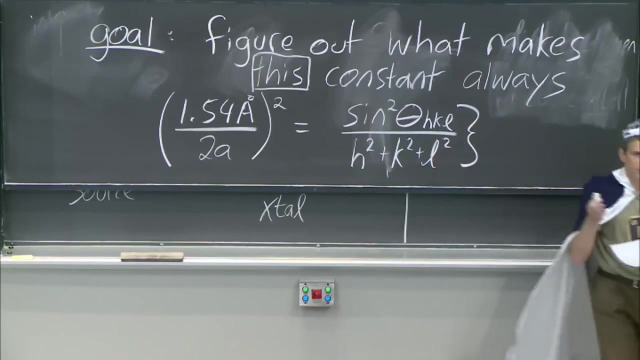 and what I've written elsewhere, But that is really it. That is what we do in X-ray diffraction. What makes this Well? by this, what I mean is this term on the right. How do I make sure that this never changes its value? 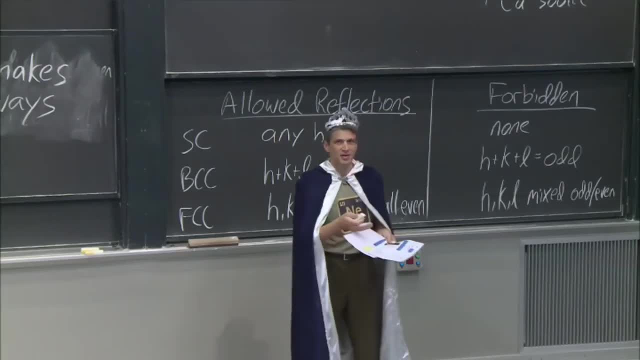 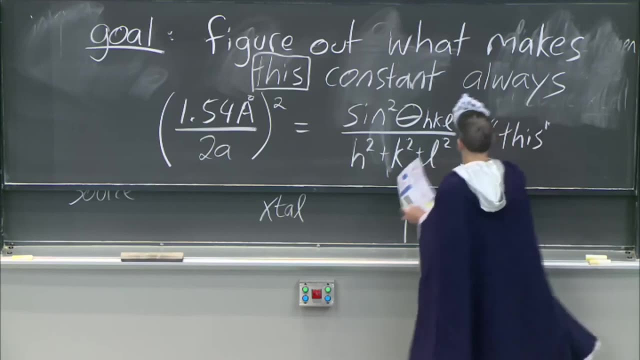 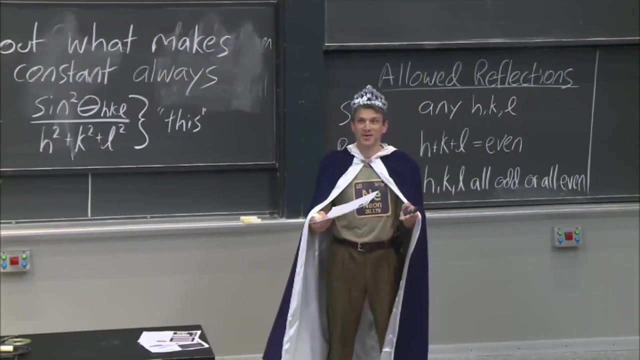 Because the thing on the left never changes its value, right, And just making sure that you've got that concept. That is this: Oh yeah, OK, And it turns out. It turns out. I got a recipe for you to follow to do this. 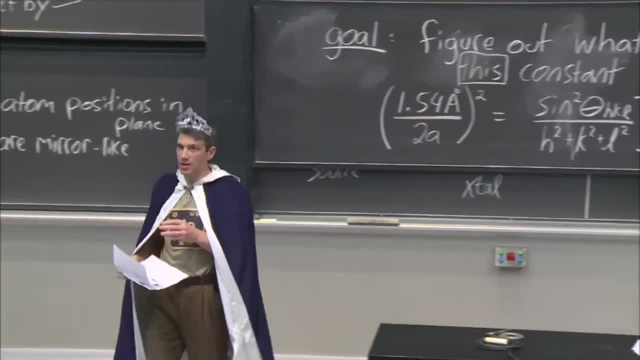 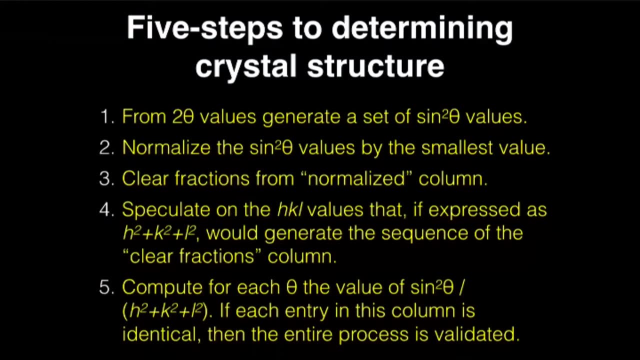 And it's on the previous slide, And so we'll start thinking about it now And we've got five more minutes, And then on Friday we will finish this and then talk about what to do with those continuous X-rays. So what do I do? 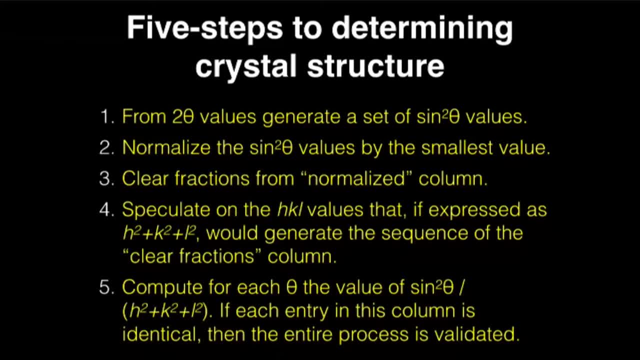 Well, the way you do this is systematically Gesundheit. The way you do this is systematically And the first thing you do is you take off the two theta values that generate a set of sine squared values. So the X-ray spectrum measures two theta. 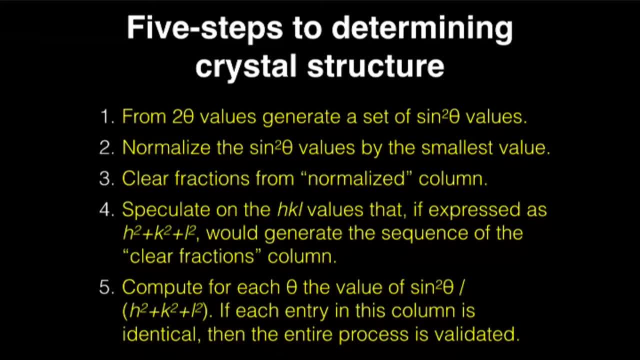 But we know from here that I need sine squared, So I'm going to write down the sine squared values. So that's a first step, So, OK, Good. So for the first one, I've got the first peak, So I would start to. 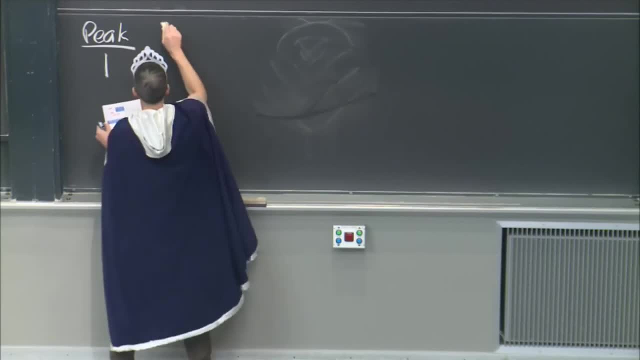 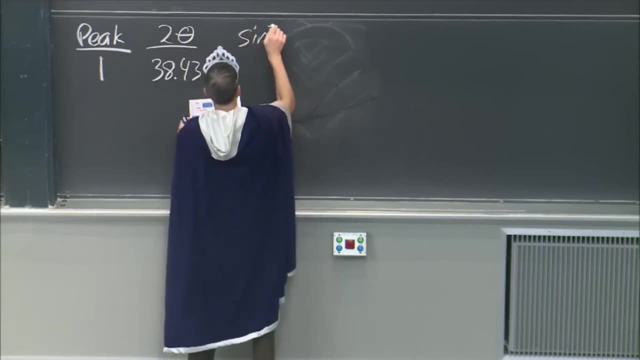 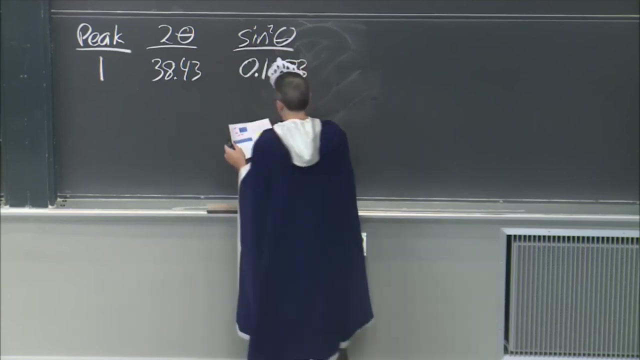 I'm going to log my data right. The first peak and the two theta is 38.43.. And the sine squared theta is- and I'm just going to do that math- 0.1083.. OK, OK, good. 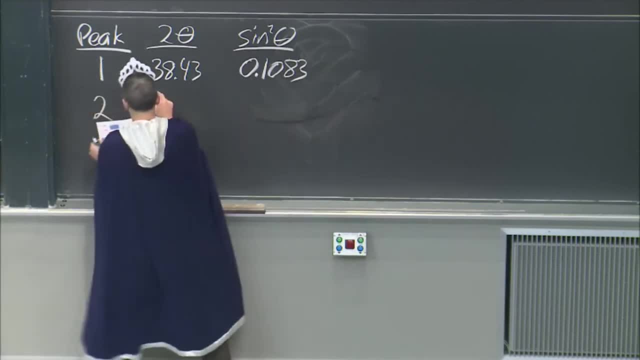 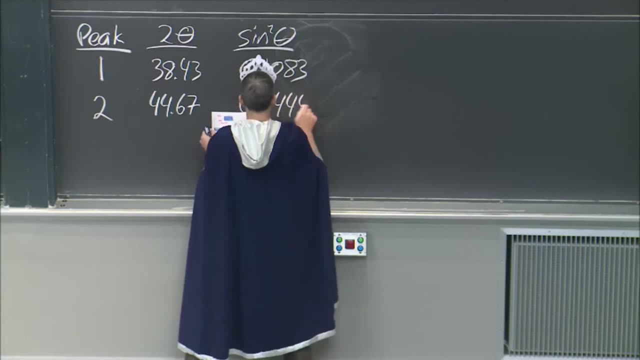 And the next one. the next peak is 44.67.. And the sine squared of that is 0.1444.. And so on. So you read off all the peaks and you make those columns. OK, so I've gone through one. 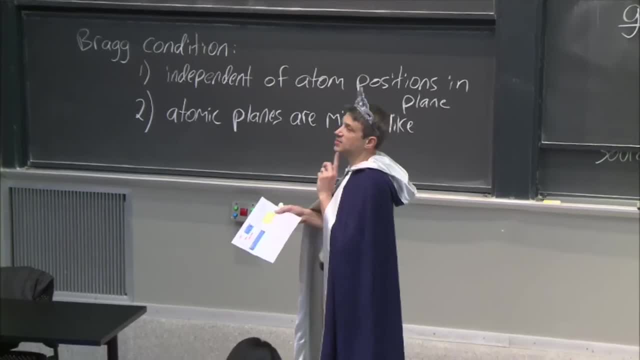 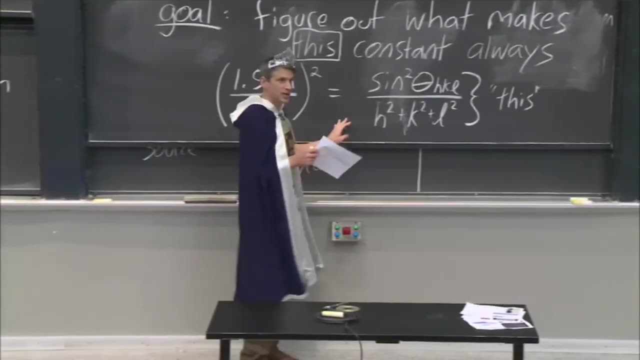 Now the second one: normalize the sine squared theta values by the smallest value. Right, OK, You say, why am I doing that? Trust me, This will achieve our goal. This will get us there. This is a nice, simple recipe to achieve our goal. 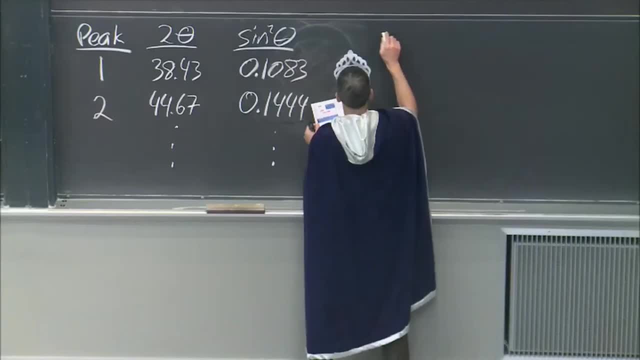 So the next column would simply be sine squared theta divided by sine squared theta. OK, Well, I ran out of room there, But that's going to be obviously 1., And this would be 1.333.. And so on. 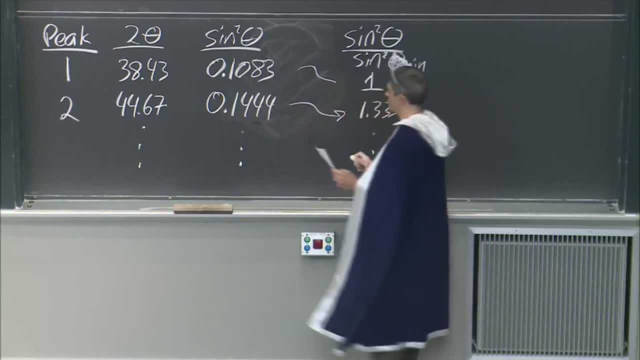 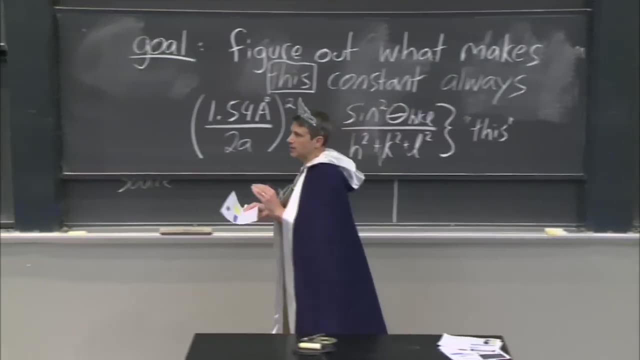 So that's the next one. So I'm just setting the top row to 1.. OK, I'm setting the top row to 1.. So that's OK. Good, Now I'm going to clear fractions. So I've normalized. 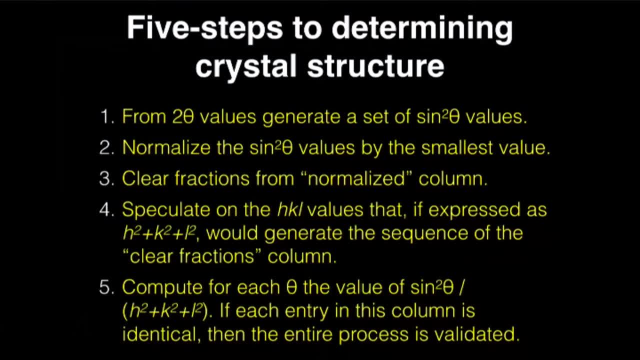 And now I'm going to clear fractions. So I'm going to clear fractions, So I'm going to clear fractions. And if I do that, if I clear fractions, well you say, what does clearing fractions mean? It means just what it implies. 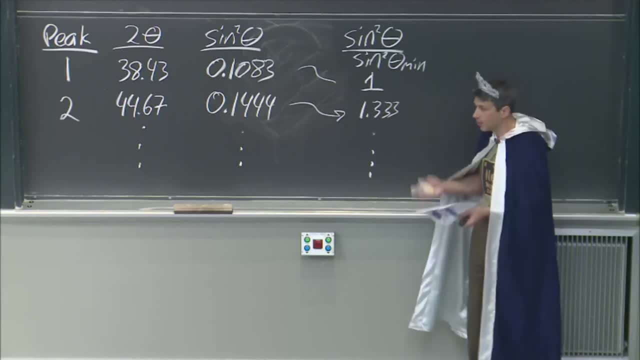 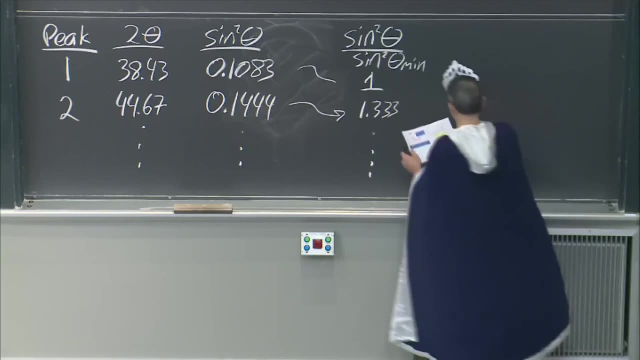 I don't want fractions anymore, So I'm going to multiply. It means I just need to multiply the whole set of numbers by something that gets rid of the fractions, And it turns out that in this case it is 3.. So 3 times sine squared theta. 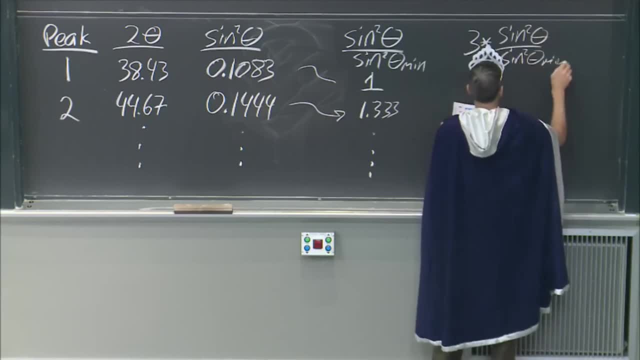 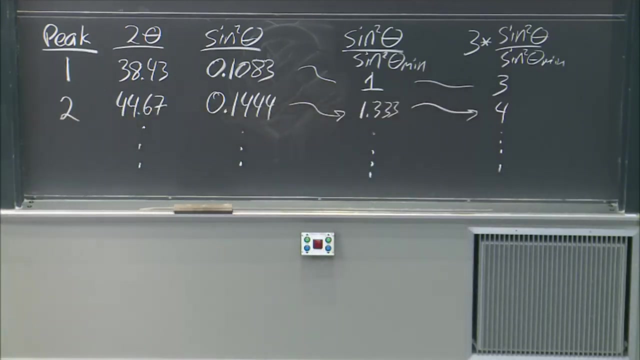 Over sine squared theta min, And that is going to be 3. And that is going to be 4. And so on. OK, So this is the problem Now. we're almost there. We're almost there And we're not going to finish today. 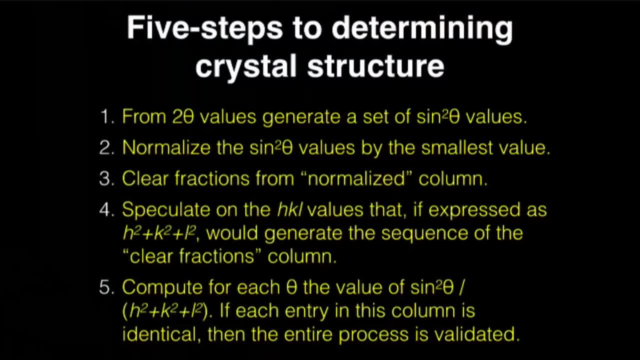 But we're getting real close. That's good. It leaves us with a sense of anticipation and excitement. So, OK, I got clear fractions. What values of hkl, if I have this h squared plus k squared plus l squared, would give me the sequence: 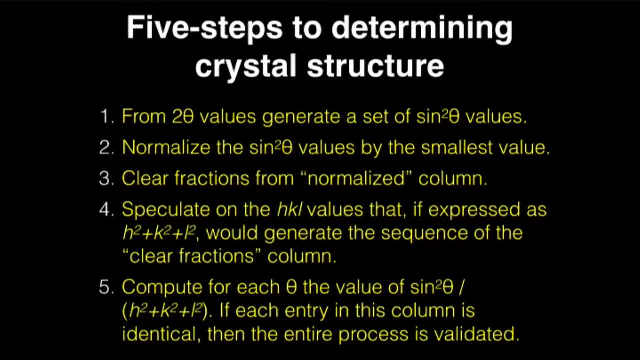 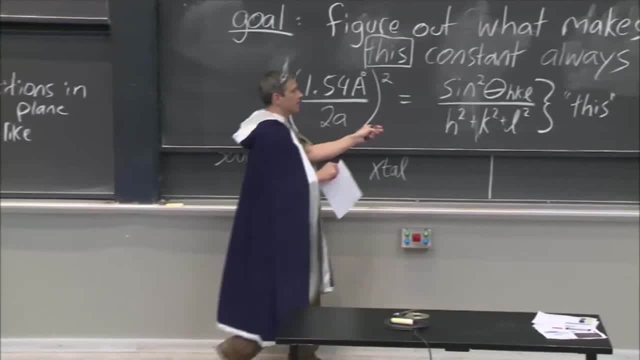 of clear fractions. What values of h squared? Now remember. you say: why am I doing this Again? go back to this. This is why I have a simple recipe for you to accomplish this goal. That's where we're going with this. 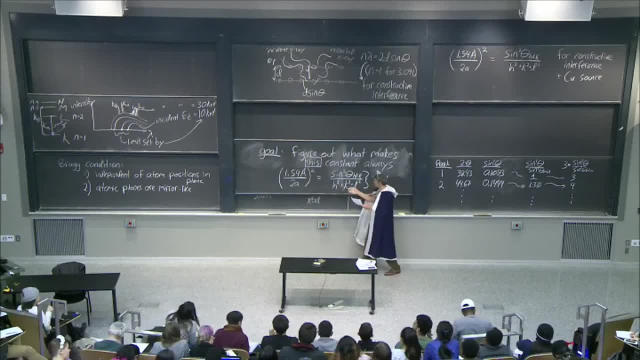 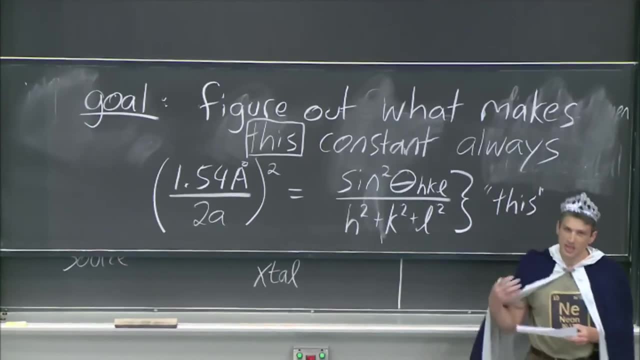 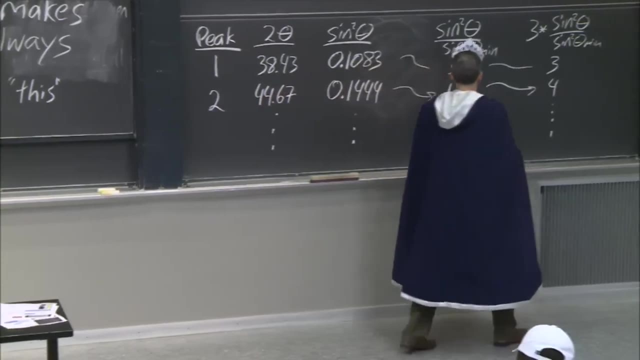 Right, OK, So I'm now going to see, with those clear fractions. now it's very easy to see what hkls would give me. h squared plus k squared plus l squared equals that clear fraction value, Right? So for example here: well, if this is h squared plus k squared, 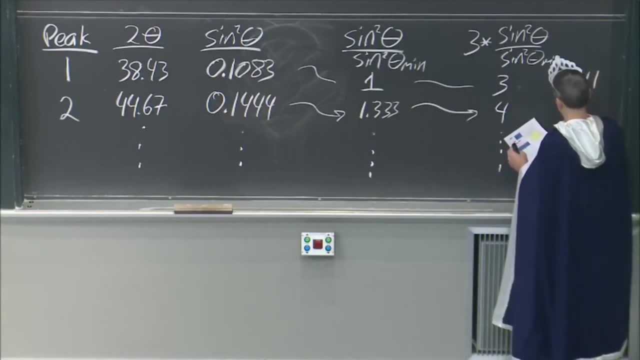 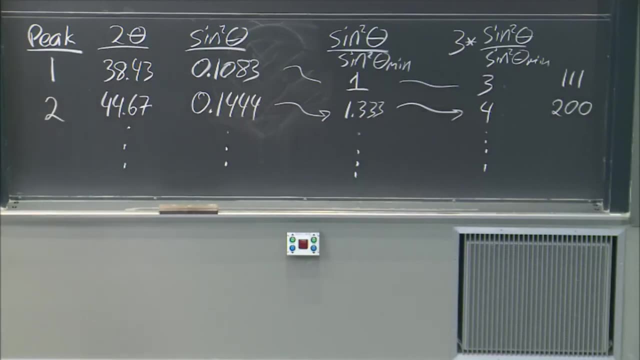 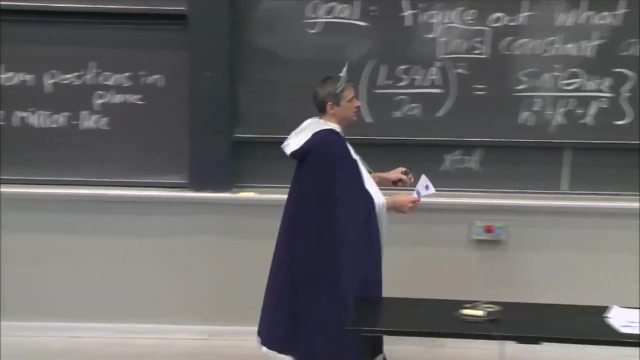 plus l squared, maybe this is 1, 1, 1.. And this might be 2, 0, 0. For example. So we're almost there. We're so close. What we're going to do is I'm going to start on Friday.